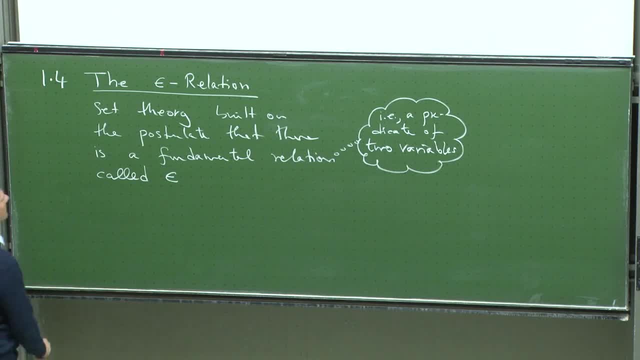 notions about it. It's simply a relation and it's called epsilon. There will be no definition of what epsilon is, and that's important. There will be no definition, in the strictest sense, of what epsilon is, apart from it being some predicate of two variables or, for that matter, or of what a set is. Now, this is weird. We're going to write down. 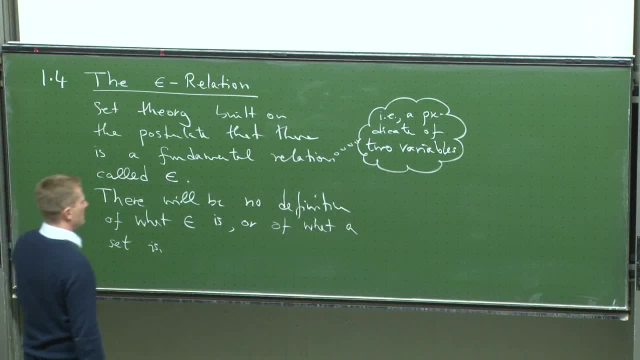 theory. but I tell you there will be no definition of what the elementary symbol, epsilon, the element symbol, actually is, or what a set is. Well, I use the definition in a strict sense, namely saying epsilon is defined like da-da-da-da or a set is da-da-da-da-da. We're not going to say this. 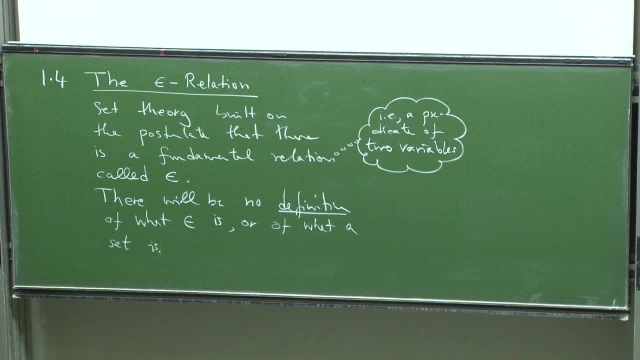 Instead, we're going to write down nine axioms. Instead nine axioms, We're going to write down nine axioms that use or that speak of epsilon and sets, And these eight axioms will teach us how to use epsilon and what constitutes a set. 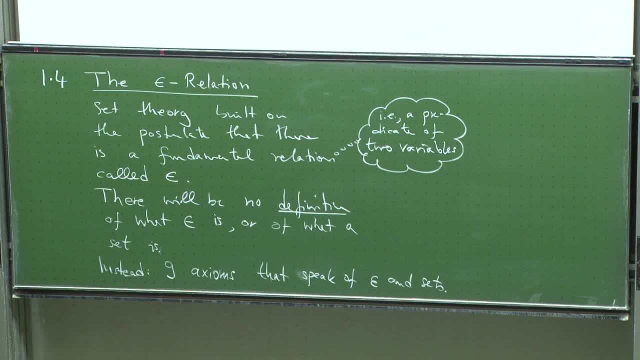 So it will only be the interplay between the epsilon and what we call sets which defines what a set is and which defines what the epsilon means. And, as I indicated last time, such an approach is necessary if we want to start writing down mathematics from scratch without any prior notions, without 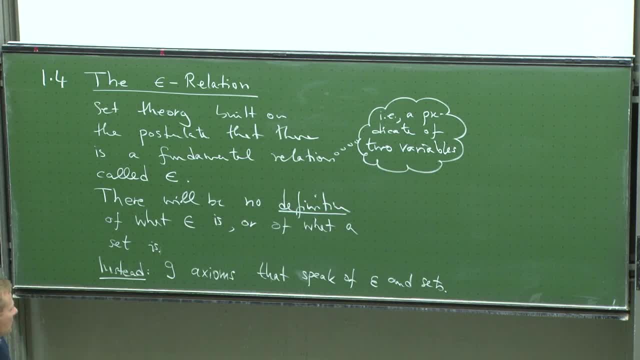 any prior terms in terms of which we could define the element, relation or a set. Now, which axioms are there? So overview over the axioms, So I memorize them as ee, perp, icf. So you've got to learn this like a poem. 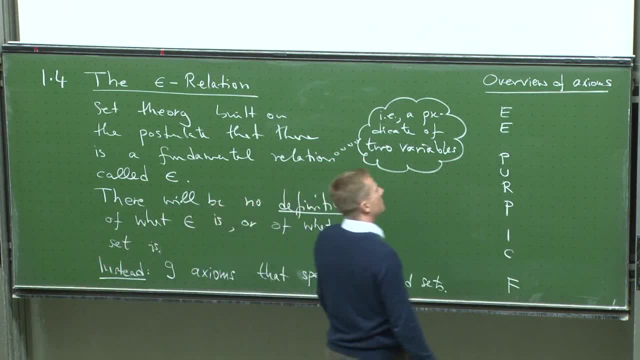 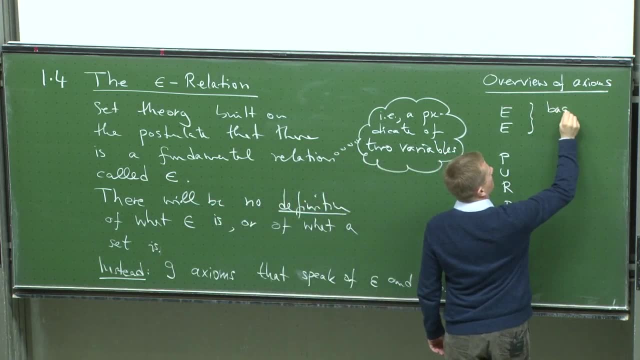 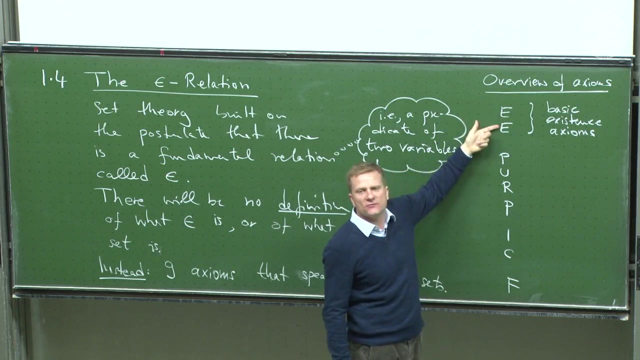 ee, perp, icf. Well, this ee, they're- let's call them- basic existence axioms. So that's their character And that has to do with the kind of a property of the element relation, And the e stands for existence of an empty set. 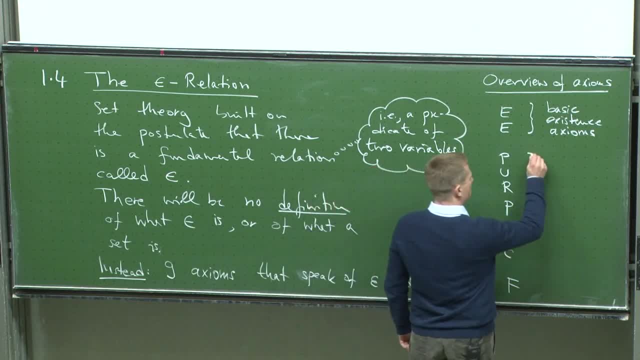 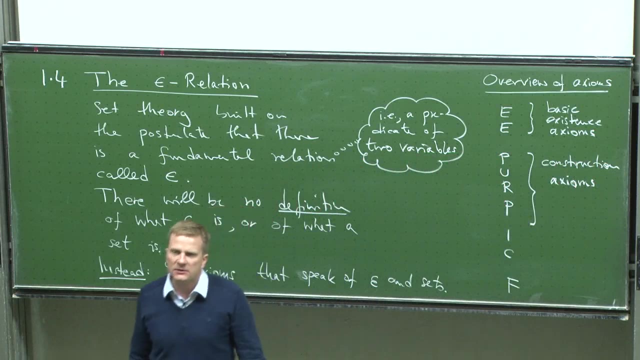 Of course we will specify this, The perp. they are heavily used construction axioms, Construction axioms, construction axioms which instruct us how to build new sets once we have some given sets. That's, of course, a recurring theme that if you've got a structure, you want to know. 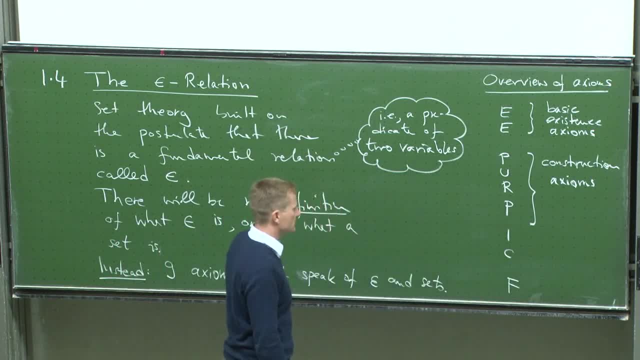 how to build from elementary building blocks or, given structures of this type, new structures. P is the pair set. axiom U is the union set axiom R is the replacement axiom, powerful thing, P is the power set axiom. Now I see these are further existence axioms. 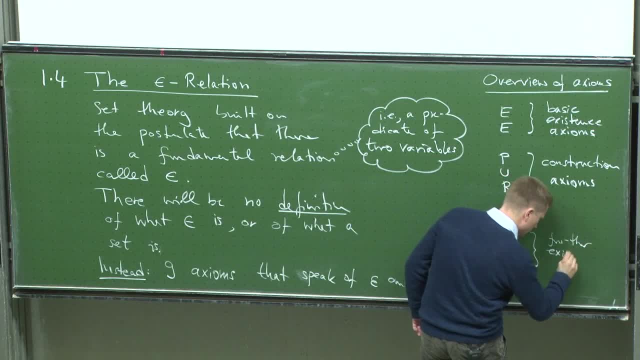 Further existence axioms, but they could also be classified as construction axioms That are a little more advanced and actually are rather newer than the other axioms. And the F is the so-called axiom of foundation, And the character of this is more of a non-existence axiom that says: 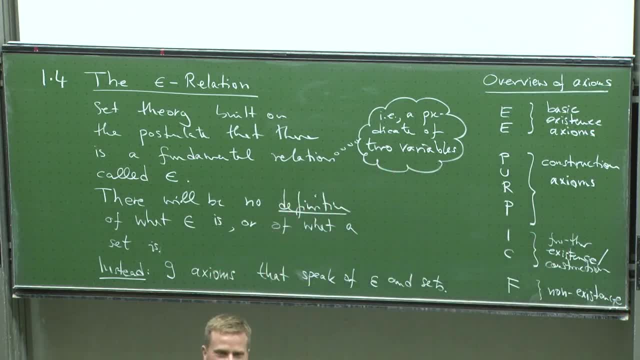 don't use sets of the following kind, So that excludes something. That's the overview of axioms, And now we're discussing them in turn And I use I will discuss them in this order, Partly because some of the later axioms rely on the earlier axioms. 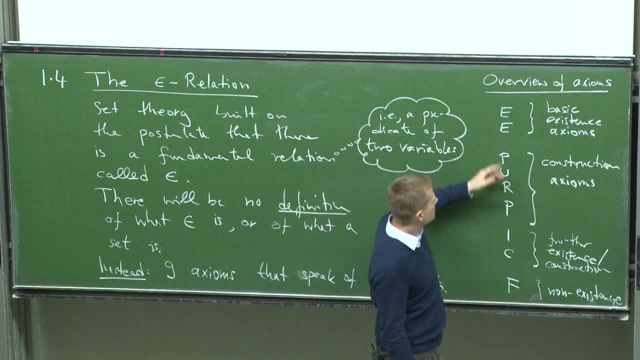 But then also I want to give some immediate application of each axiom So that we get a feeling for them, And sometimes I push them down the list in this order In order to be able to use some previous application in the more advanced application. 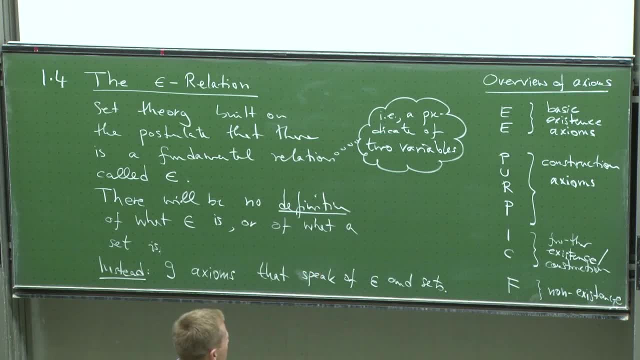 So that's why we have this order. But EEPERPICF, you agree, is a wonderful mnemonic, So never forget nine of them. These are the initial letters, if you will. So before we go there, let's actually introduce some new relations. 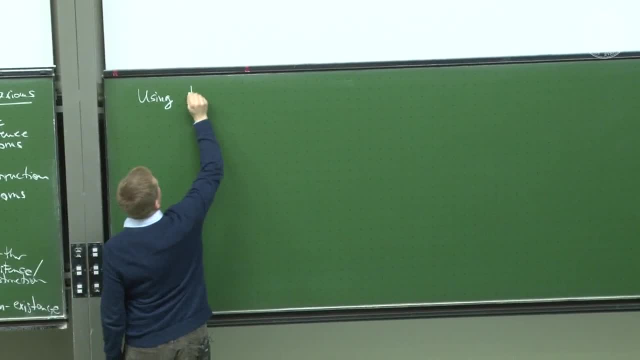 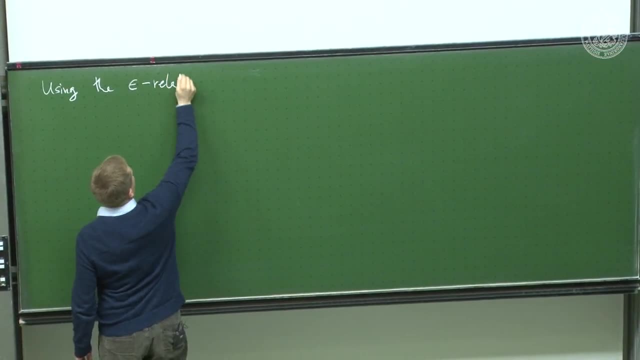 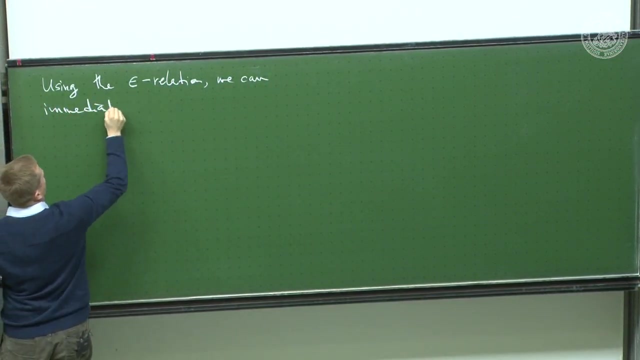 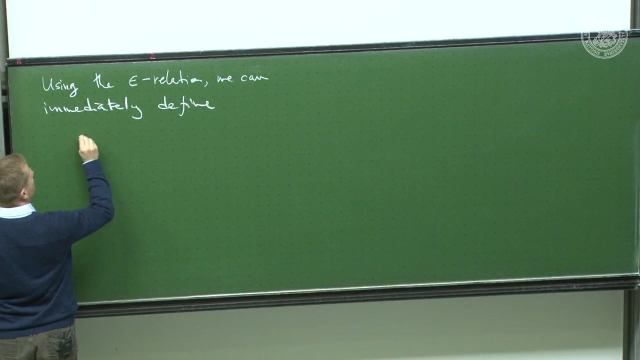 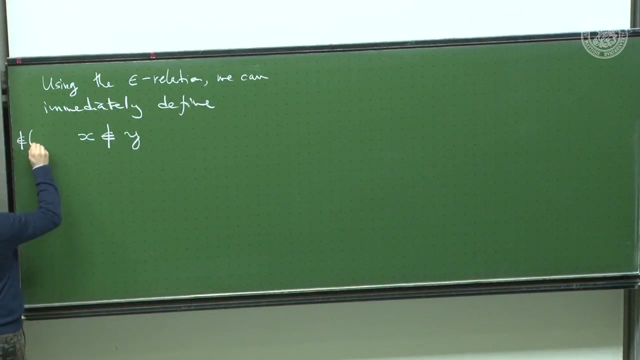 Using the element relation, I sometimes call it the element relation. The element relation, we can immediately define well further relations. One fashionable one is x, not an element y. So you see, a relation in principle is a symbol that eats two variables. 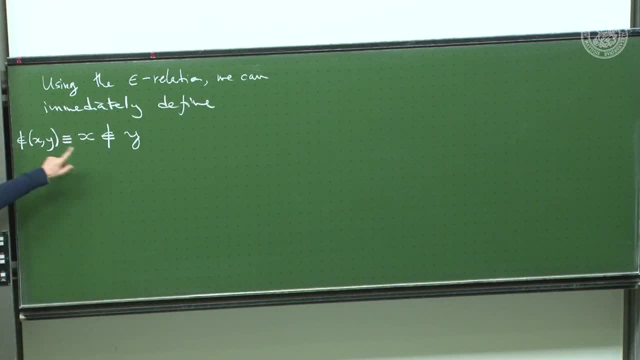 But it is tradition to then put the symbol between the two variables. So, if you wish, the right hand side is defined in terms of the left hand side, Because you save two brackets and a comma And it's the more traditional notation. 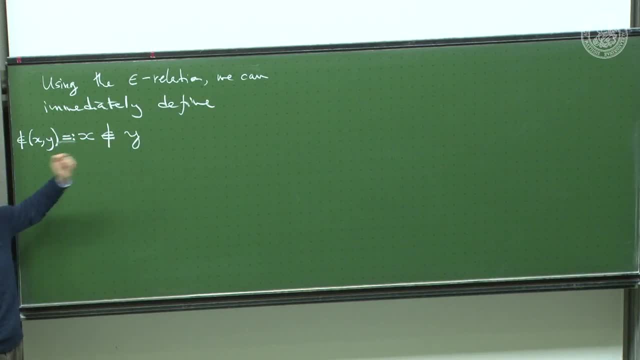 Just for you to realize, this really is a relation between two objects. Once we have so we define this, This is defined to be equivalent, Not x and y, And we define a subset relation Written like this, Which is defined to be the case: 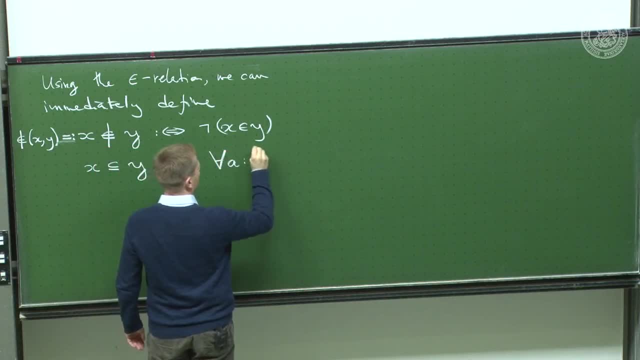 if for all a, it is true that a in x implies a in y And finally we define x equal y. So you see the equality sign which we would probably normally take without further questioning what it means. 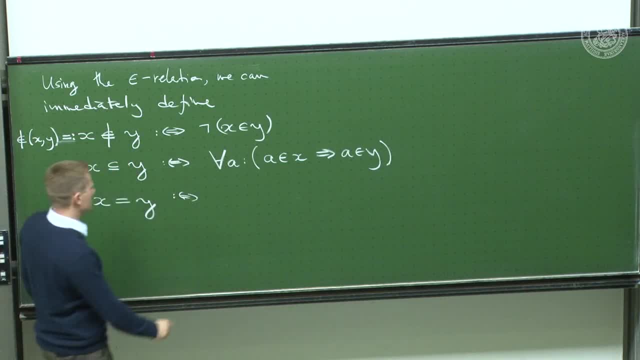 is actually defined in terms of the epsilon relation. x equals y means that x is a subset of y And y is a subset of x, And for that subset relation we use that here. So that's the definition of the equal sign. 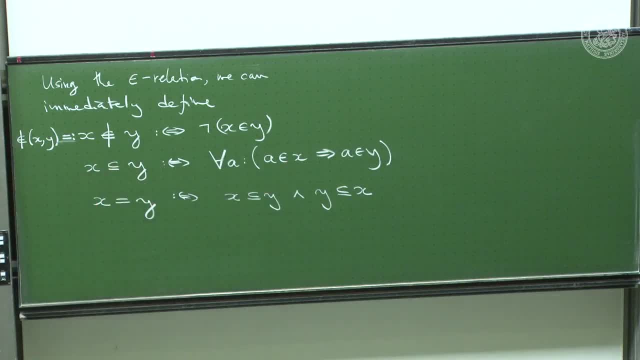 Which, therefore, ultimately, is defined in terms of the epsilon relation. Now, having said that, um, we come to the axioms, the Sermelo, Frenkel, Frenkel, axioms of set theory. So these are the nine axioms. 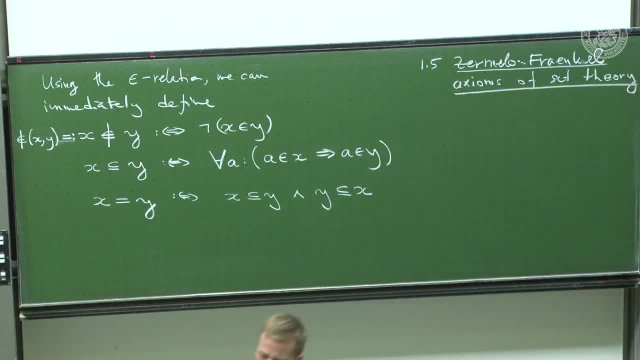 I talked about, And the first axiom actually declares that the relation between epsilons and sets. So let's call this the axiom on the epsilon relation. What it's character is. we know it's a relation. 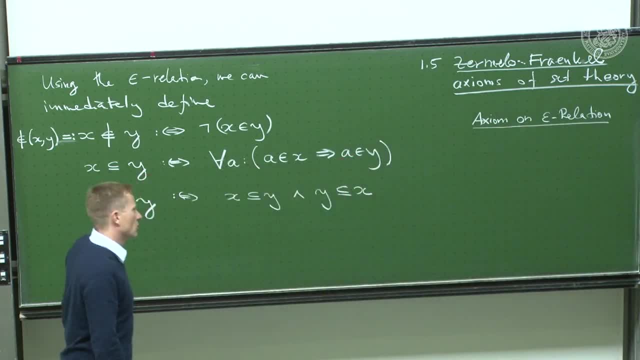 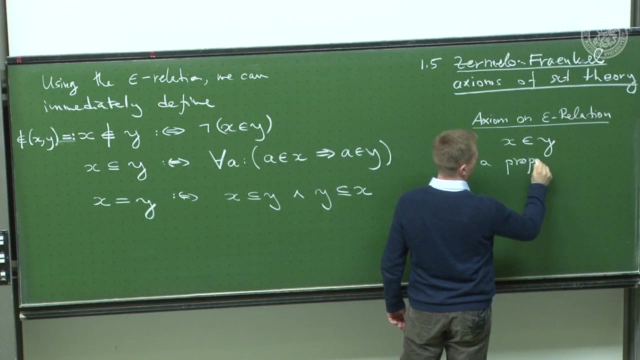 but what it's relation uh to sets Um, Whenever, no, um x element y is a proposition, that means it's either true or false. is a proposition if, and only if. 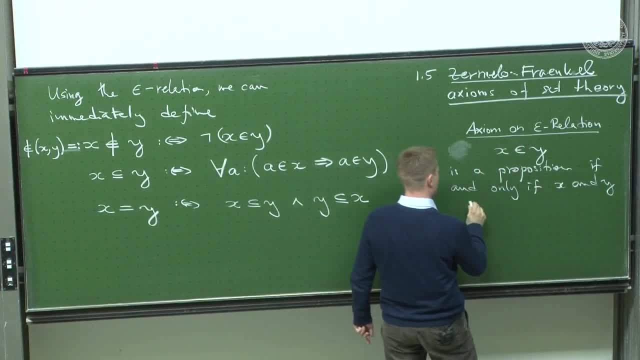 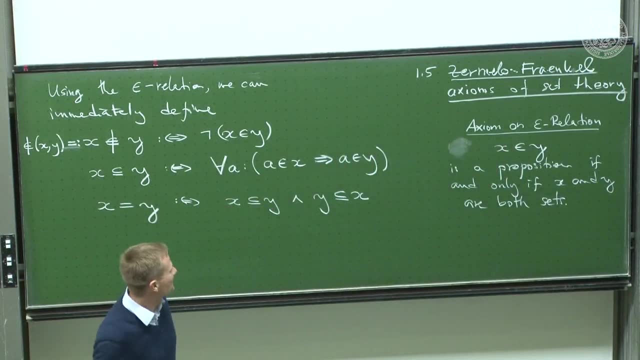 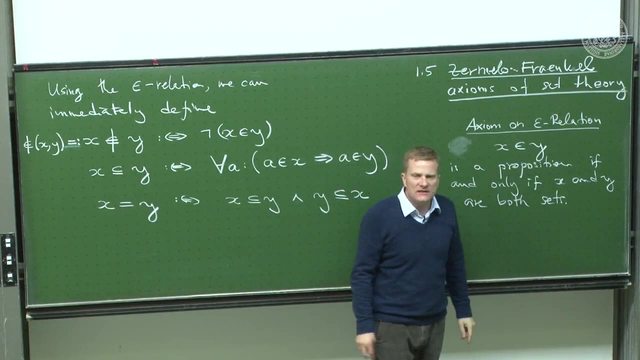 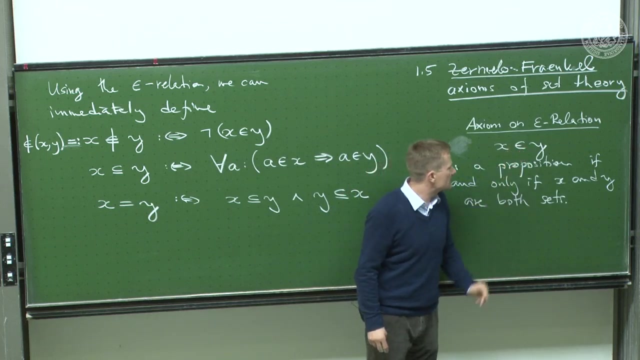 x and y are both sets. Aha, So you remember that. in first order, predicate logic. I explained last time we leave it entirely open what the nature of the variables that enter a predicate, in this case a predicate of two variables. 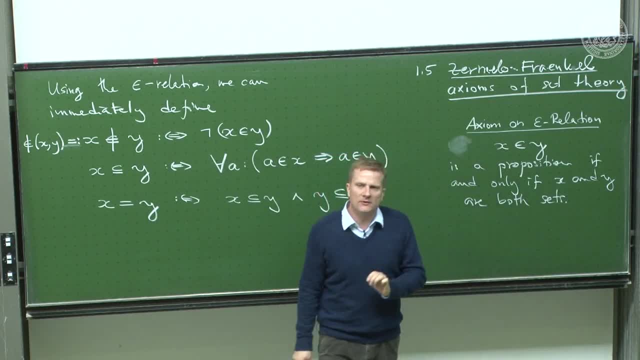 what the nature of these variables is. But this first axiom clarifies x element y. that's how we read it: x, epsilon y is a proposition, and therefore epsilon a relation, only if it acts on. 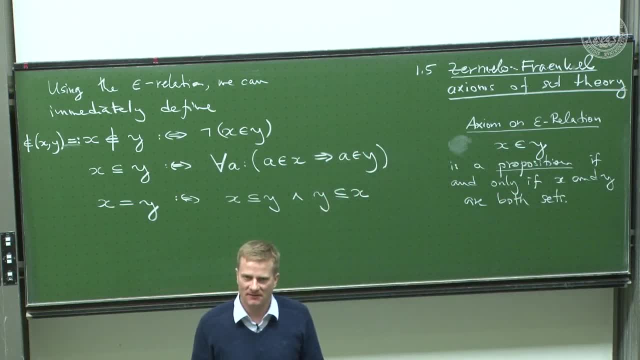 what we are going to to call sets. It's the first thing we know about sets And that seems so trivial that for a long time people thought this is not much of a historically. 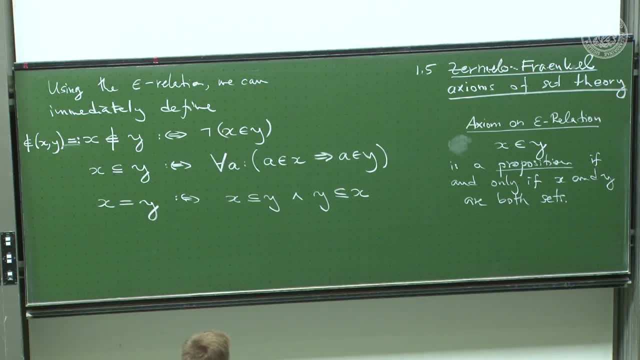 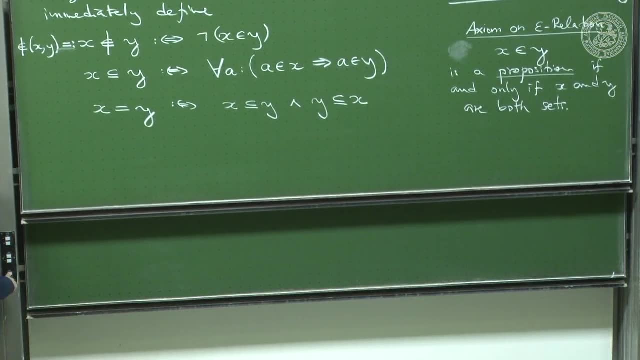 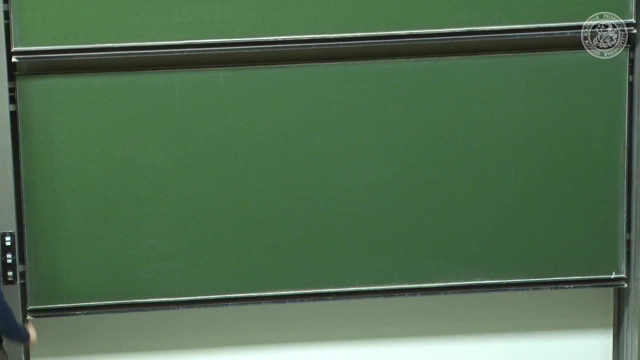 this is not much of a condition, But in fact it is. So let's immediately give a counterexample. what is not a set, And this is a very famous counterexample. Counterexample, Assume there. 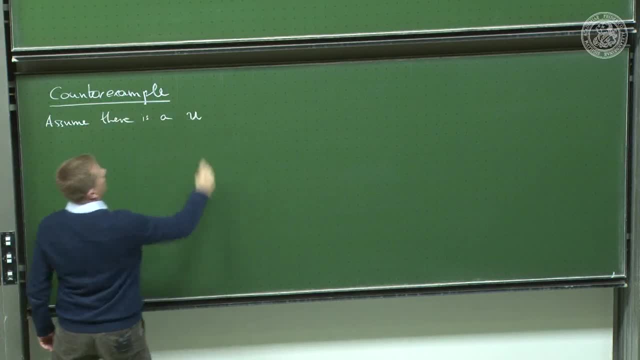 is a, an object, U, there is a U or there is some U that contains all sets, x, all sets- forget about the x- all sets that do not contain, as an element, themselves. 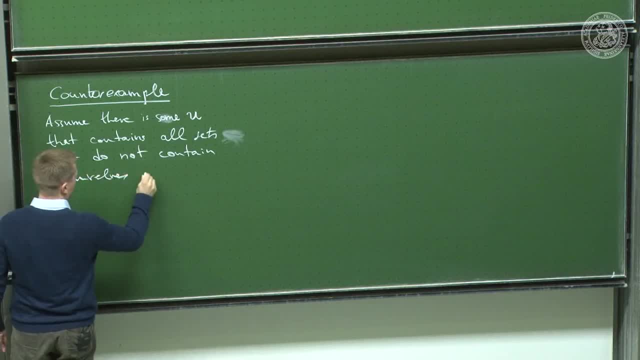 what do I mean by this? in order to be precise- and we should be precise in order to fix our language before we get more nonchalant with it- to be precise, we assume there exists a U such that for all Z in U, for all the elements of U, 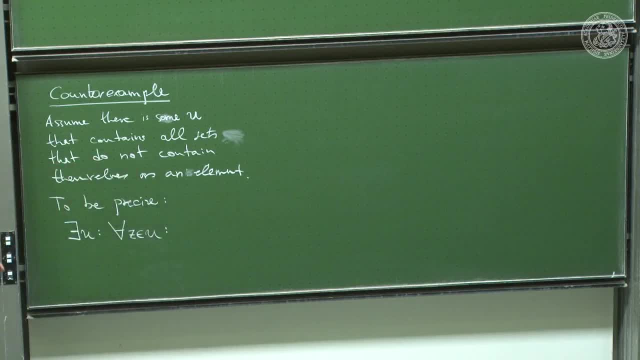 it is true that- sorry, I didn't explain so that for all Z we have that Z in U if and only if Z. I called it Z, not in Z. so so is this right? we have all those Z in U that do not contain themselves. yes, so we assume Z is a set. 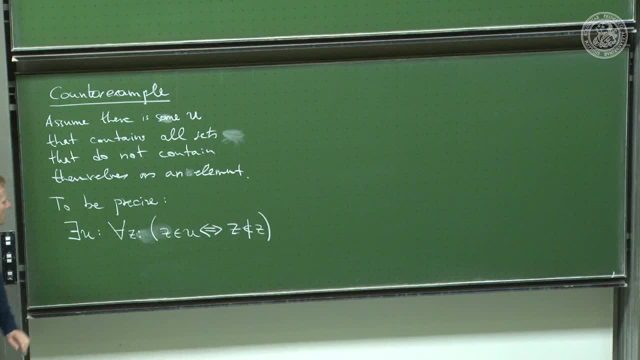 and we look, we assume there is such a U. now question: is U a set? can this set of all sets that don't contain themselves be a set? maybe? maybe you're worried about this because you have been trained to distinguish very carefully between a set and the elements of a set. 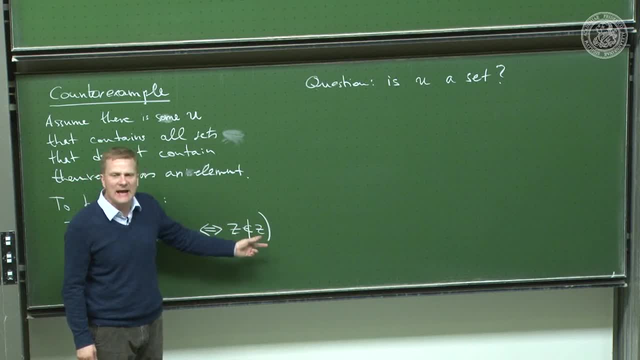 and it may disturb you to think of a set being an element of itself or not being an element of itself, but remember well and finally, this non-existence axiom will say: don't even look at such stuff, ok, but at the moment, and it's very instructive, 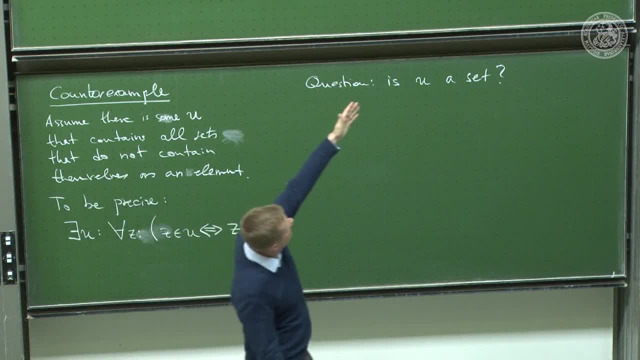 instructive to consider this. we just said epsilon is a relation and whenever X and Y are sets, X element Y is a proposition. yeah well, if Z is a set, then Z element Z or Z not element Z. Z is a proposition, right? so at this point it's perfectly fine to do this. 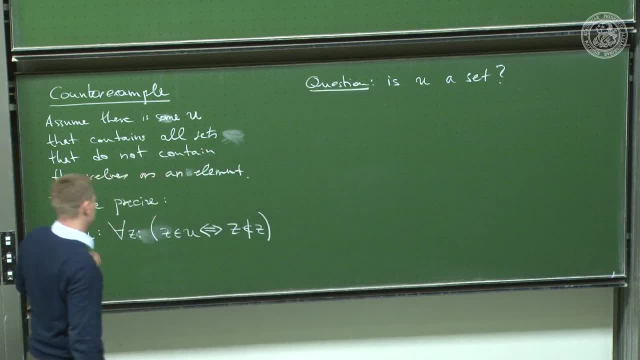 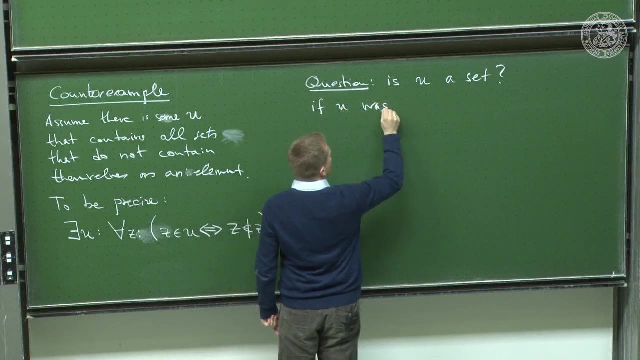 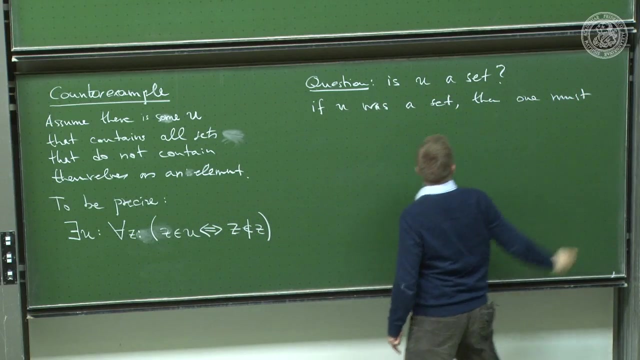 but the question is: this collection of all the sets that don't contain themselves, is this a set? again? and the answer is no. but how can we see this? well, by looking at this axiom, because if U was a set, then one must be able to decide whether 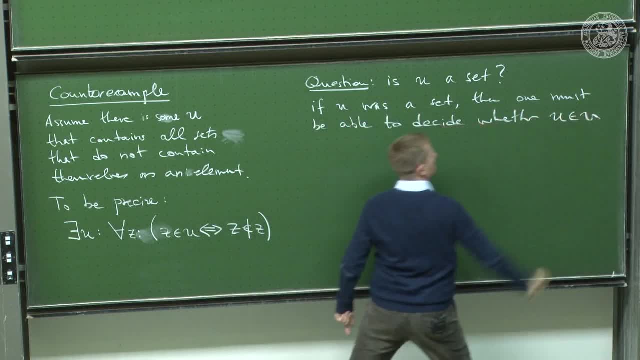 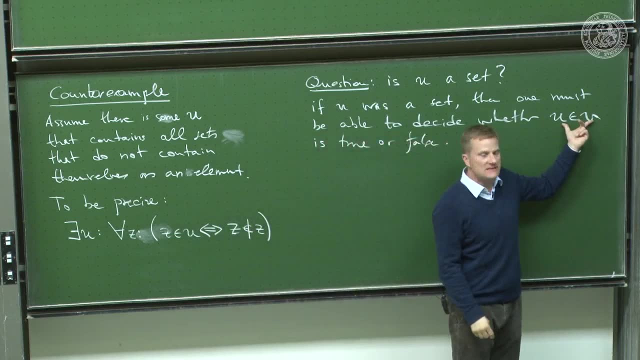 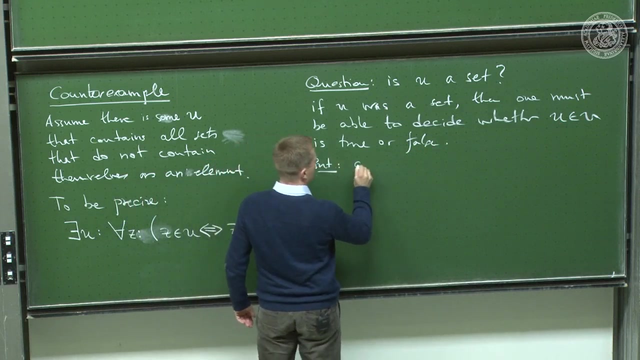 U in U is true or false, why? well, if U is a set, then U in U must be a proposition, and a proposition is something that's either true or false. very simple. well, that's exactly the problem here. but assume that U in U is true. it would be one possibility. 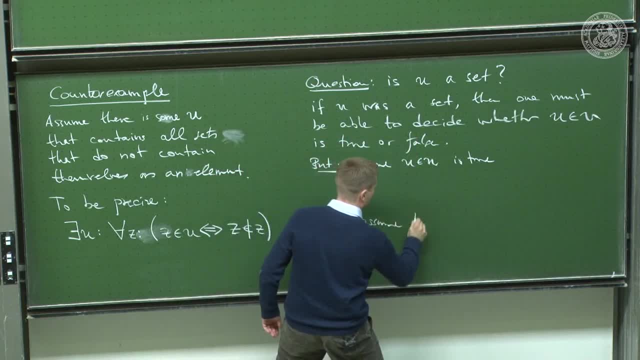 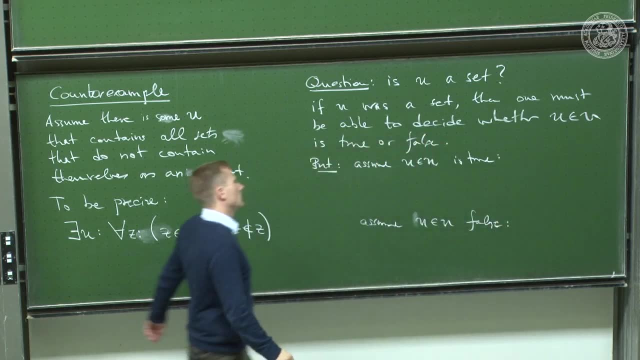 and the other one is: assume that U in U is false. so one of the two must be the case, because U is defined well. if you assume U in U is true, then it must be true, then U is an element of itself, so it's some particular Z. 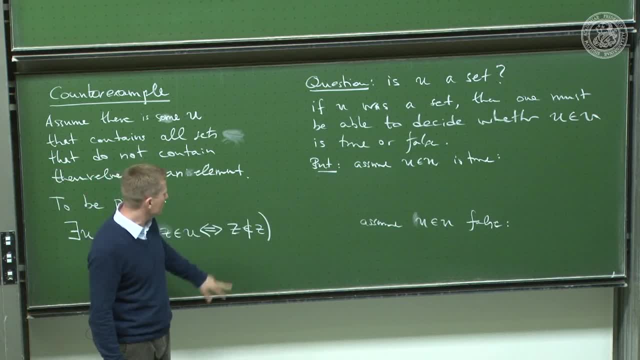 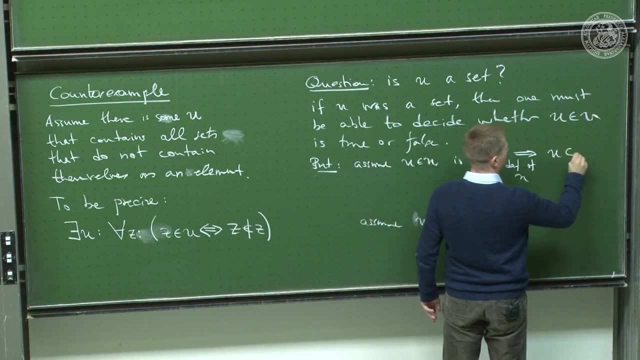 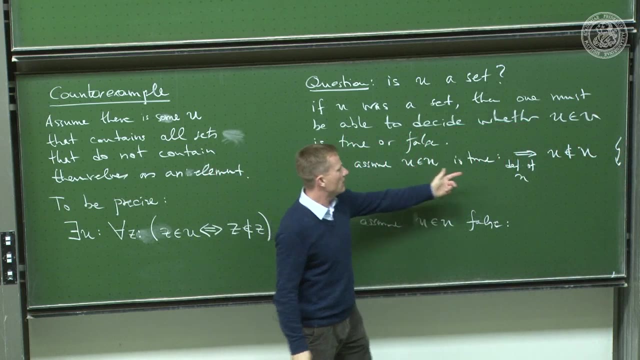 but then it implies that Z not element Z, so that U not element U. it immediately follows from the definition of U that U is not in U. that's a contradiction. so we assume U is in U. it implies U is not in U. what does that mean? 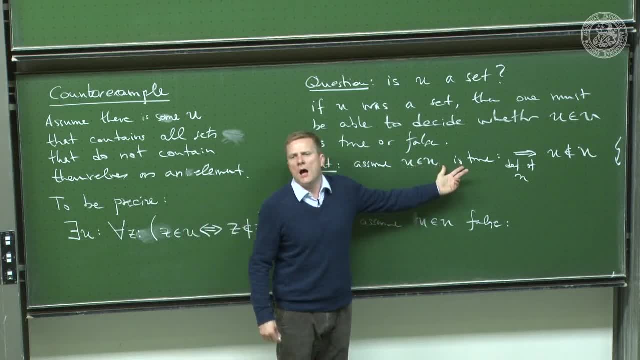 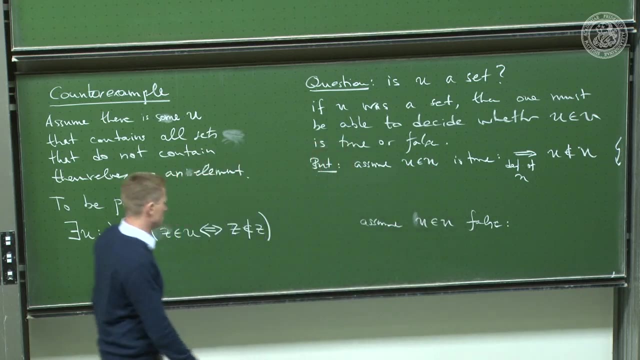 well, it means that this assumption cannot be true. not a problem. yet if that's not true and it's a proposition, then it's probably false. it must be false if U in U is a proposition, so let's investigate that case. assume U in U is false. 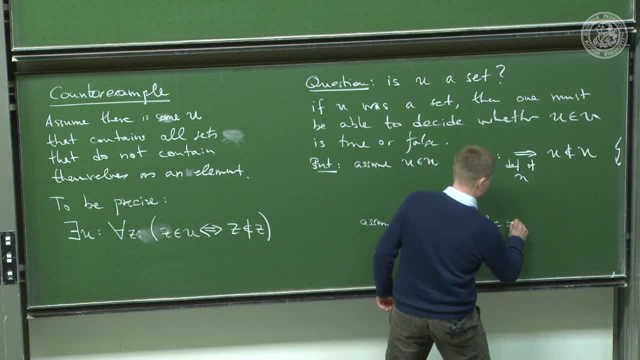 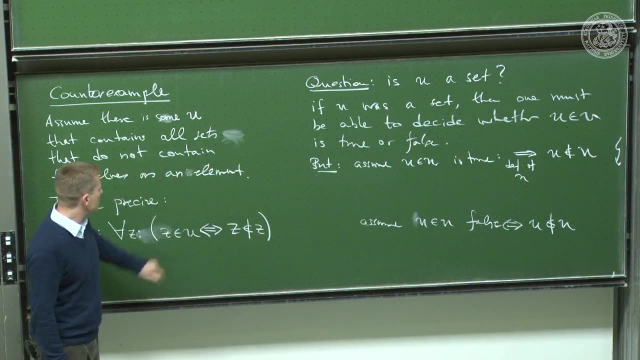 if U in U is false, that is equivalent to saying that U is not in U. no doubt that's the definition of not being an element of something. but if U is not in U, then it must be in U, because U contains all those sets that don't contain themselves. 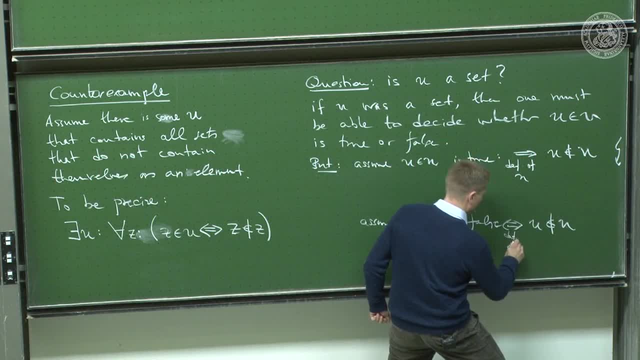 so that's the definition of, not an element of. but then it follows by the definition of U that U is an element of something else. so that's the definition of, not an element of U. U that means the assumption that it's false also leads to a contradiction. 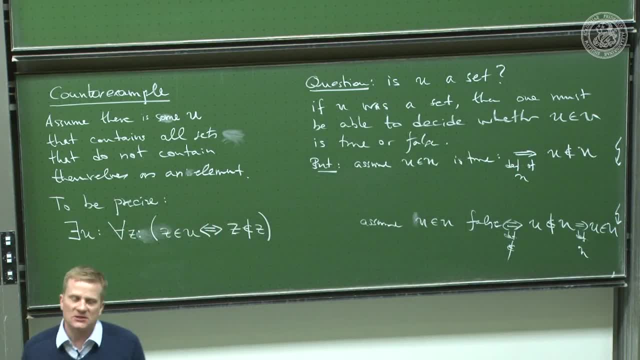 there's only one conclusion. conclusion U is not a set. this is the right way to go into the so as having taken the idea of values over the paradigm is present- has been taken into fight. into fight thick volumes. and they thought they built the work of their life. 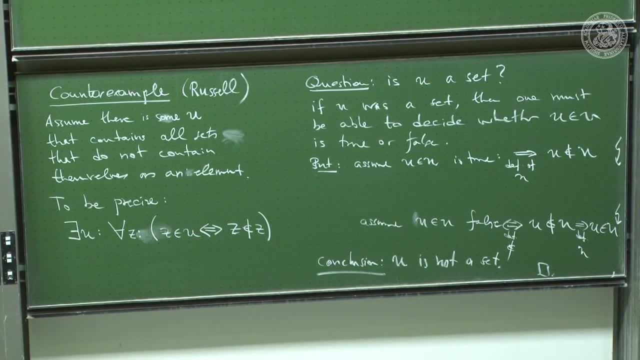 and they built this language, this foundation for mathematics. but it was not this set of axioms. it was what today we polemically call naive set theory and which is taught usually at school and in undergraduate courses. we use naive set theory And in naive set theory 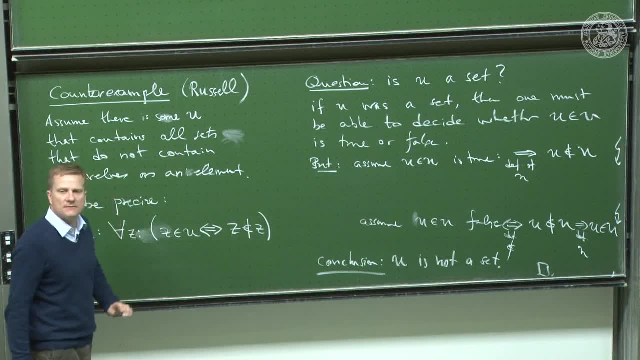 you can easily make constructions like this. you would in school. you would maybe write: u is defined as the set with all those elements z that have the property z is not an element of z. This is just the standard notation for this. You condition elements to be: 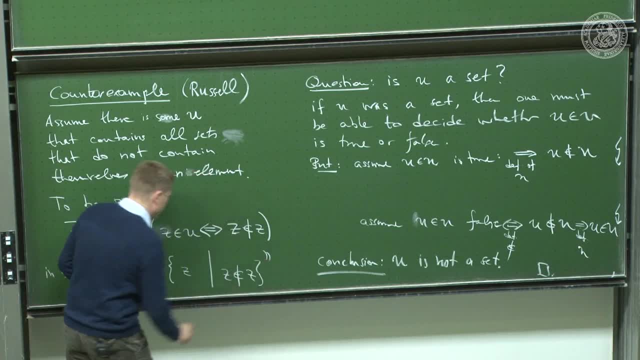 in a set, I mean, mind you, we haven't introduced any such notation yet, but that's the idea of what is written here, and so you easily construct things, objects that are not sets- And Russell, after they wrote these two books, and he discovered this: 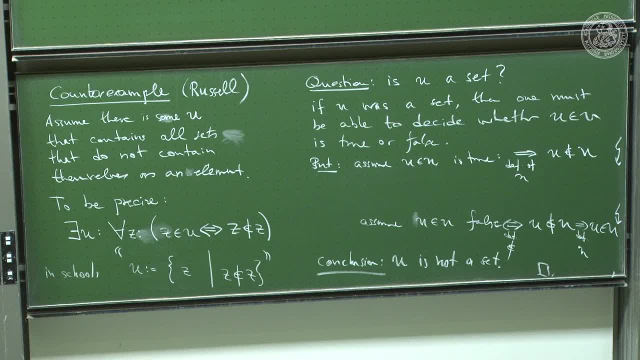 contradiction, this antinomy. he actually couldn't sleep well and he had nightmares about the big Cambridge library people taking the two books and he had nightmares about the big Cambridge library people taking the two books and he had nightmares about the big Cambridge library volume and throwing them out the window and stuff and so on. 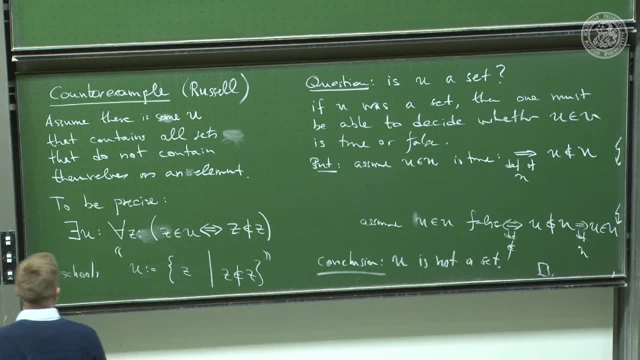 So it's a drama, But finally the resolution of this drama and other dramas, other contradictions, inconsistencies of naive set theory were finally resolved in a big struggle by a number of people and today we honour Sermolo and Frankl in particular for coming up. 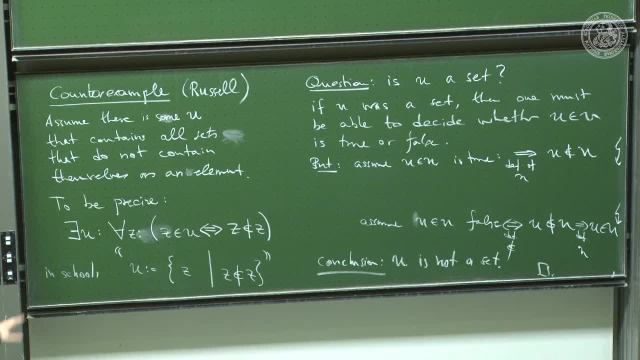 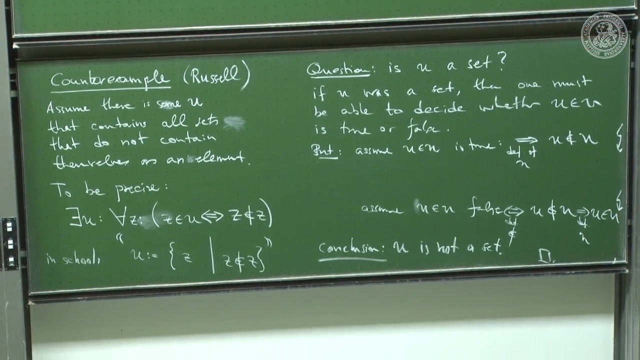 with a set of axioms that deal with this in a better way. so the first axiom: fine, but you need 8 others in order to not run into difficulties. but the first axiom already tells you this would be a problem. any questions? so we completed E, the first E. 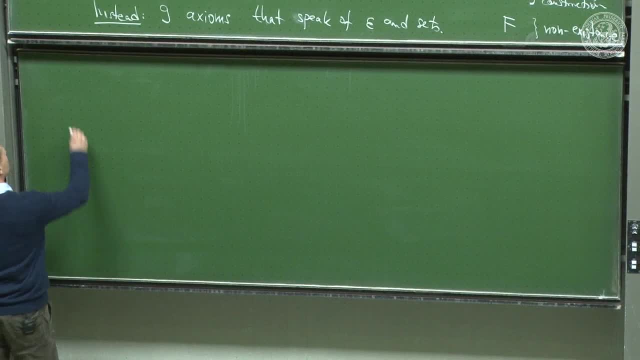 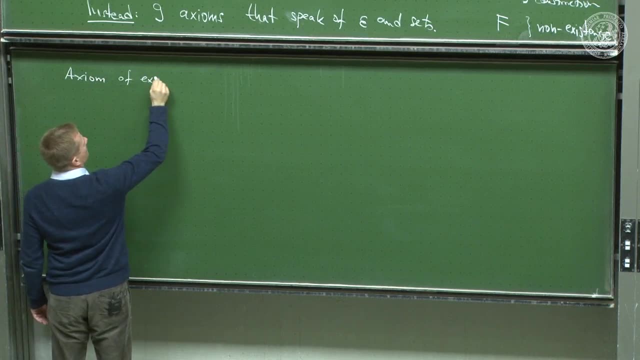 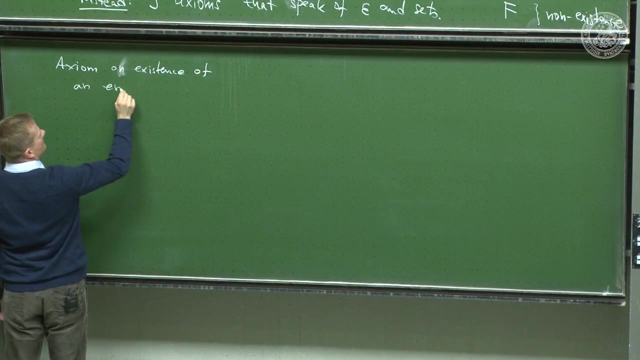 now we go for the second E. the next axiom is the axiom of the existence, or on the existence of the axiom, of the axiom of an empty set, and that's an easy one, very important: there exists a set that contains no elements. what does that mean? 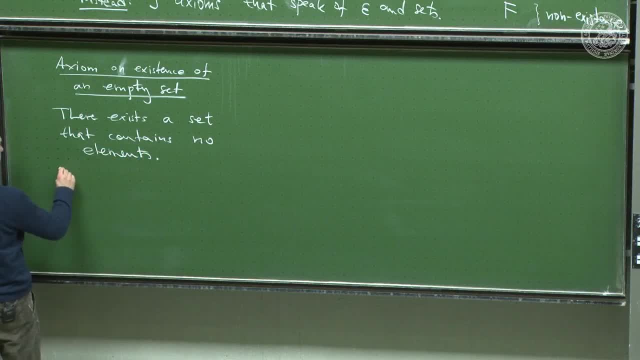 well, we agreed on having a precise language. that means there exists a set- let's call it x, such that for all y, it is true that y is not an element of x. this is the precise formulation of the statement: there exists a set that contains no elements. 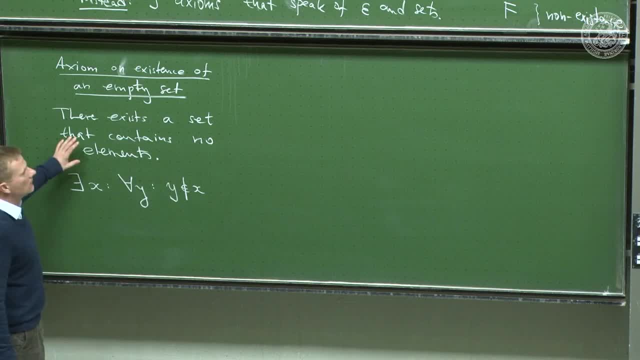 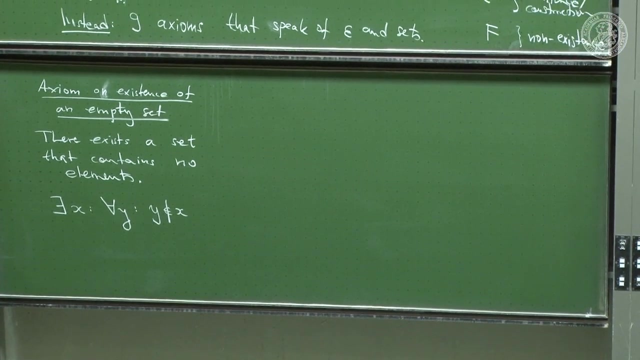 I will carry on for a while to formulate the axioms in this fashion, in this formal language, so that we see how that works. so in principle, up here we could have, maybe we should also write down the formal version of this axiom. so let me bring this down again. 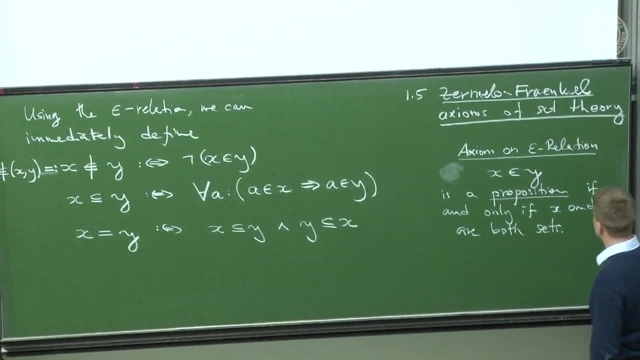 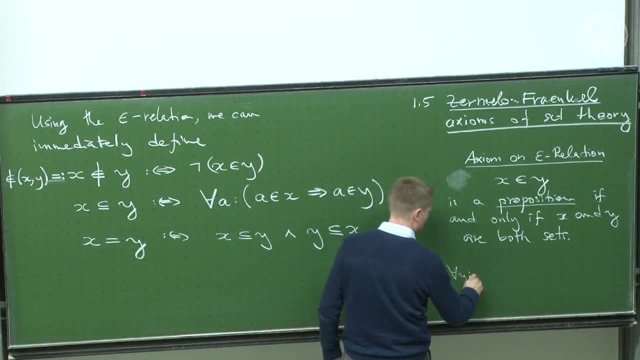 so the formal version of this axiom is the formal version of this axiom, so let me bring this down again. so the formal version would be: for all x and for all y. x element y is either true. either. or we define this exclusive, or it's either true. 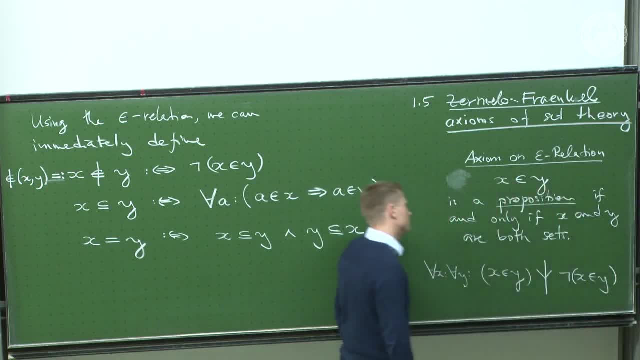 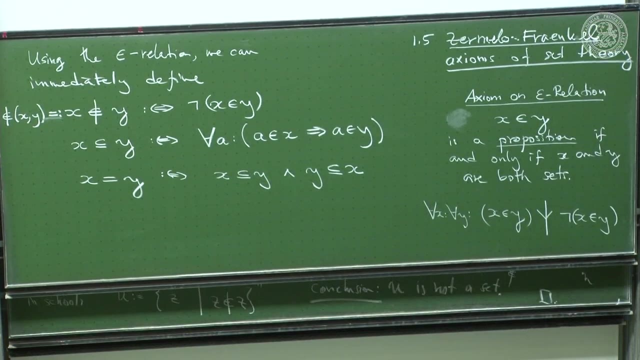 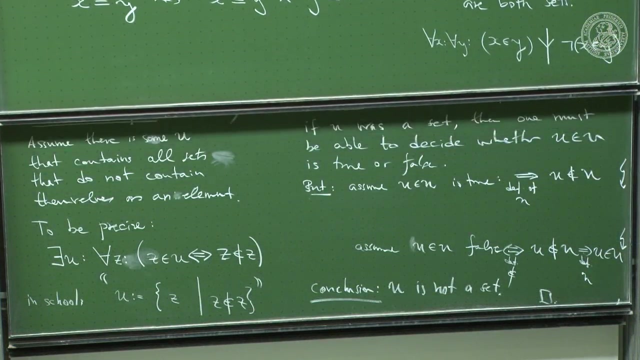 or it is false, if you wish. this is the statement that this is a proposition. it's descriptive: terzium non datur. there is no other possibility. it's either true or false. well, this is a little bit unnecessary. we know what it means to be a proposition. 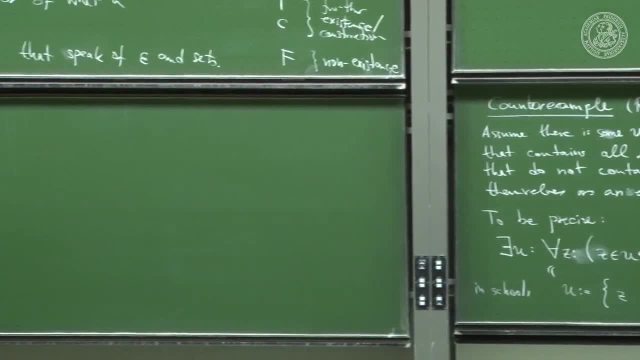 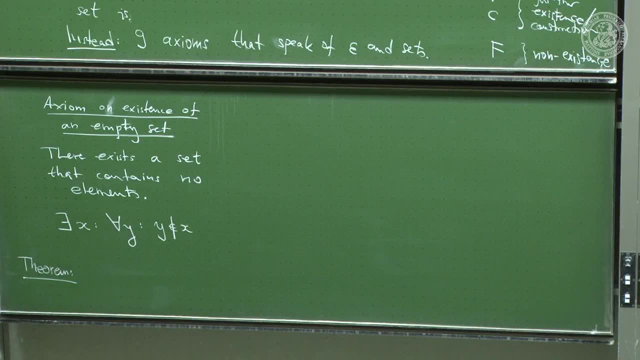 now, this is the existence of an empty set. now we have an immediate theorem which is very simple: there is only one empty set. there is only one empty set and because there is only one, we can give it a name. call it empty set, zero with a slash. 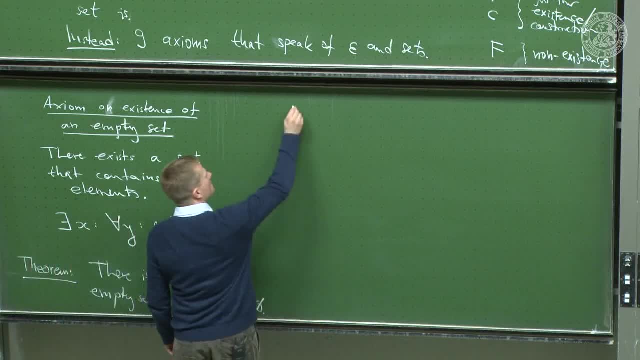 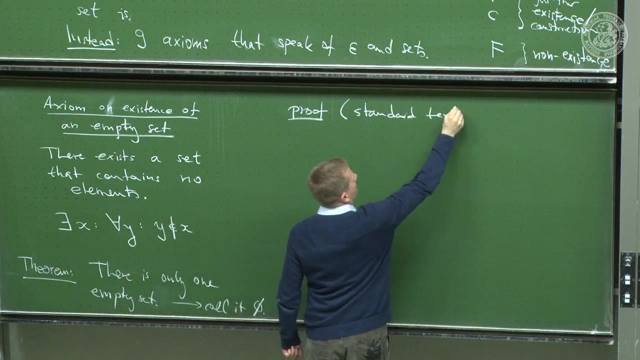 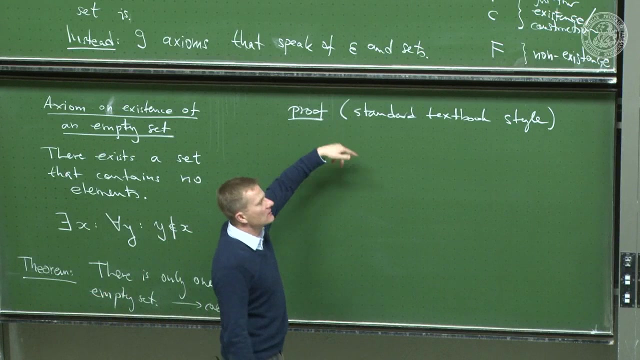 now, what's the proof of that statement? and I'll give two proofs. same idea of both proofs, but the first proof is the standard textbook style proof, which in this case, it doesn't mean that the textbooks omit something or not precise enough. well, it actually means we use our standard way. 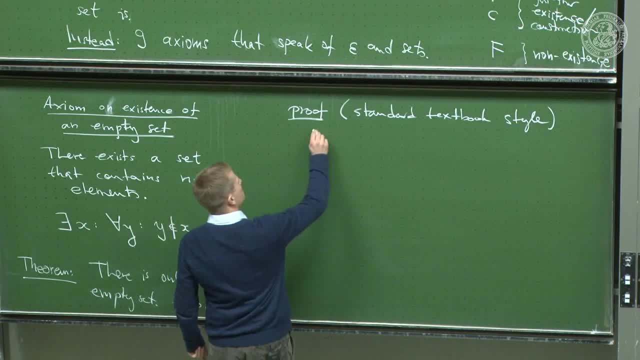 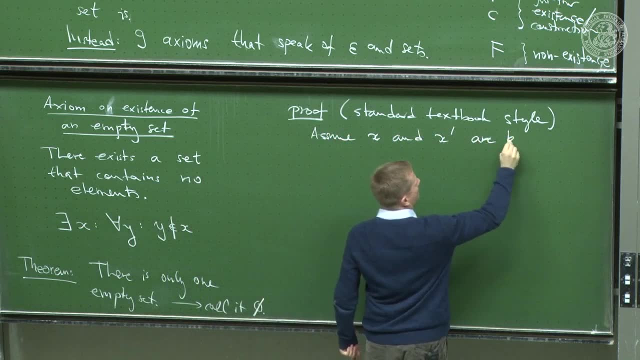 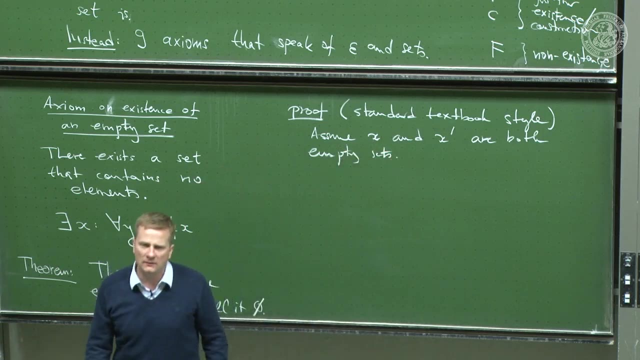 of thinking of the textbook, of the textbook of thinking about these things, and it goes as follows: assume x and x prime are both empty sets. how do we prove that there is only one? well, we have to show if this assumption is that this assumption leads to the fact that 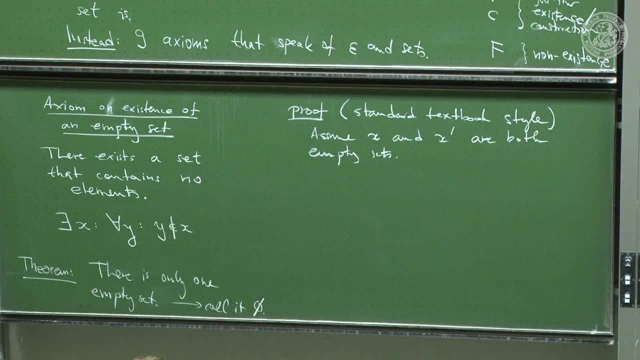 x equals x prime. so if two empty sets are always equal, then there is only one: are both empty sets? well, if that is true, then I can write down something like: y is an element of x. and what do we know about this proposition if x is an empty set? 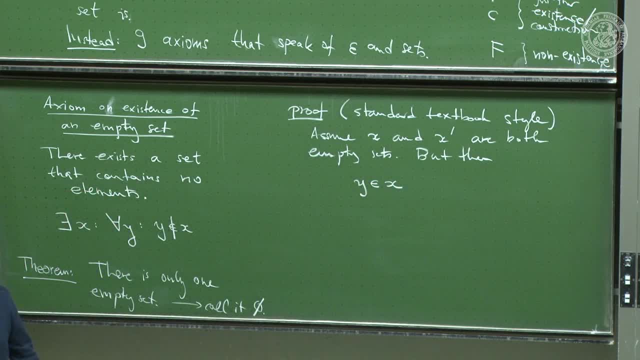 and I write down y and x. it's false for whatever y is right, because the empty set has no elements. but if this is false, then I can write an implication arrow, and here I have an implication arrow, and here I can write whatever I like and the whole statement. 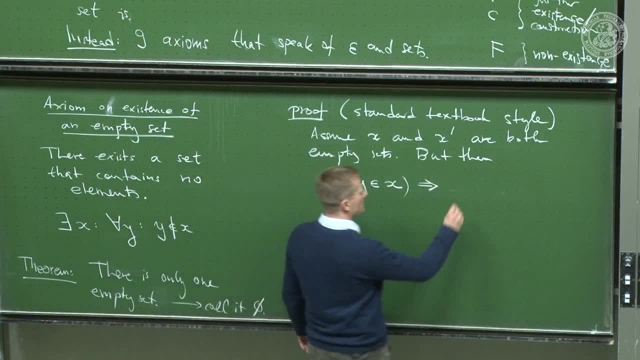 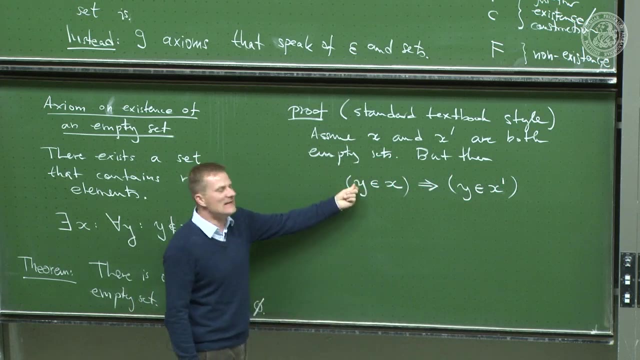 will be true, correct. and I happen to like to write x element, y element, x prime. well, if I can write whatever I like, I mean any proposition I like. ok, I do this. so the whole thing is true, independent of what y is. is that correct? but if that proposition, 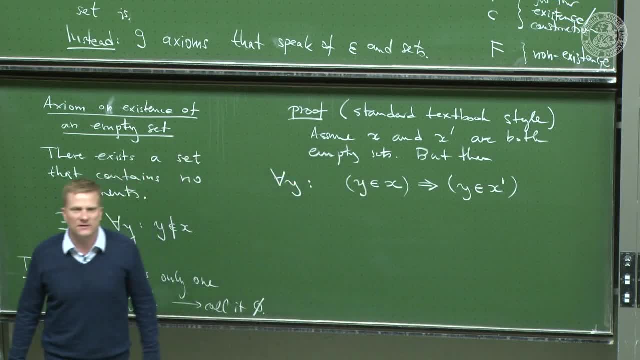 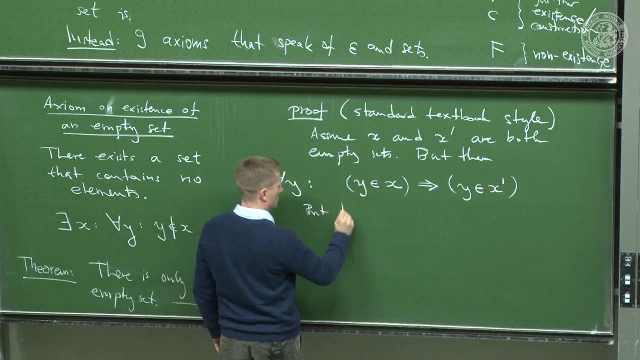 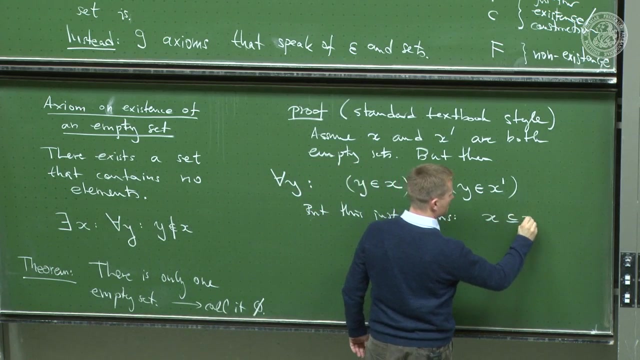 is true independent of what y is, we learned it's the definition of the all quantor. to then have this whole thing being true if the proposition is true independent of the y, aha, yeah, but this just means by definition that x is a subset of x prime. 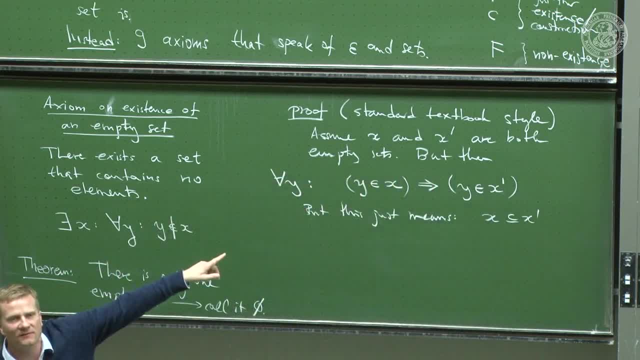 that was our definition of what a subset is. it's still up there. yeah, conversely, same argument. I can write down y an element of x prime, and this is always false. why? well, because x prime is an empty set for an empty set: y and x prime. 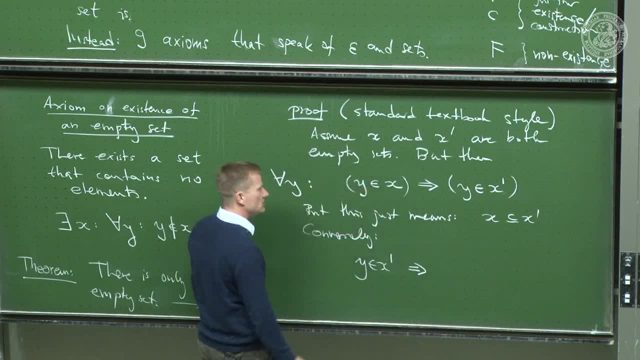 is always false. this is always false. I can write an implication arrow and write down another proposition of my choosing. I happen to like y element x, because this whole implication, this whole proposition is true, independent of y. I know that the all quantification of this is true. 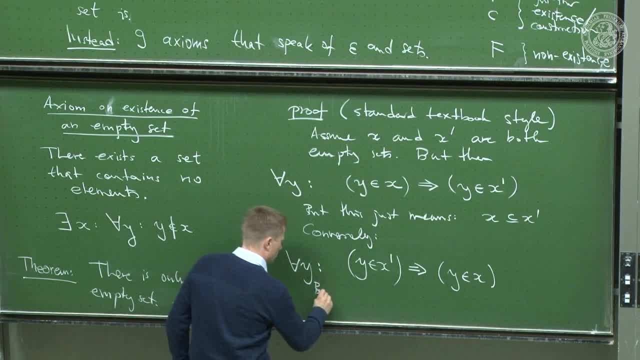 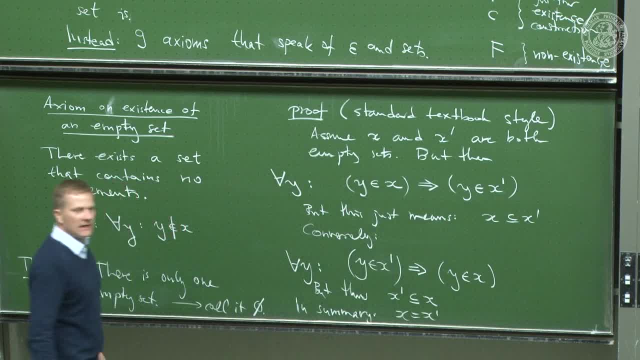 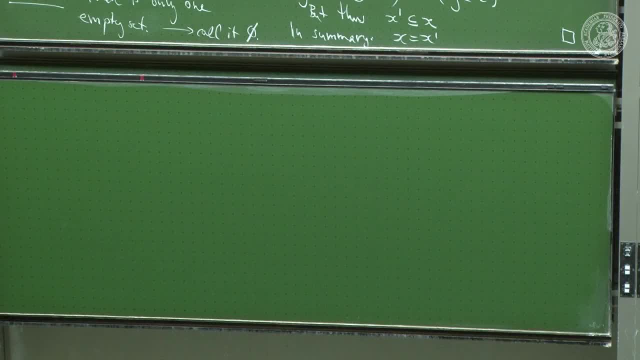 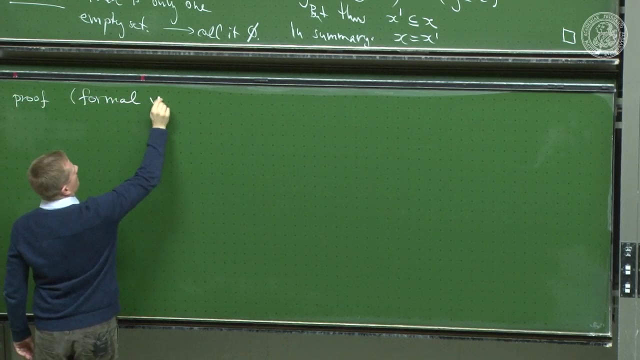 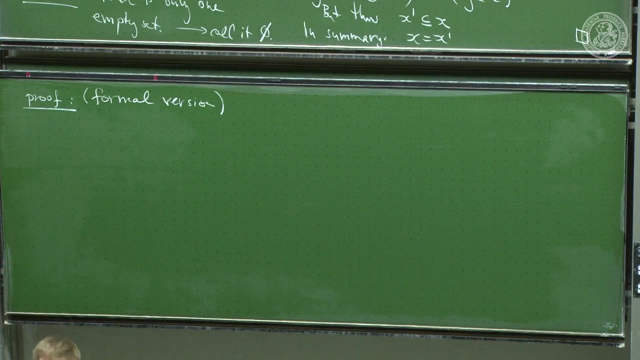 a very elementary proof. didn't we define what a proof is? does this have the form of what we define, what a proof is? no, it doesn't. so we will give a precise proof, a precise proof, proof, a formal version, and we will only do this once. no, no, no, no. 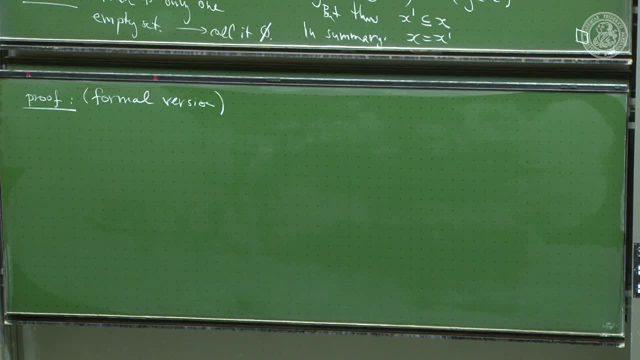 there is an element relation and what a subset is. unfortunately I erased it. what a subset is is defined in terms of that, but it's not the same thing. say again what implies. what does x being a subset of y imply that x is an element? 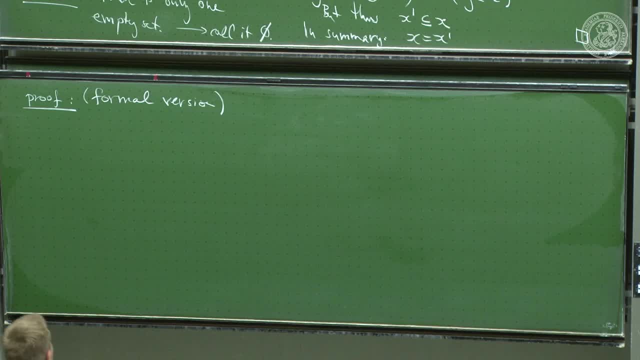 no, no, neither direction. neither direction, which is easy to check. find counter examples for both directions? ok, but I appreciate the question. so the formal version. how does that work? well, the formal version. we have to encode our assumptions as axioms. and what's the assumption? 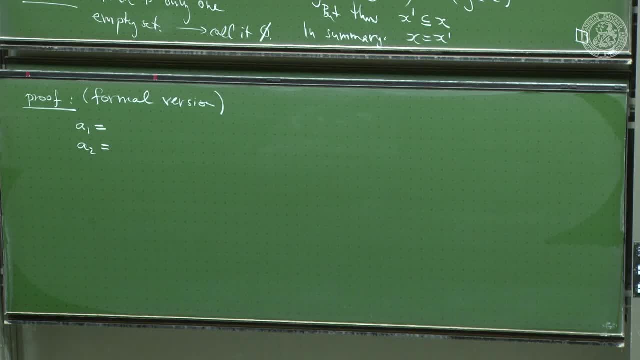 well, the assumption is x and x prime are both empty sets. so we assume we have here for all y y not an element of x, and the second assumption is for all y y is not an element of x prime. these are two assumptions, namely. I mean we'd say 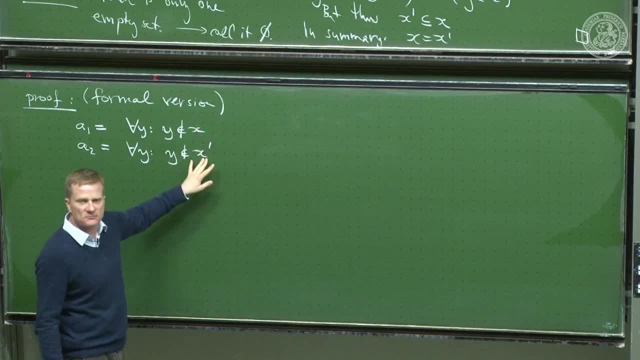 ah, this means x is an empty set. this means x prime is an empty set. that's right. and now we need to write down a string of further propositions. well, if you want to be very picky, propositions are not equal to each other. they're equivalent to each other. 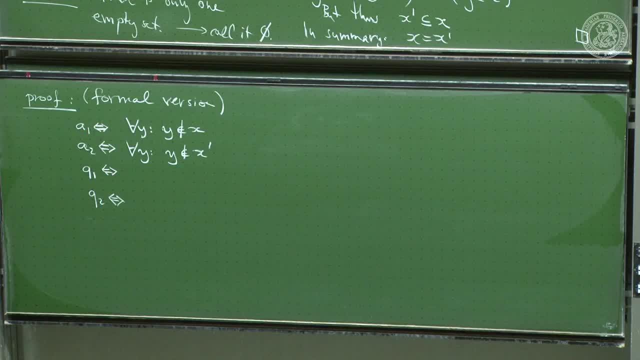 so if you want to be very picky, we have to write this. ok, we should be picky, maybe. and finally, we want to arrive down here, at the statement we want to write down here, we want to prove so at some mth step m to be determined. 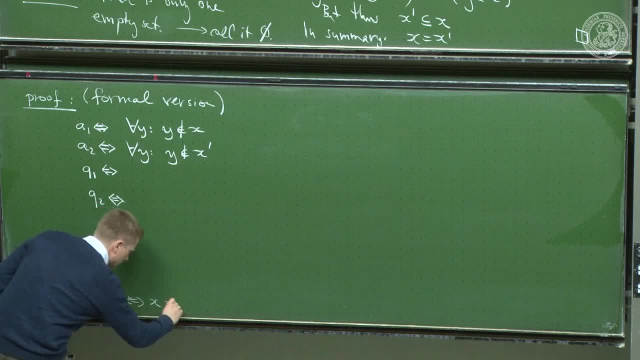 we want to have the statement that x equals x prime, and the task is to find these steps in such fashion that for every step of the proof. so these are the axioms, axioms of our system, meaning assumptions for the proof, because, apart from this, we only want to use 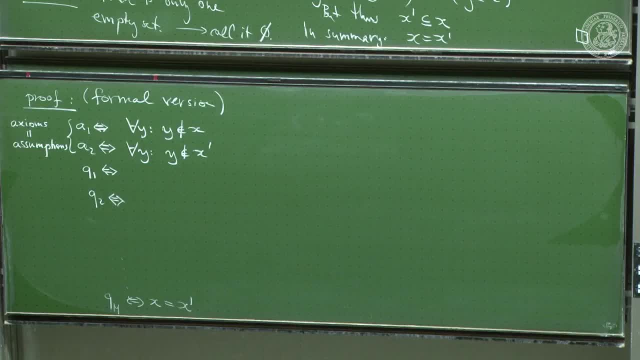 the definition of x prime. well, we only want to use propositional logic. so therefore, these amounts of the assumptions, because propositional logic only would be an empty set of assumptions. now we have the assumption: x and x prime are empty sets. so now we need to find 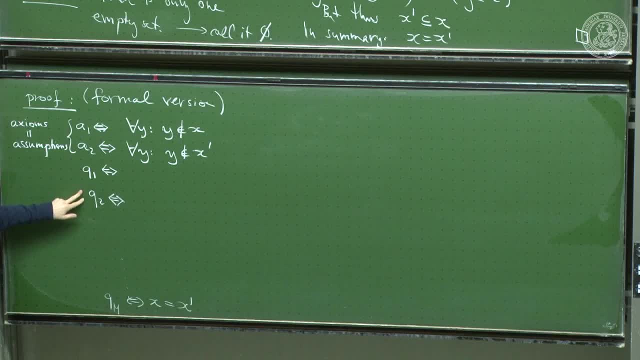 such steps, such that we arrive here and that for every step we can tell which of the deduction steps: t, tautology, a axiom or m modus ponens, which last time I wrote down in the definition of a formal proof justifies this particular. 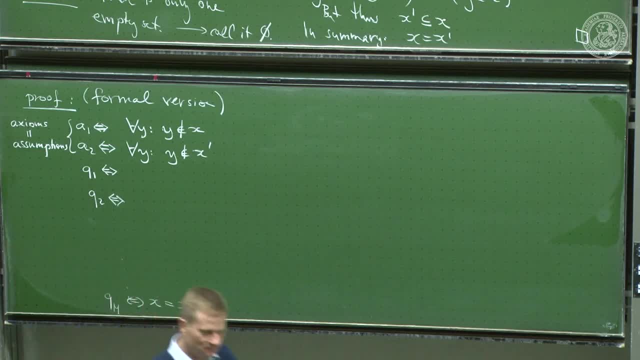 step. so ok, so how does this start? well, the first thing we write down a tautology, and that is: if for all y, y is not an element of x, that implies that for all y y is an element of x implies y is not an element of x. 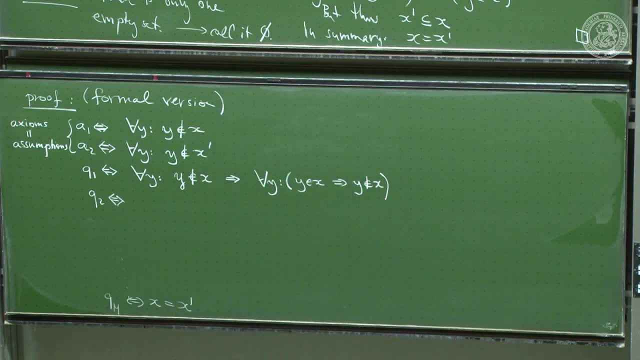 let me see. well, this is what. let me see. this nonsense is an element of x prime. that's what I wish. it doesn't matter. I can again write here what I want. so I want this. so well, why is this true? well, you see, here, this would be true. 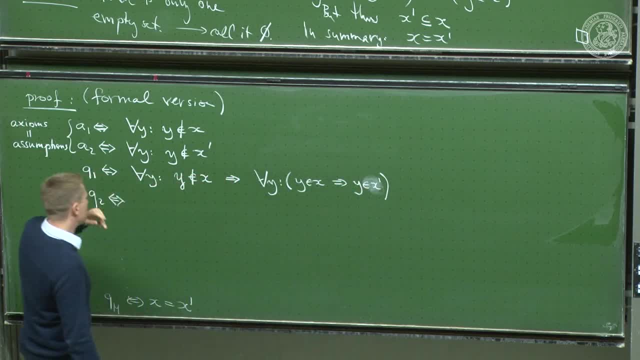 well, if for all y and x, this is true, this is implied. but if I make it a condition that y is not an element of x, then x, this thing is true. so if you put the brackets here right, that means the brackets around here. I don't need to write them. 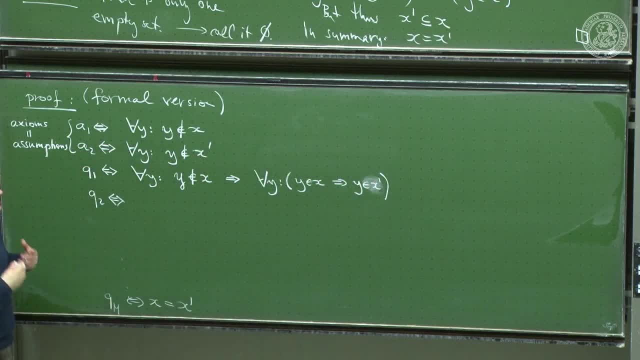 brackets around here. this whole thing is just true for any y, x and x prime. this is simply a tautology. so the reason why I can write down this q1: it's a tautology. ok, so right. so now I pull one of the axioms. 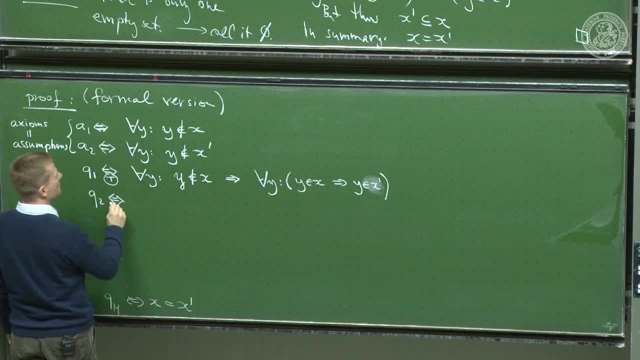 I take the first axiom so I write: q2 is the proposition for all y. well, it's a scheme of proposition. y is not in x. why can I write this down? well, by deduction rule a, you can pull any of the axioms into this list of steps. 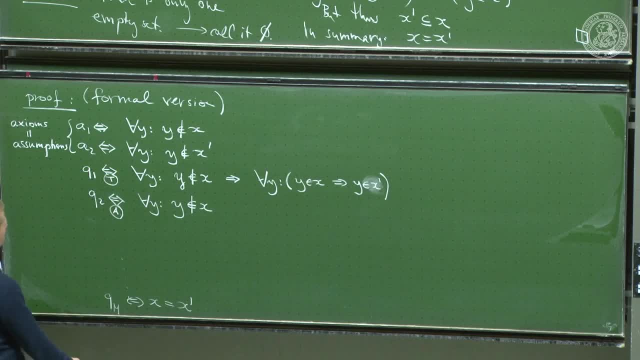 ok, compared to the definition of proof. and then q3, we use the modus ponens. that's the third deduction, rule m. what did it say? it said that you take two steps, two prior steps of the proof. well, there's only these two, and you put: 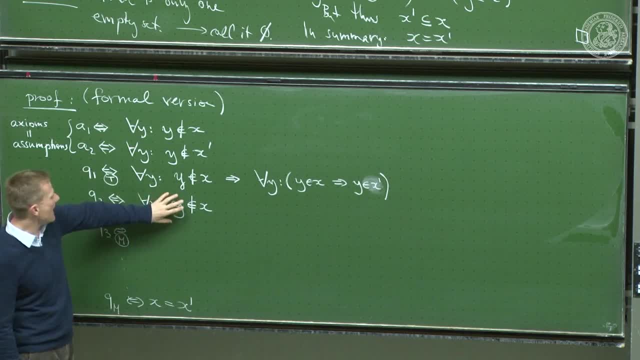 an and between them. so you take this and this and this whole thing, and what you then can write down here is something that follows from this, in the sense of you take q1 and you take q2, and then you can write down q3, if the implication 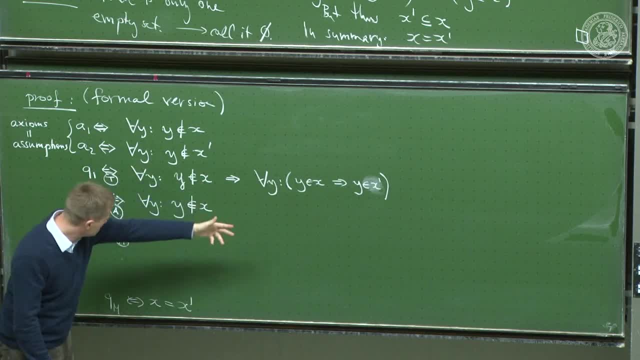 that this one and this one gives q3 is a tautology. that was the definition and it turns out that if you take this and this, implying this for all, y, y in x implies y in x prime actually is a tautology. so you can postulate: 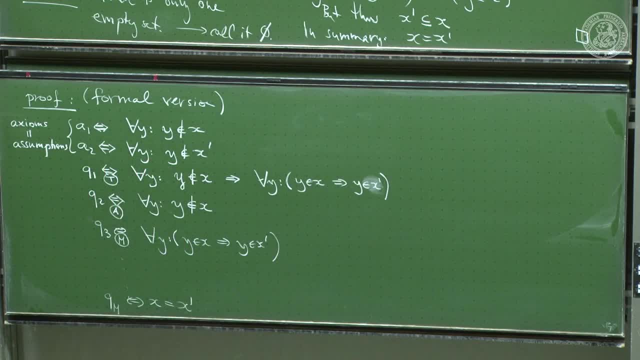 now you can put the q3 of this shape into the list, okay, so this is certainly something you probably want to have a look at again at home and very carefully check the definition of what a proof, what constitutes a proof, and you will find that it is a proof. 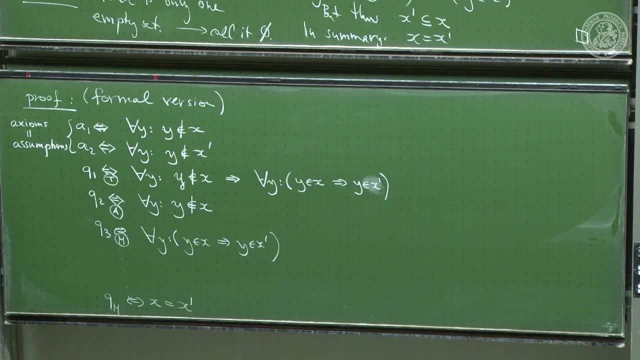 and you will find that this is the deduction, rule m that allows you this. now, this, however, is just a short form, so we can immediately we recognize that this statement just means x is a subset of x prime, exactly our definition. so, for our own thinking, which? so it's just. 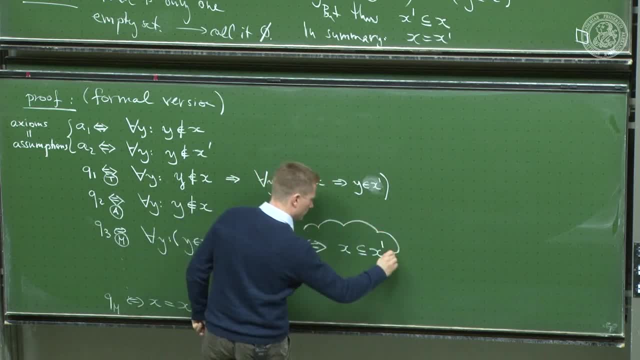 an abbreviation of x prime, which is an abbreviation to write that this statement is just: x is a subset of x prime, and so you see, this is also something we arrived there, well, almost in one line. here we used a number of lines. well, because this is a formal proof. 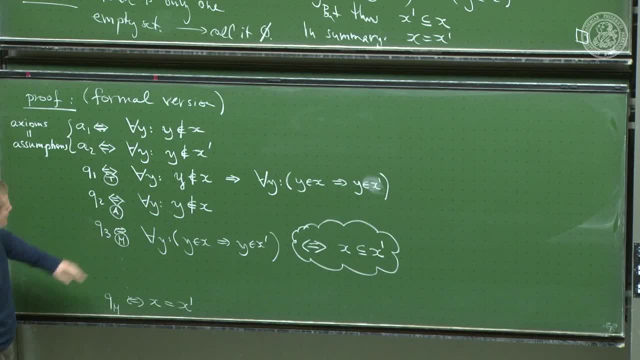 I shouldn't write similarly, but it's totally clear that you now do steps q4, q5 and q6, which are really similar. ok, let me write them down quickly. you again employ a tautology. you say for all y, y, not an element of x prime. 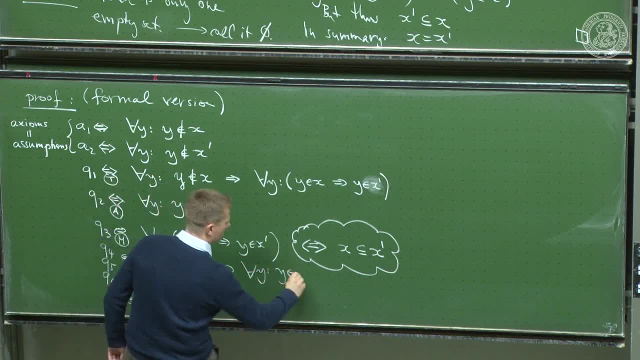 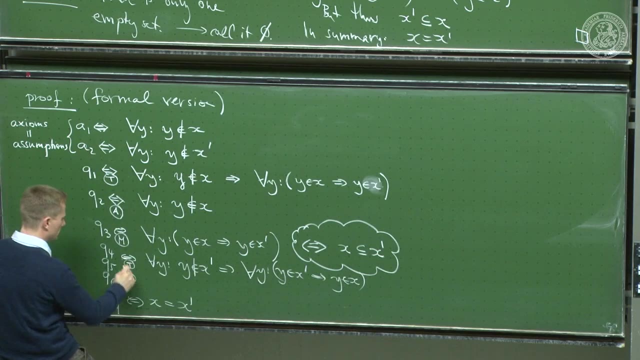 implies for all y. y in x prime implies y in x, because this is a tautology. q5. you pull the second axiom a2 down here, and so you write for all y, indeed y not an element of x prime- and then for q6 in exactly the same fashion. 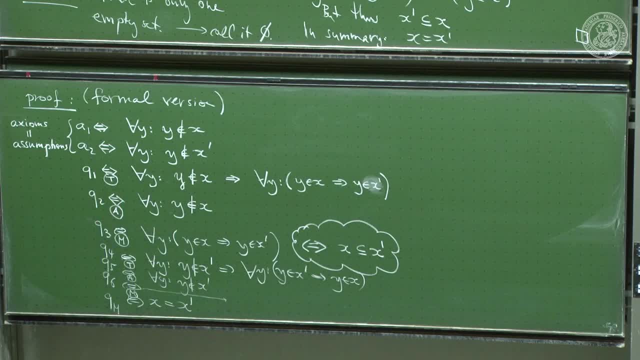 over here. you can now conclude that q6 is a valid step of the proof if it has the form for all y. y in x prime implies y in x, which again in our theorem- I'm thinking well in this short form- means x prime is subset x. 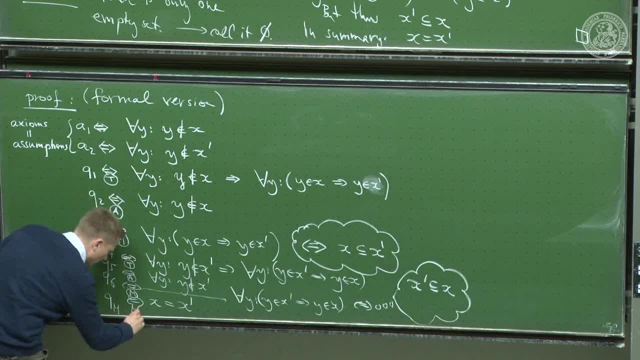 and then you again can invoke the modus ponens and say: look at two previous steps in the proof, in this case look at. I should write down so: this modus ponens used 1 and 2. this modus ponens used 5 and 6. 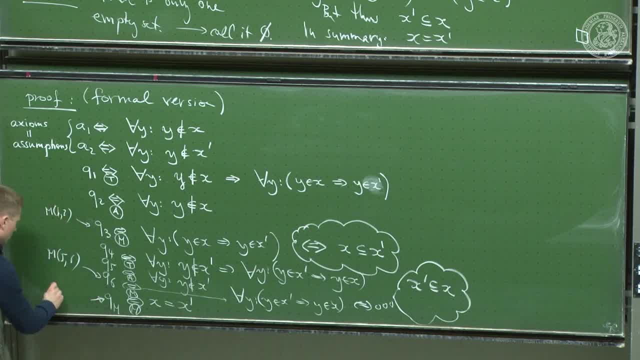 and this modus ponens here is: x used steps 6 and 3. no, it used 4 and 5, I'm sorry, 4 and 5 and this used 3 and 6, and you can check that. obviously, this and this implying. 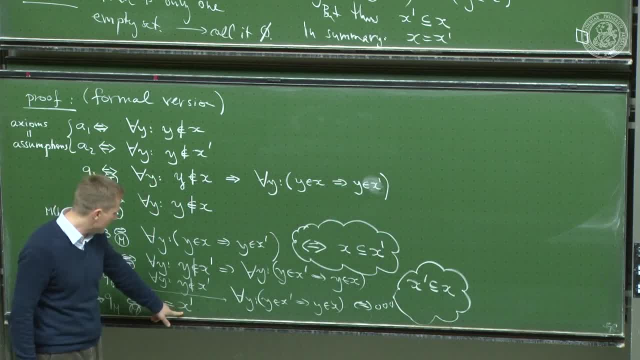 this is a tautology, hence you can write this as the 7th and final step of the proof which says the two empty sets are the same. this is the formal proof and obviously it is nothing more and nothing less than breaking down the standard textbook style proof. 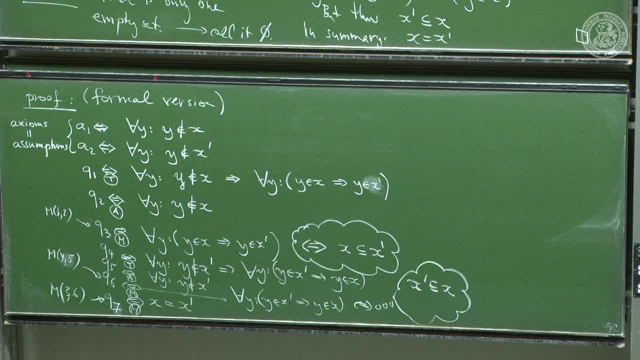 in a really pedantic manner, but we are certain now this constitutes a proof: there is really only one, just one empty set. so you see, we took the whole thing on two levels from the kind of standard mathematical language formulation. there exists a set that contains no elements. 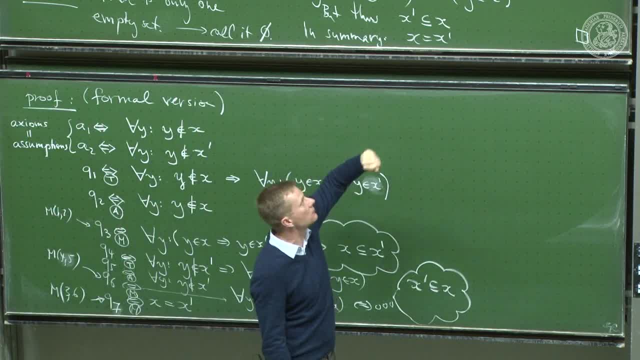 that kind of corresponds to this kind of standard textbook style proof. or we can be very precise and use our first order, predicate calculus, predicate logic, and then mirror this in this very formal version of the proof. this is how. that is the spirit of axiomatic set. 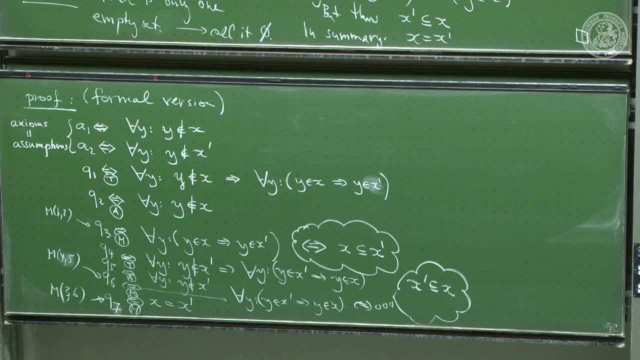 theory. you are just very precise about what you are going to say and you have got to be very precise. however, we are not going to follow this very strict formal proof technique any further in this course, because the proofs get longer and longer and longer, and there is 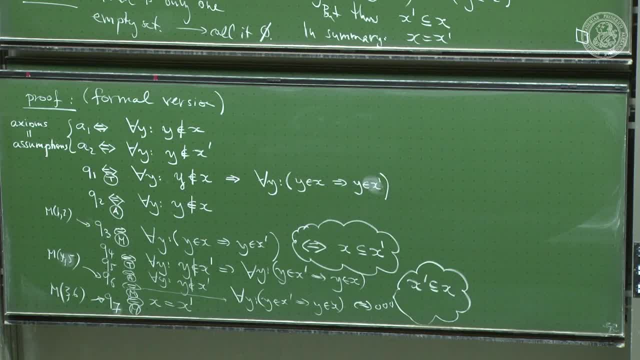 actually no book of mathematics that spells out all the proofs for all the theorems it proves in this fashion, because it becomes practically impossible. but it shouldn't be impossible in principle. so that was what I already was hinting at last time, that in principle you must. 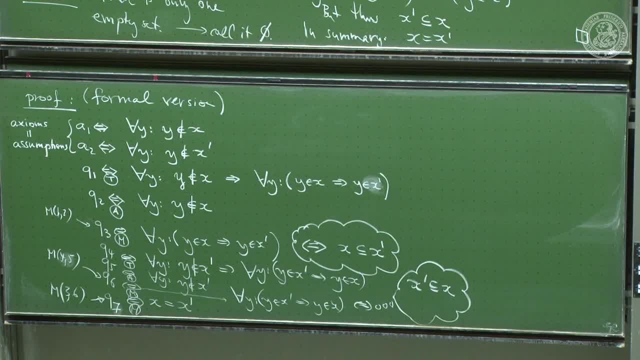 somebody presenting a proof must be able to break it down to this level, although in practice, this is certainly well, hasn't been done for anything serious as far as I know. ok, so where are we? I should note this: EE, perp, IC, F. so we got this. 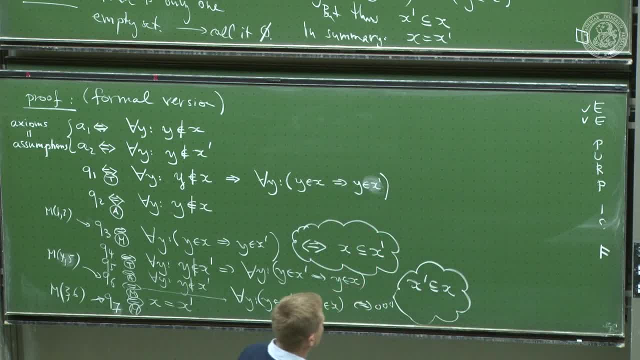 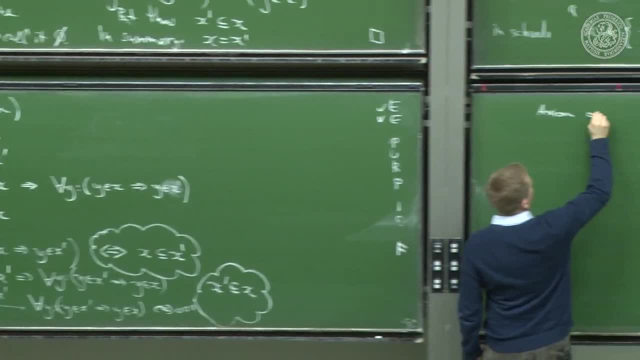 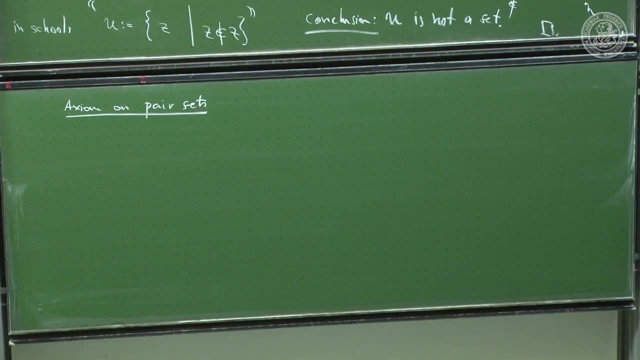 one and we got that one. there are seven more to go, so the next is the axiom on pair sets. it's a bit tiring to go through all the nine axioms, but on the other hand, this is the foundation for all of mathematics, so it's. 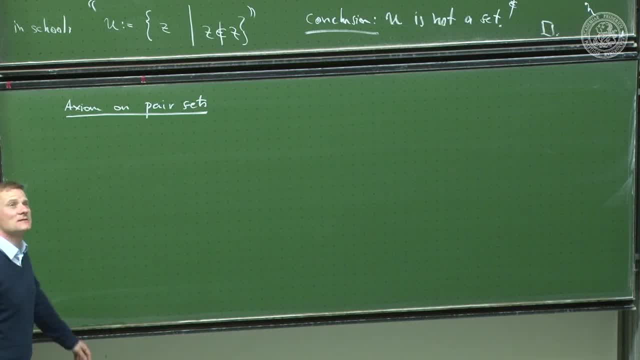 worth it right? what is it for a number, for a field like the real numbers it's? it's also nine axioms to define a field: commutative, associative, neutral, inverse for plus, same for the multiplication and one distributive law. so I mean certainly to build. 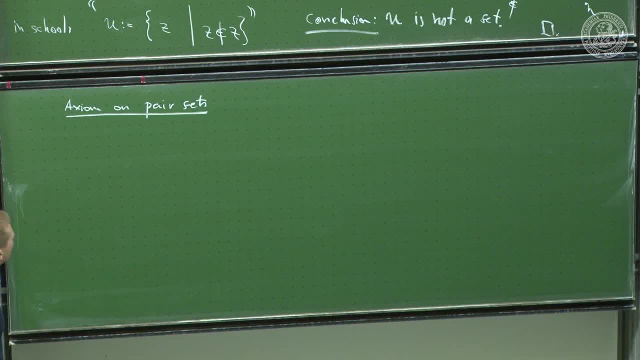 all of mathematics on these nine axioms is not too bad. so the axiom on pair sets is the following: let x and y be sets, then there exists a set that contains as its elements precisely the sets x and y. that's it so. and the key word. 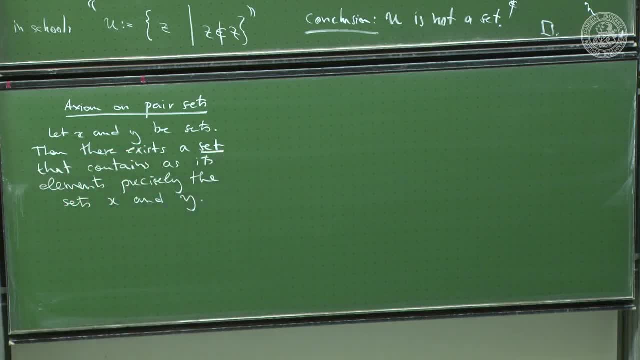 is: there exists a set. that means you take one set, you take another set and you put them together as elements of a new set, and this new thing you constructed this way is a set, and that is what this axiom assures us of. so there is okay, okay. 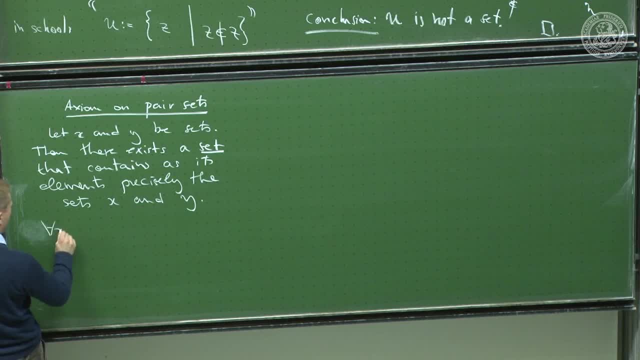 how do we write this? for all x and for all y? there exists a set, let's call it m, such that its elements are precisely those, such that, for all u, u is an element of m if, and only if, u is x or u is y, for any. 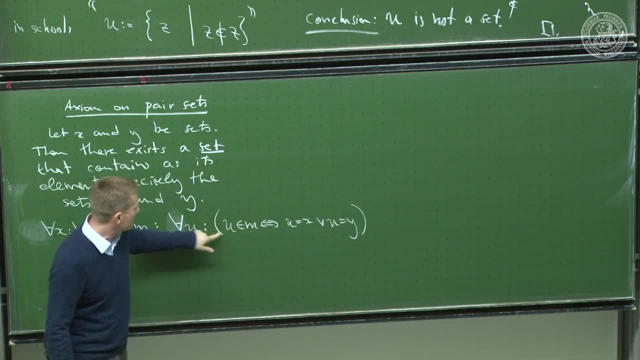 sets. there exists a set such that all its elements or that its elements are precisely those, that is, either x or y, would be the exact formulation. the usual notation for this is: denote the set m. this set m by x, the elementary school thing, the set with the elements. 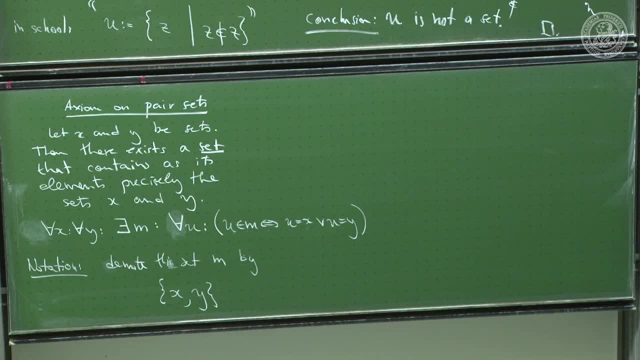 x and y is denoted by open a bracket, x comma. next element: close the bracket full stop. okay, but that, this construction, I mean I can write this down. all right, and I could put a little flower on the right upper corner as well. right, I can write. 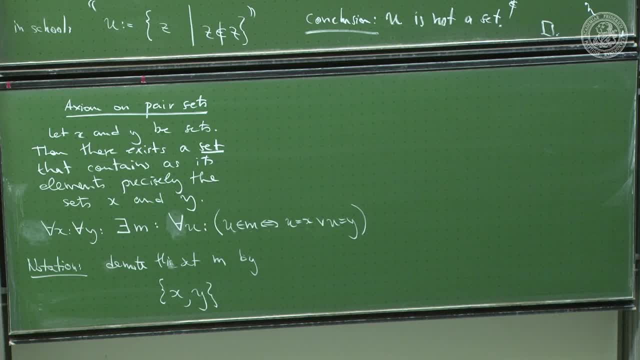 down what I wish, but what the axiom assures us of is: if x is a set and y is a set, then this whole thing counts as a set is a set. we need to have an axiom that assures us of this. now there might be an initial worry. 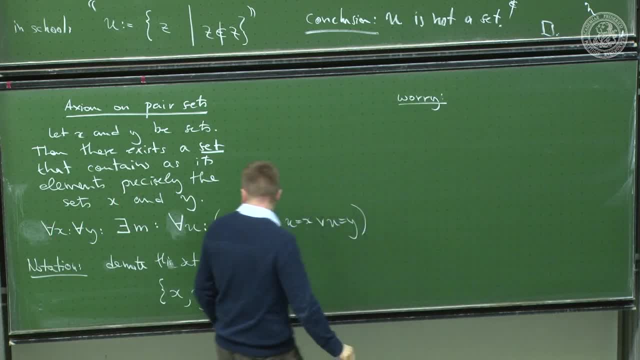 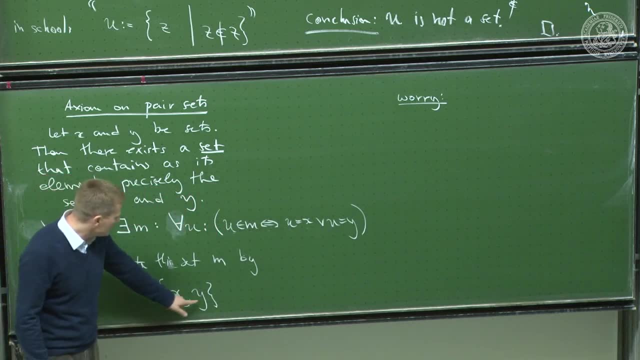 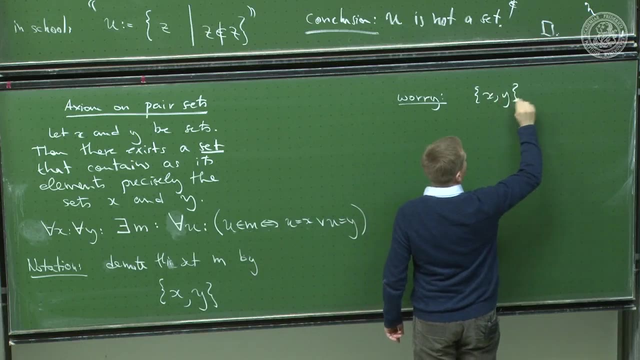 and that is why didn't I call it the set y and x. why do I call it the set x and y? I introduce an order here. right worry: is x, y the same as y x? this thing is defined between sex assets. is this the same the answer? 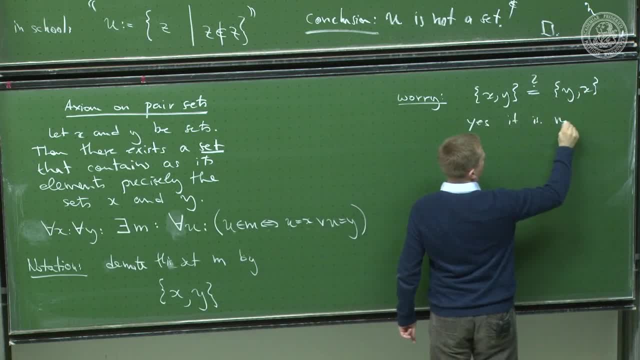 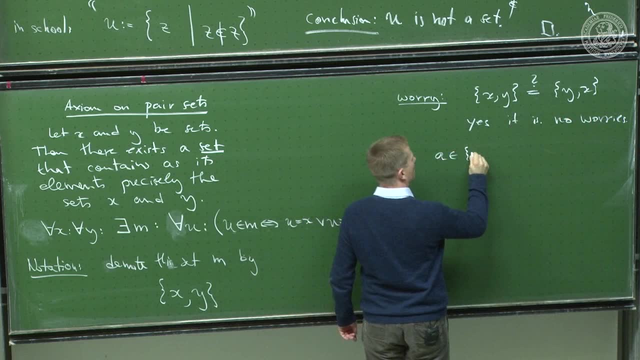 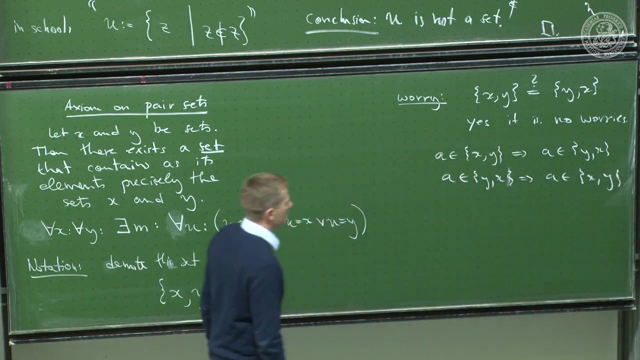 is yes, it is no worries. why is it? well, if an- a comes from x- y, that implies that a comes from y- x, and if a comes from y- x, that means a comes from x- y. how do I know this? well, by employing the element relation and start. 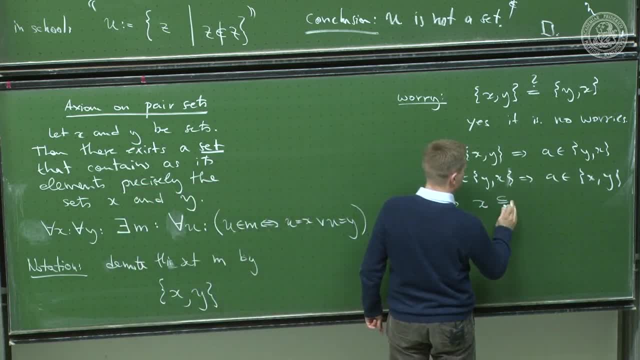 stuff like this. that means x is a subset of- sorry, that means the set x- y is a subset of the set y- x, but also the other way around. so in total they are the same. so our notation doesn't introduce any prejudice or what you learn in. 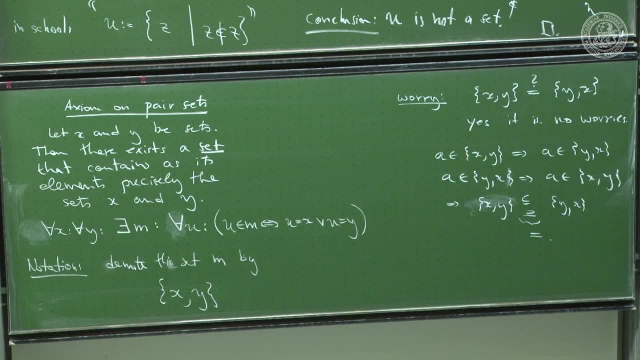 elementary school is: the order doesn't matter. we agree the order doesn't matter. no, we don't agree on it, we prove it. okay, but that the whole thing is a set x, guaranteed by the axiom on pair sets and by the way. so one more remark. well, 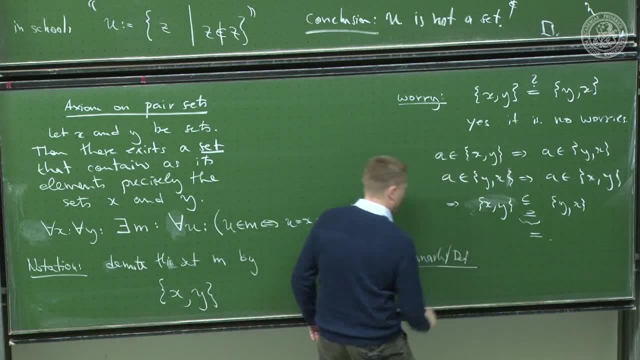 if you want remark definition, it's really trivial. the pair set axiom also guarantees the existence of sets of one element, um, if i write this: i take a set x, so the x is a set. i take a set x, then i define the pair set of x. 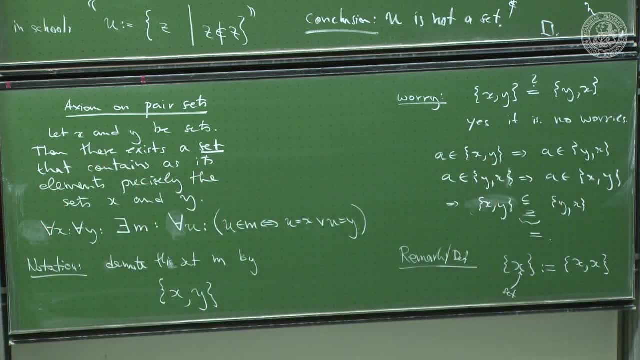 with x. oh well, if x is a set, then x is a set, then i can use the pair set axiom and i call this the set of one element. and by a similar argument is here you can see you have the x in there twice. but because equality. 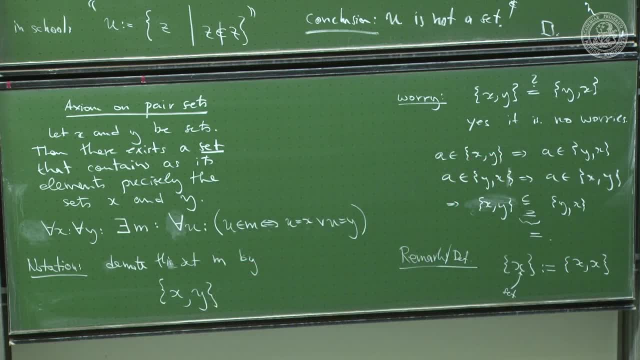 is defined by the element relation, the element, the pair set with the elements x and x. there is no more information than that. x is in there. you can think about that too. so what we have from the pair set axiom is we have these one element sets and 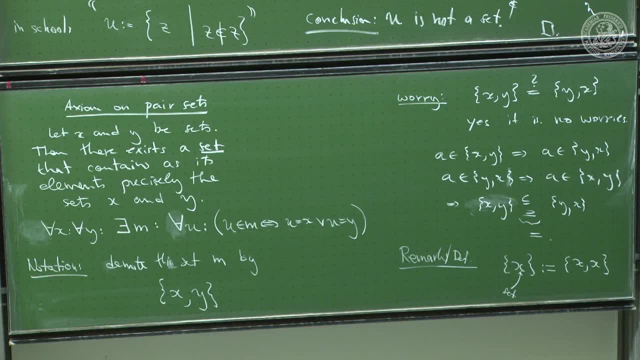 we have two element sets. that's it. at this stage, there is no justification to write down for sets x, y z. a set with the elements x, y, z, it's not defined, okay, it's not defined, but we have these two. however, the pair set axiom will: 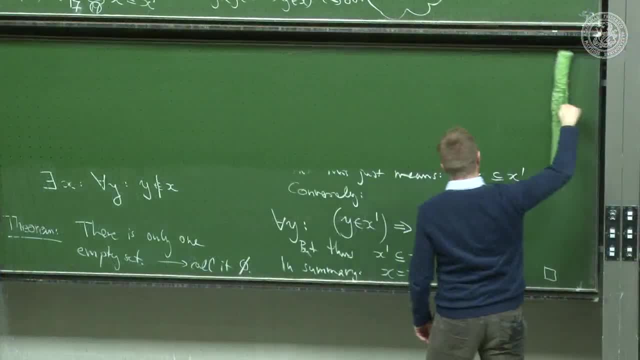 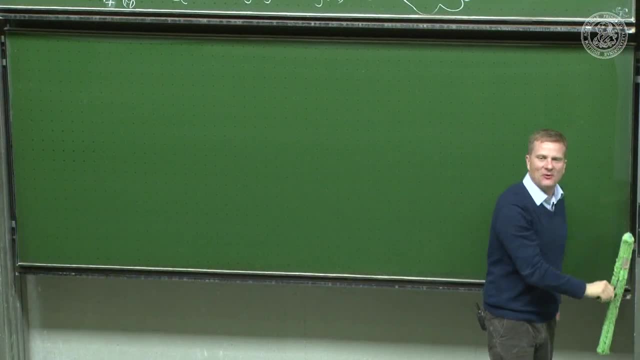 make its appearance again very soon. so probably the most demanding task at this stage is to get rid of old prejudices about what a set is and what the whole thing means, and to free your mind from that in order to appreciate the systematic definitions that we make and 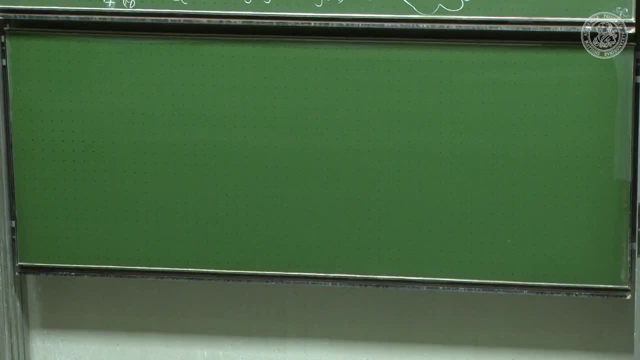 some of the things you thought you can do with sets will simply not be allowed by the axioms we write down. but therefore we must appreciate how what we already knew is consistent follows from the axioms. it's a little like learning about well number fields or 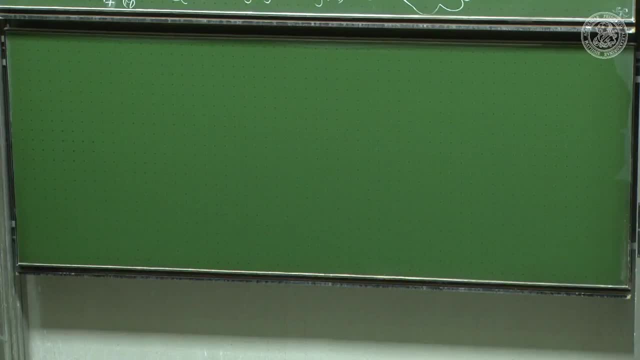 groups or whatever, and realizing that, say, the commutative law between real numbers, is something special. you have to write this down as a law in order to use that. a plus b is b plus a and okay, fine, so it's the pair set axiom the next. 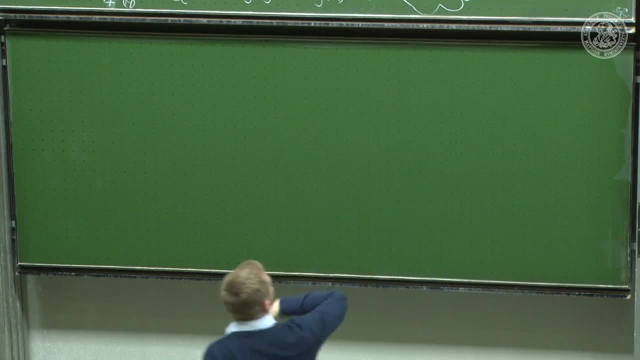 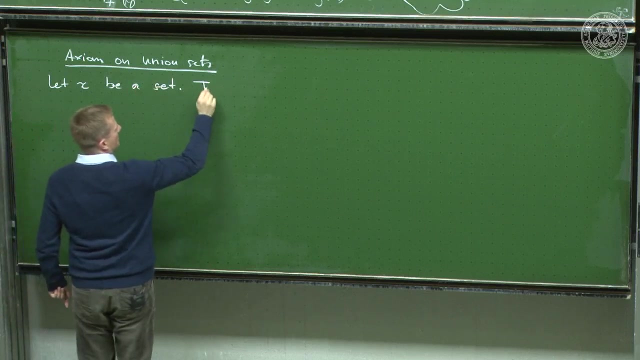 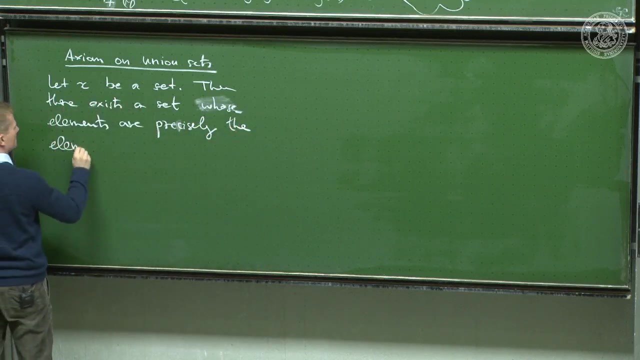 thing is: in our e we have the p, the u is the axiom on union sets. axiom on union sets takes the following form: let x be a set, then there exists a set that contains whose elements? whose elements are precisely, precisely the elements of the elements, the elements. 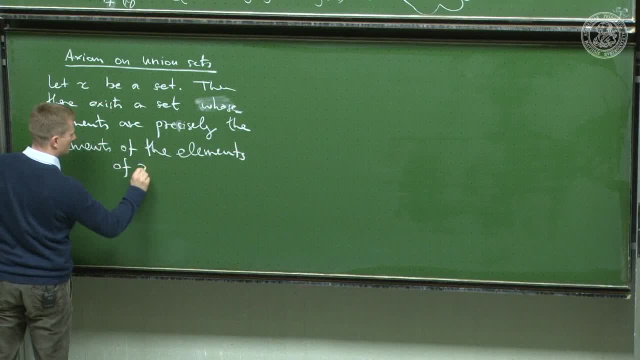 of the elements of x. okay, so we have a set of elements of the elements. so this, so I leave it as a homework for you for all the further axioms that I write down, to convert this language description, which should be clear in the standard sense, to convert it into: 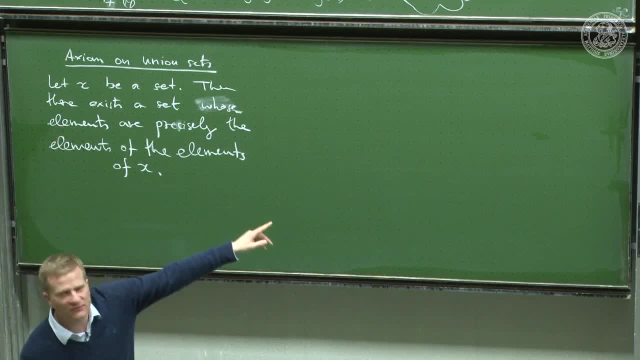 first order predicate logic statements of this type. it's a very good exercise in order to make very precise what you mean. so if you think you understand it, what it means, put it in first order, predicate logic language- then there exists a set whose elements are precisely elements of the elements of x. 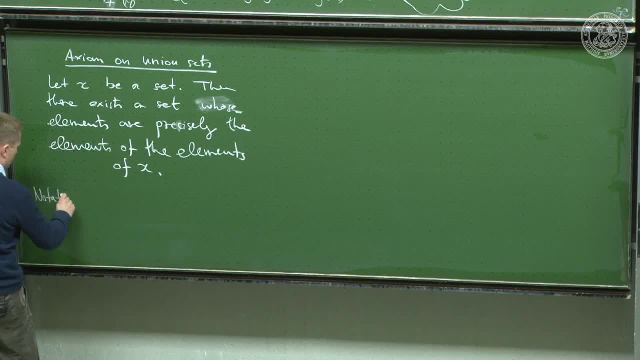 notation, maybe you expected something different from union, don't? you need at least two sets in order to build a union? well, the set x is already the collection of all the sets that are to be put into the union. so, notation, there exists a set. let's call it u. 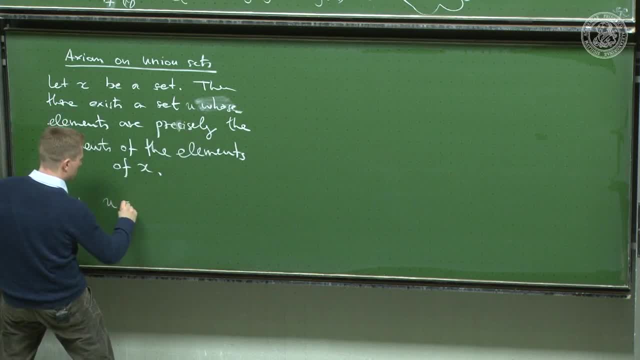 notation u is usually written as a big cup and behind it you write the x, but still doesn't quite look like the elementary school thing. so let's write down an example. as an example, let a, b and c b sets. ok, we start with sets a, b, c. 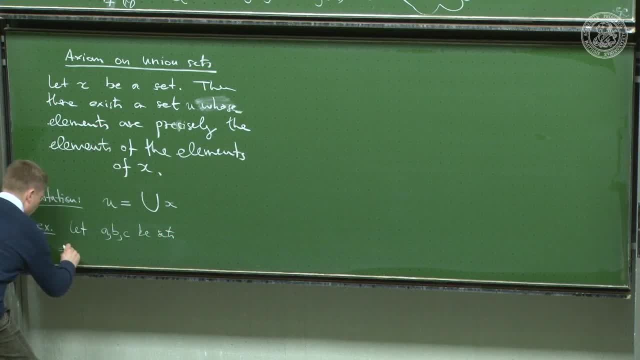 and then it follows that: what do I do? I take the set with the element a. what do we know of this? if a is a set, we know this. with the brackets around, it is again a set. how are we guaranteed that this is again a set if a is a set? 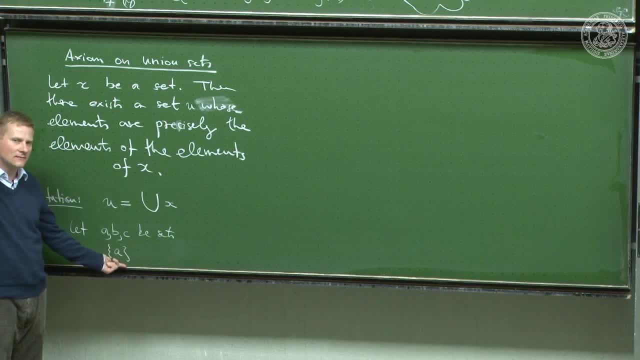 which axiom- pardon me, the pair set axiom- exactly. take this one. now. take the set b c, the set with the elements b c. again, the pair set axiom tells us this is a set because b and c are sets. so this is a set and this is a set. 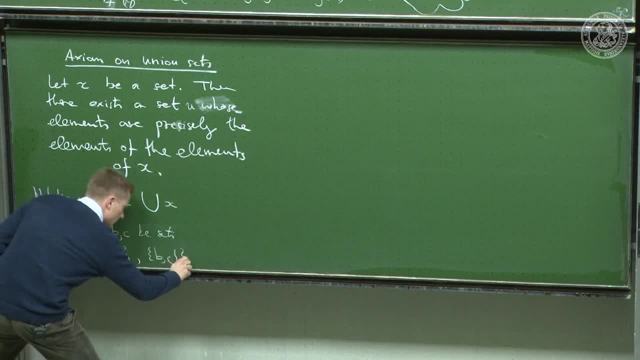 so I can put them together into a set. is that right? how am I guaranteed that this whole last line is a set? again, the pair set axiom step by step. so this is a set. well, let's call this set x. let x be a set. alright, we constructed a set x. 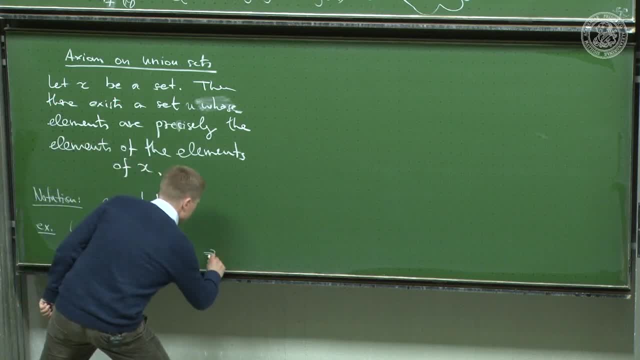 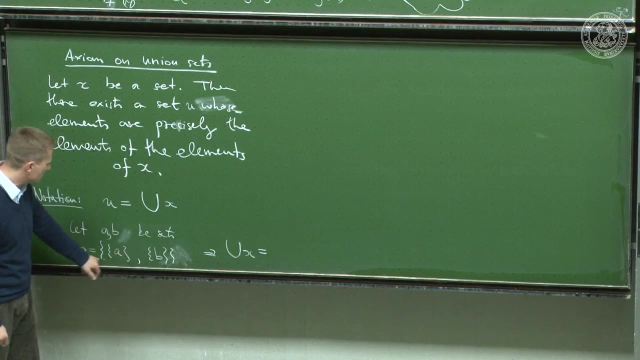 what is the union of x? well, the union of x contains all the elements as its elements precisely. let's only use one element set. here the example is a little bit more elementary at this stage. a, b sets. this is a set by union, set axiom, pair, set axiom. 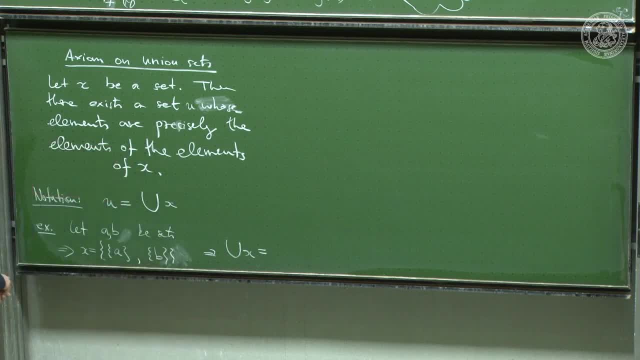 again, pair set. axiom x is a set. now what's the union of x? it's the set that contains precisely the elements of the elements of x. the elements of x are the set with the element a and the set with the element b, and it contains the elements of the elements. 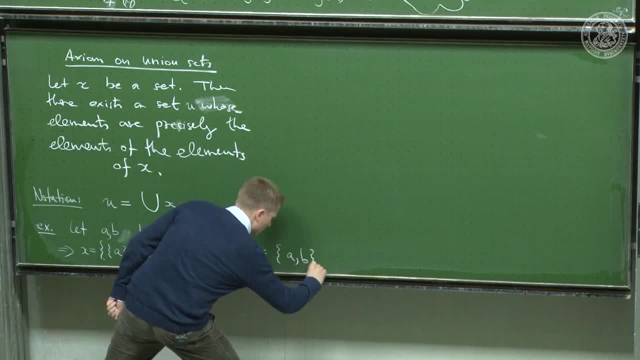 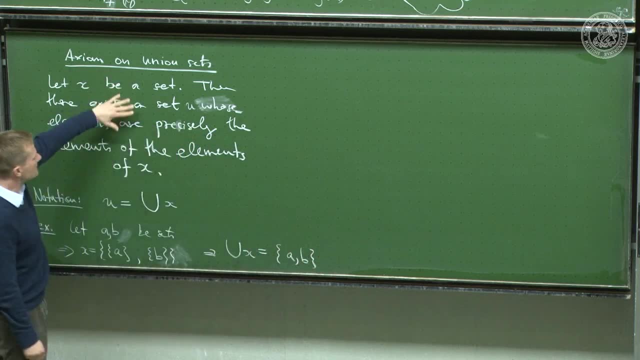 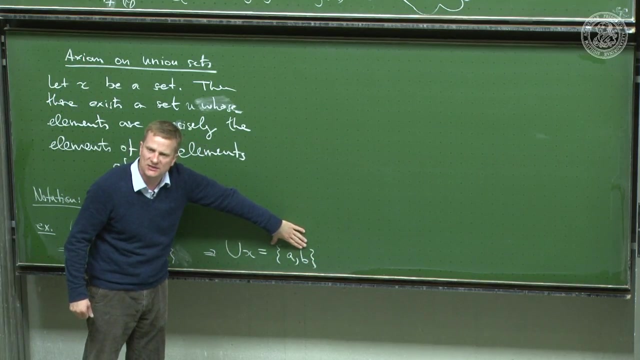 so it's the set a, b and we already know this is a set and that is what the union set axiom assures us of. what comes out here is a set. independent of whether we previously know it's a set here, we knew previously this is a set. 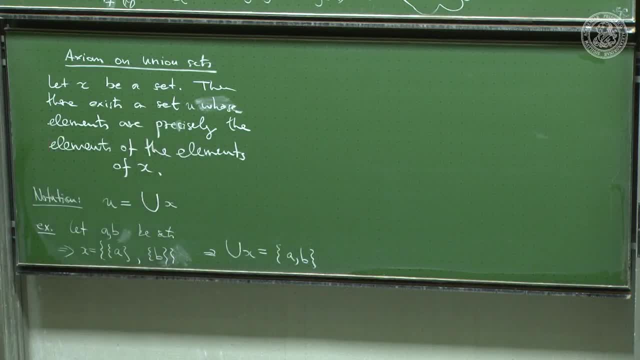 but the union set axiom says it's always a set, whatever set x you started with. so the second example would be: so, second example: we know that if we start with, x equals a, b, c. so the example I first wanted to write down: we know this is a set. 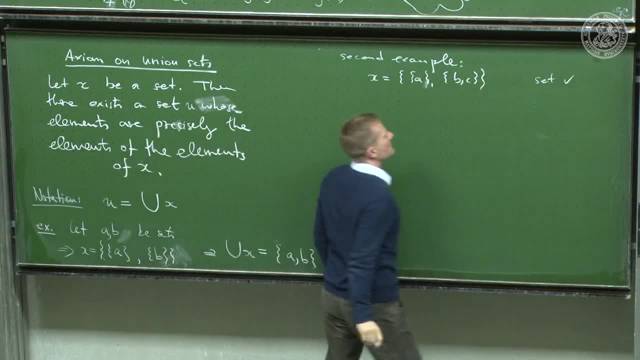 that we already know it's a set. alright, but this is a set. but this is a set, but this is a set. but then it follows that the union of the elements, of the, of the- yeah, the union of x is a set. why? well, because of the union set axiom. 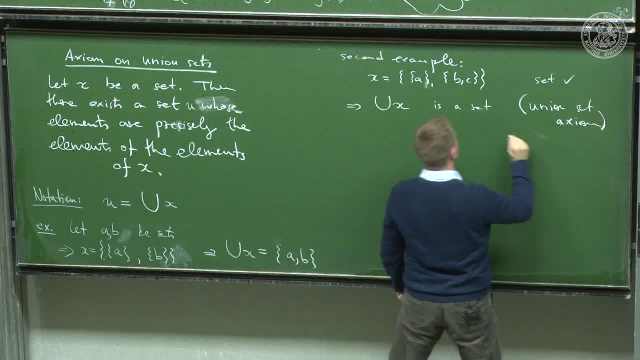 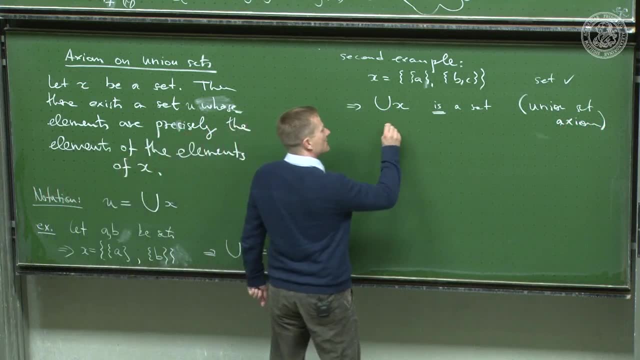 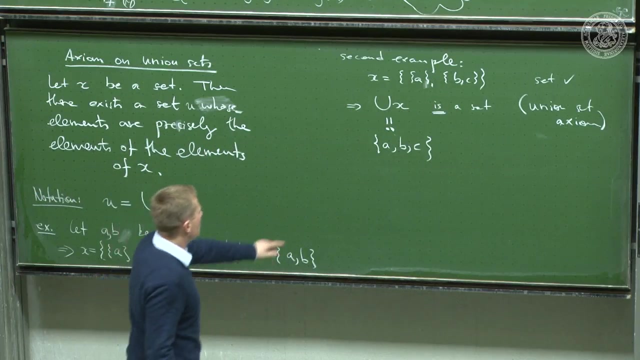 this is a set and this set deserves a name. if it's a set, it deserves a name, and so I define a b c, a b c the three element set. I define in this fashion from two element sets. ok, so how do I know? this is just a symbol. 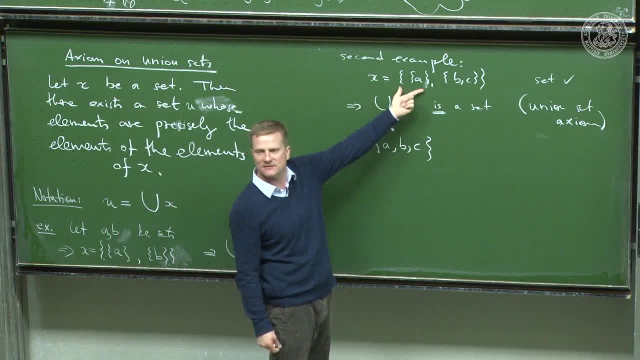 again, this is just a notation for this thing- if x is given like this, but that I know that the object is a set, that I know from here. ok, I mean, in elementary school you learn this is a set, but how do you know? it's just claimed. 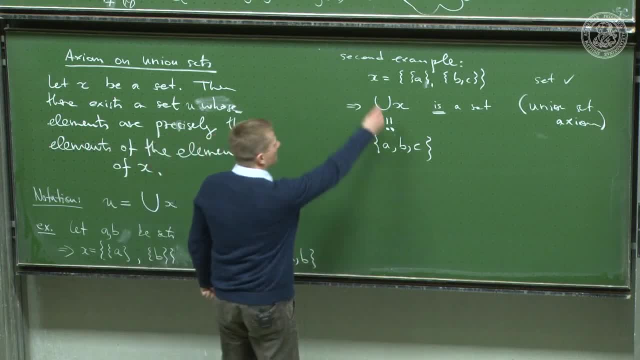 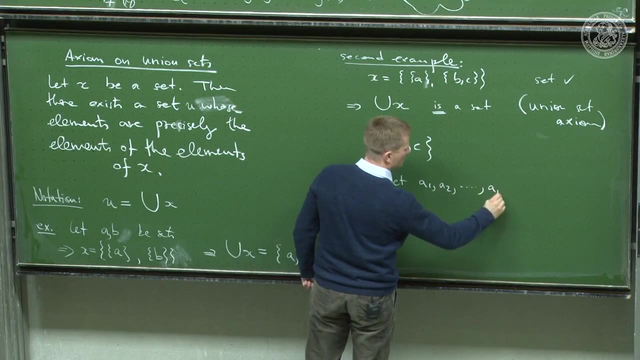 now, the axiom tells you this, and so, and of course, the second example immediately generalizes to a definition. the definition is this: let a1, a2, dot, dot, dot, dot to a n again. what are these numbers? again, the Bavarian beer. counting numbers: one stroke, two strokes. 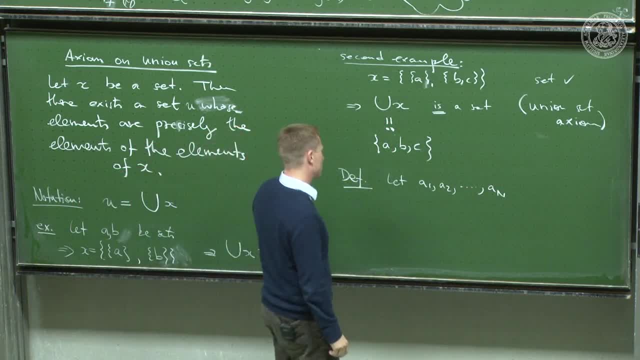 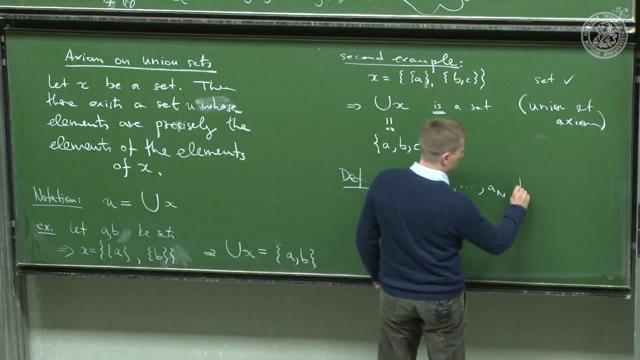 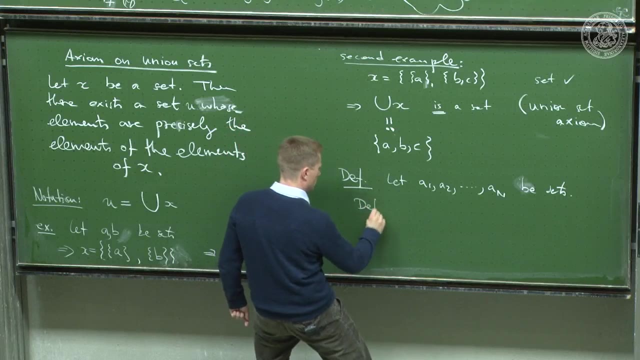 three strokes. they are metamathematical numbering. if you want, I could call them a, b, c, d and I could do this for all instances that a1 to a2 and b sets, and then define recursively the symbol a1 to a- n. I put them all in brackets. 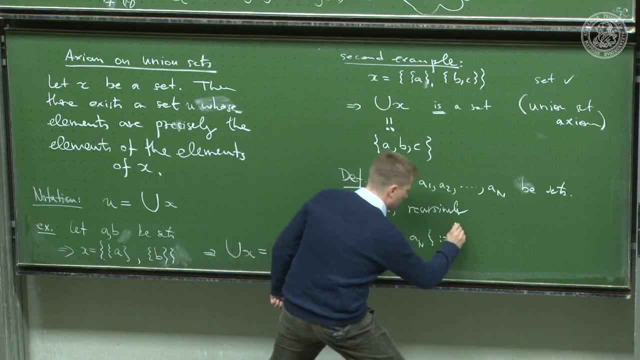 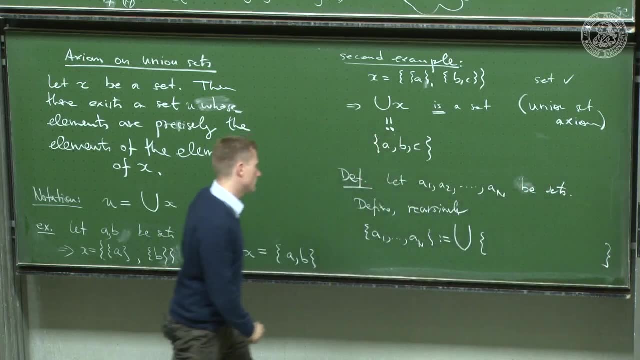 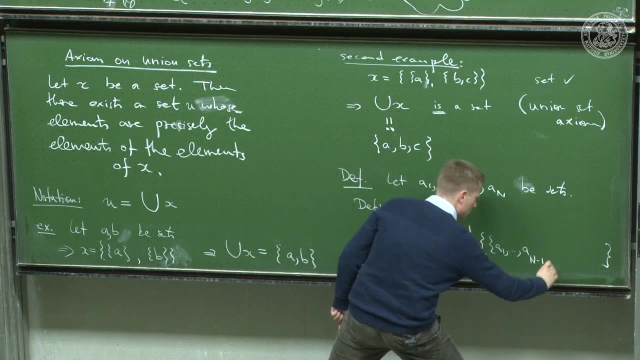 what on earth is this supposed to mean? supposed to mean the union of which set? there must be one set behind this, whose elements I take and put into the union. it's the union of a1, dot, dot, dot to a, n minus one is the metamathematical. 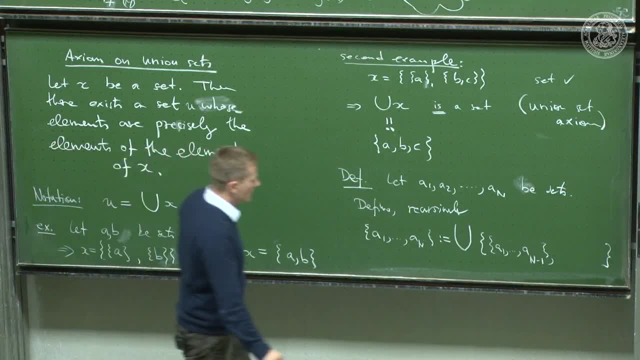 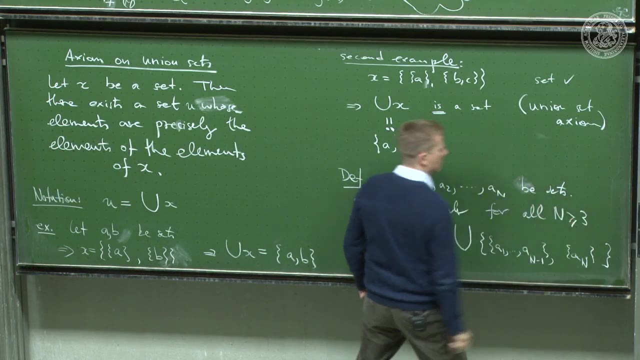 subtraction. you take one stroke away with the one element, set a, n, and you define this for all n greater or equal to three, because for n equals three, n equals one and n equals two. this is this. recursion is started by the pair set axiom. but now this defines: 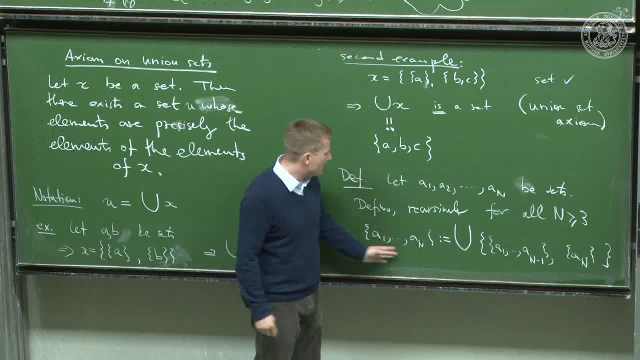 anything that we would informally call a finite element set with specified elements. you get it this way by a combination of the pair set axiom. you already know from the recursion set. before this is a set and this is a set, then you use the pair set axiom. 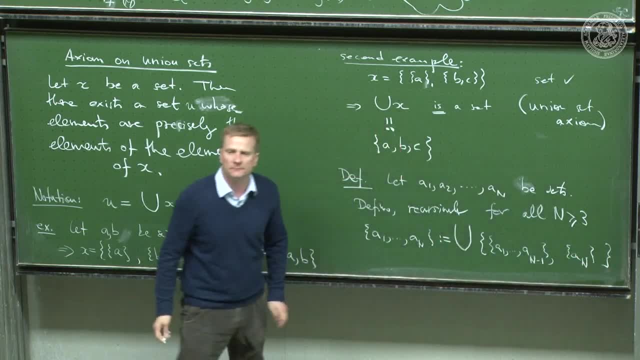 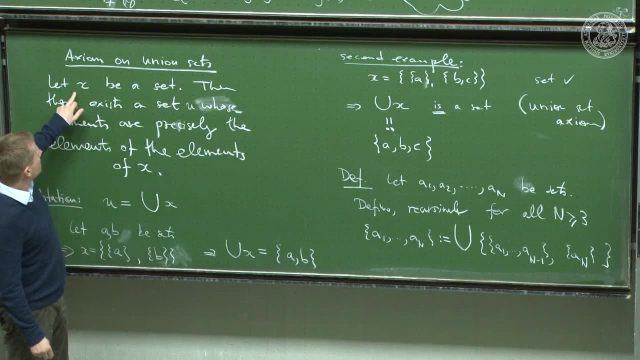 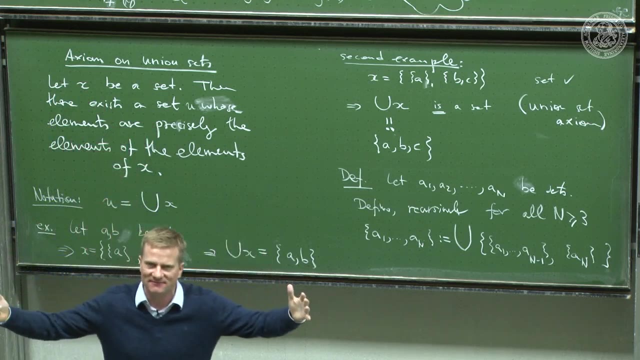 to write down the set of which you take the union, and then you have the set of which you take. now, the big thing about x- assuming that you can collect all the sets that you want to unify in a set, is an assumption. you see, because you remember. 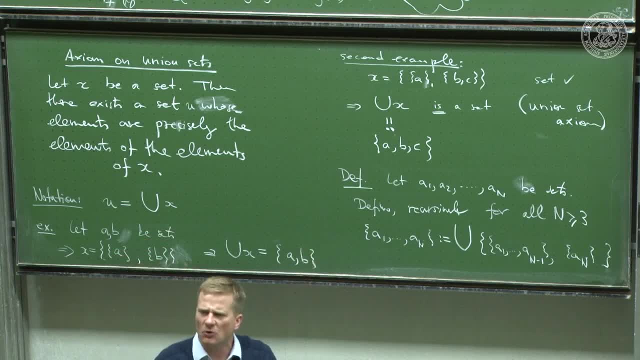 Russell's paradoxon. there we had a u that contains all the sets that don't contain themselves. this u is not a set. so this u, this Russell u, which is not a set, could never be put here instead of the x in order to make a union. 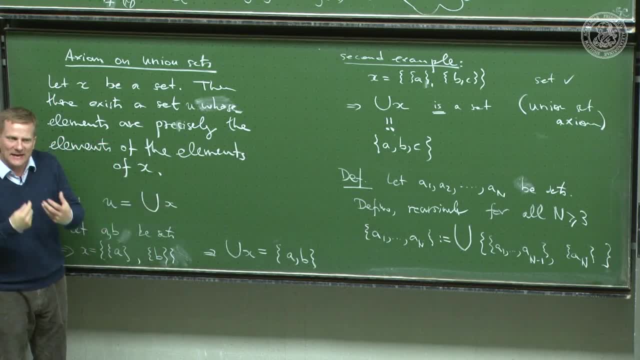 of all its elements right. so it's a big restriction that you can build unions only of- let me informally say- as many sets as still fit into a set. you could take more sets than fit into a set, like, for example, the set if you take all the sets. 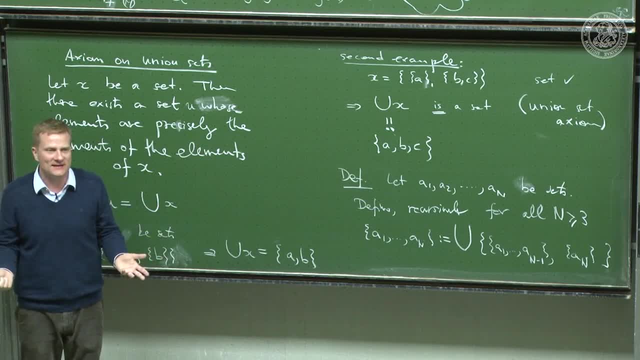 that don't contain themselves. you cannot collect them in a set anymore. ok, so you could never take their union. this is the big thing about writing down this. it's much more than saying: take only finitely many sets and put down the write down the union. 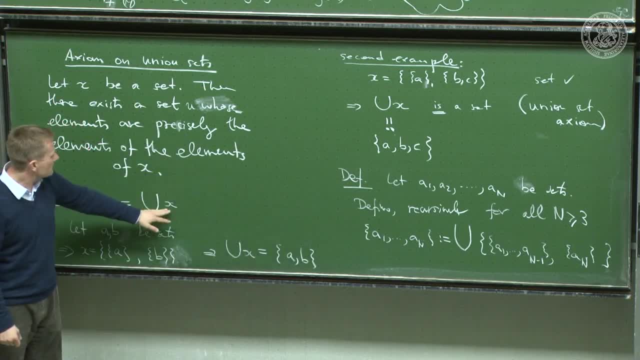 that's quick. yeah, yeah, yeah, but the idea to certainly contains an idea of taking infinitely many sets, roughly speaking, but it doesn't mean taking more sets than fit into a set. that wouldn't work. you see, this is subtle, but also very precise, and now we probably 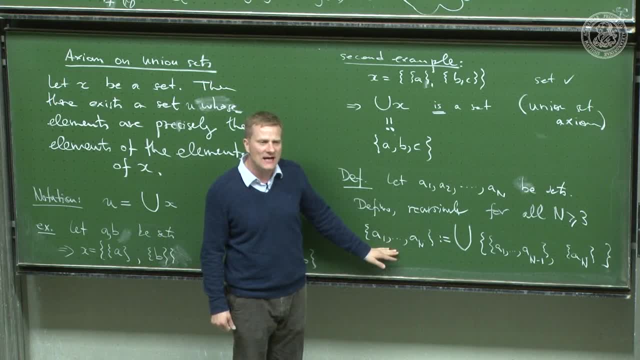 got back all the elementary school ideas at this point. a set is a collection of elements. well, what is that supposed to mean? but now we know very clearly what a finite. you take elements and you put them into the brackets. but you see, this is just a symbol. 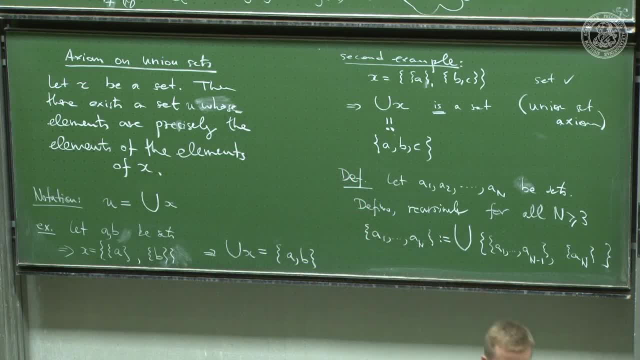 that this constitutes a set in the sense of set theory is guaranteed by the first four axioms we had, by the E, E, P and U. ok, there's the replacement axiom. let me perp. perp is just nice, but it's actually popper. 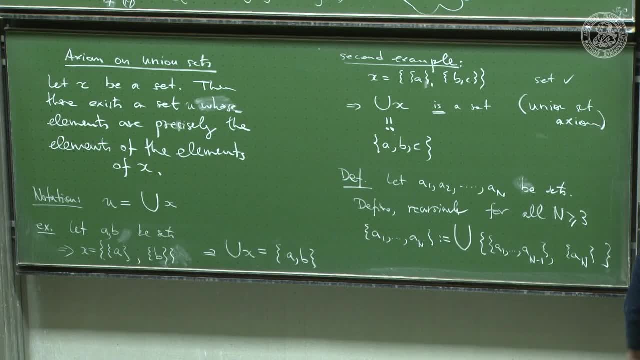 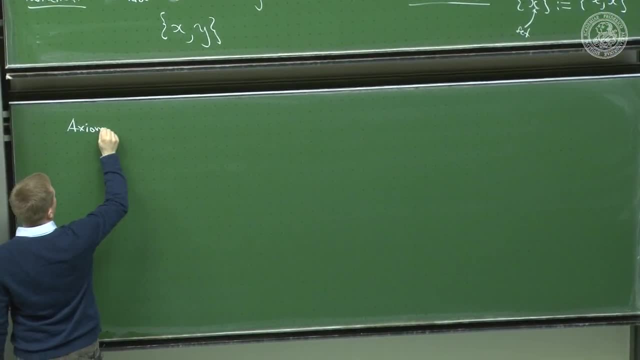 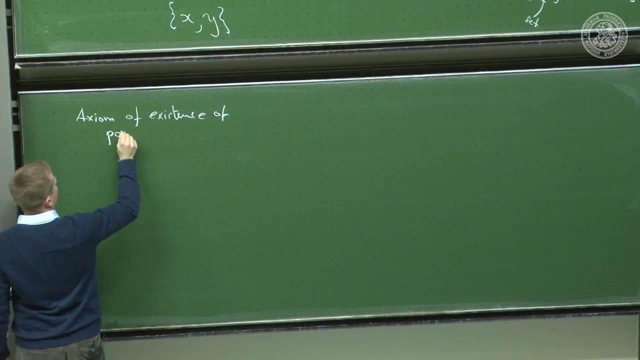 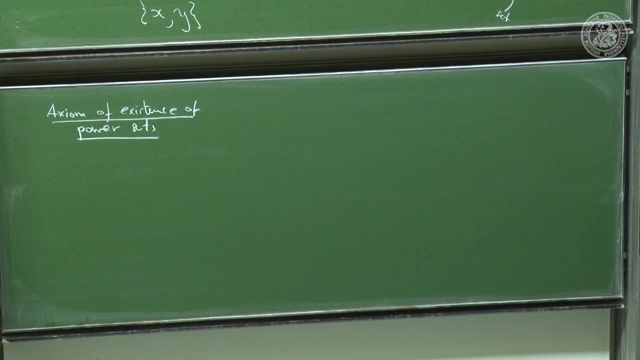 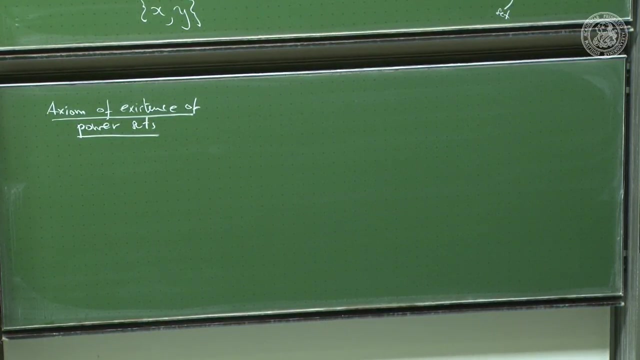 because I would like to first write down the axiom of the power set, simply because the replacement axiom takes a little bit more work. so, axiom of existence of power sets. ah, no, let me take the R first. now I remember why I want that. it's not logically necessary. 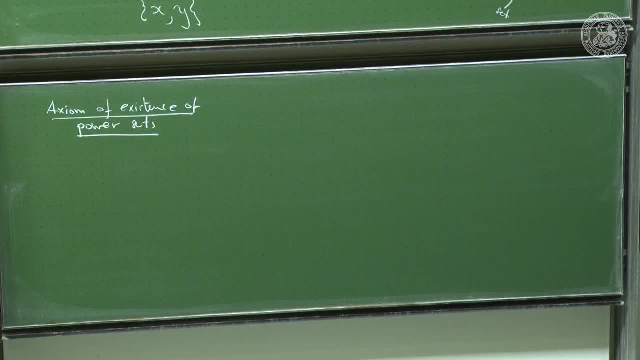 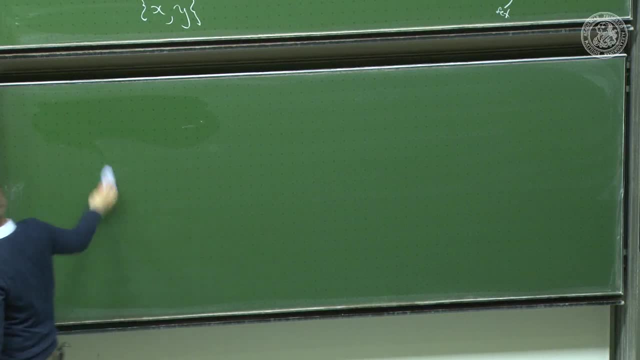 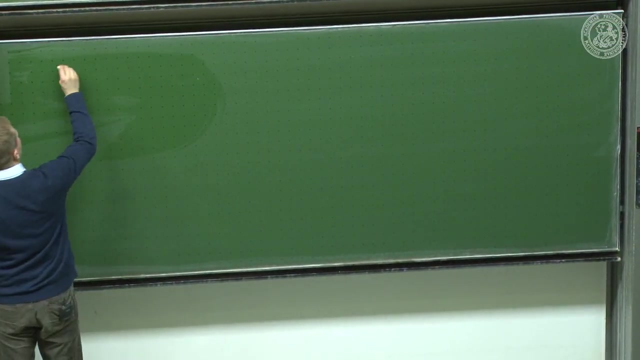 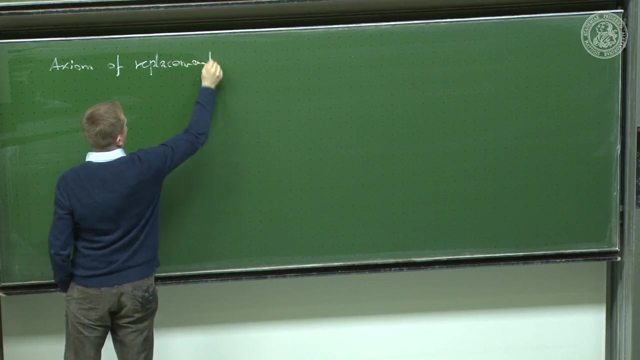 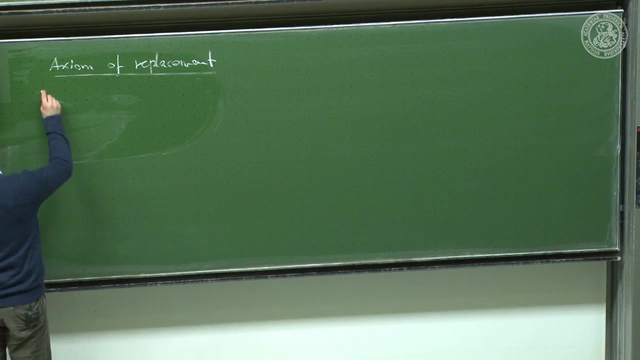 but it's pedagogically better to first take the axiom of replacement- sorry, axiom of replacement, very innocent sounding name- one of the most powerful axioms, and take some work. let R be a so called- and I'll explain this in a second- a functional relation. 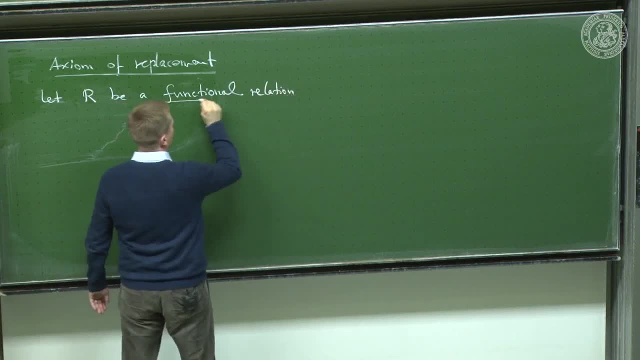 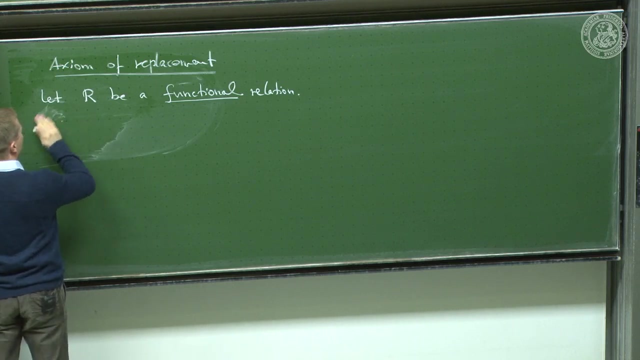 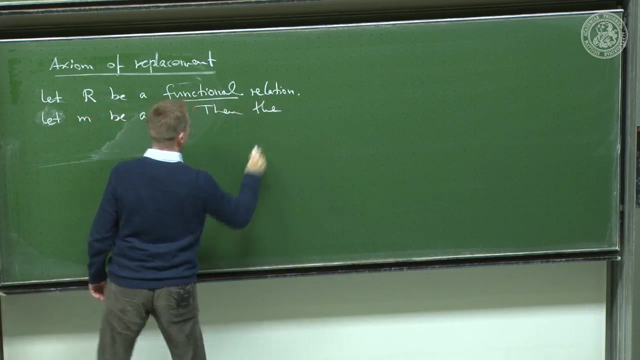 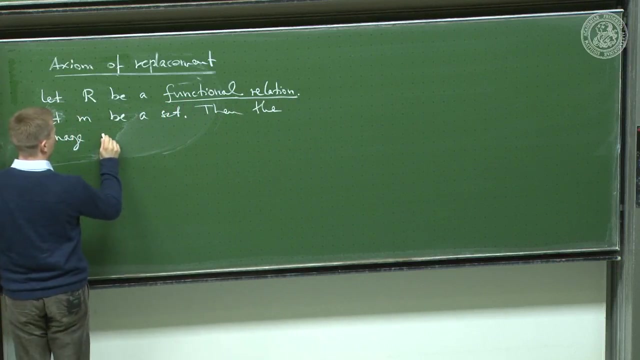 not functional relationship, but functional relation. okay, so we may assume it's existence. let R be a functional relation and let R be a functional relation and let M be a set. then the image- I need to explain these terms in a second. then the image of M, of the. 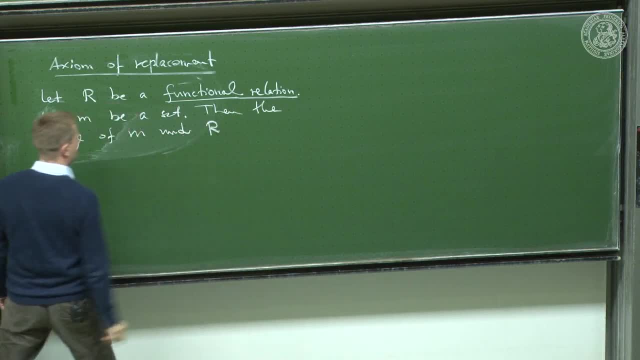 set M under the functional relation. R is the set is again a set. so you see, the axiom is a construction axiom, the axiom guarantees you start with a set M, then you construct the image of M under a functional relation. whatever that is, I'll explain in a second. 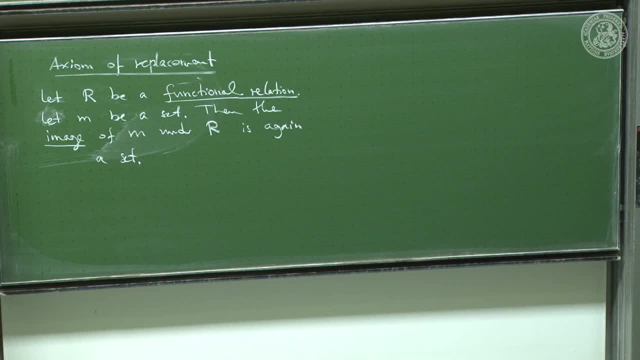 but the result is a set. again, the axiom guarantees the result is a set. now, here you can, or everywhere. we have the following definitions: a relation R, remember, a relation- is a predicate of two variables. relation R is called functional if, for every X, the, there exists precisely. 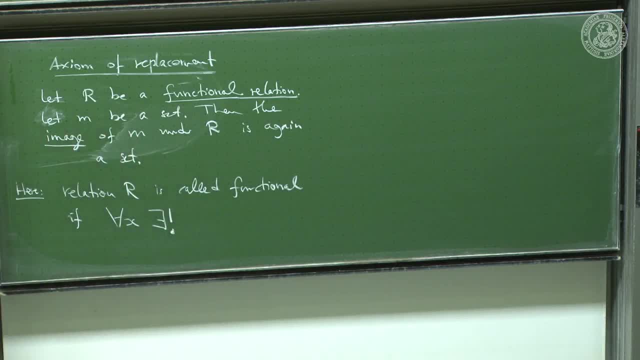 I didn't define this the exists precisely, but you know what it means and you could define it precisely. so, homework- yeah, how would you define homework? so, instead of an examples class, this week, a problem class. I give you these various pieces of homework. define what this means. 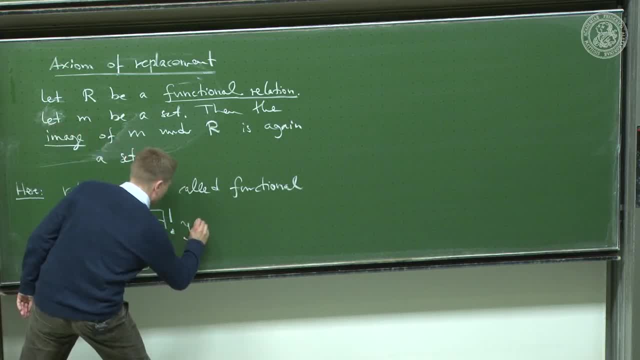 exists precisely one line, such that are of X and Y. that's what you call a function, right? I mean you start with something into every X that is assigned precisely one Y. for another X, maybe another Y, but not necessarily. okay, note that at this stage there is no. 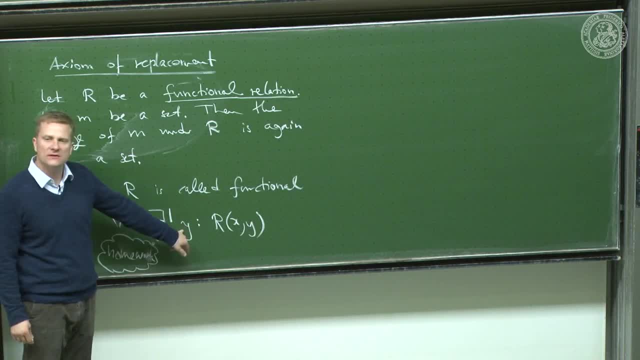 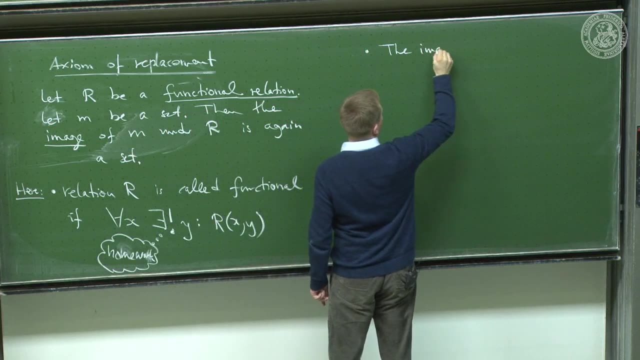 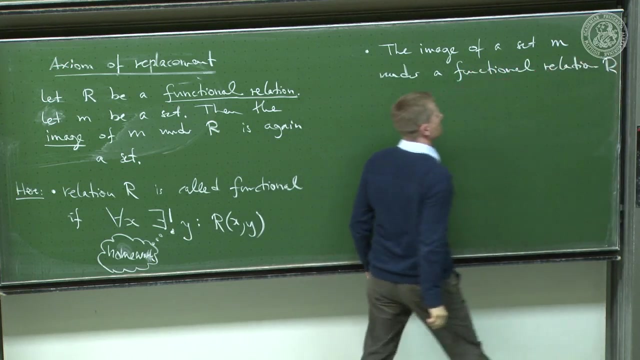 talk about X having to be a set or Y having to be a set. it's just a functional relation, nothing to do with sets. okay, so that's the first definition, and the second definition is the image of a set M under a functional relation: R and the set. 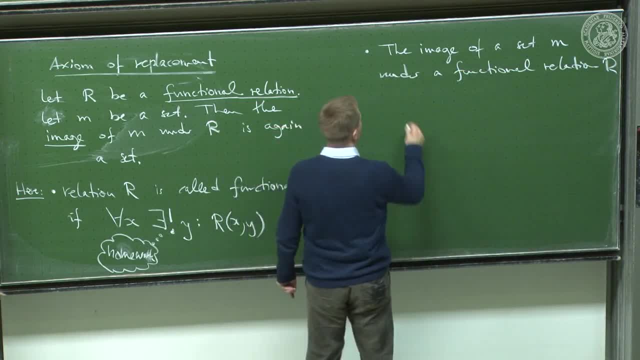 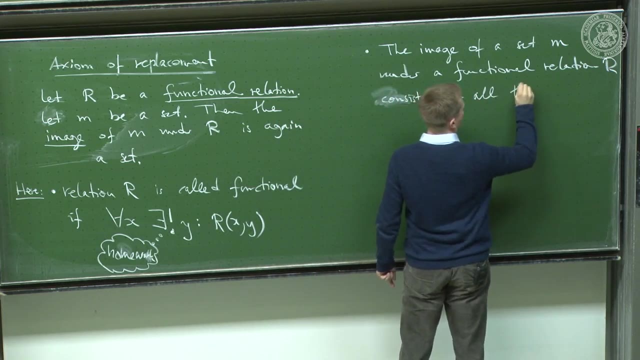 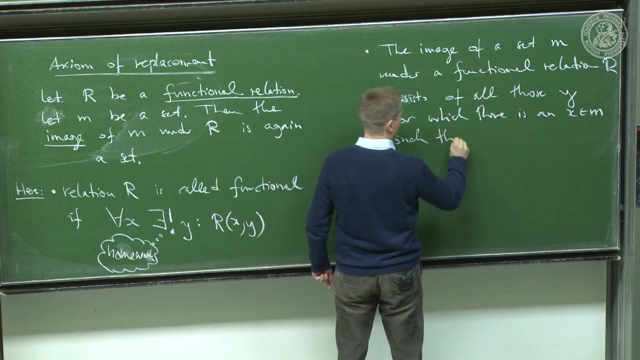 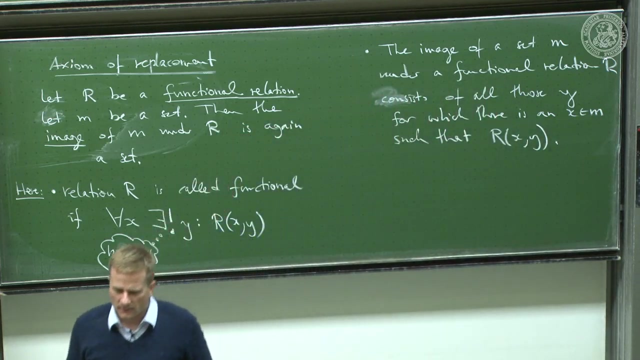 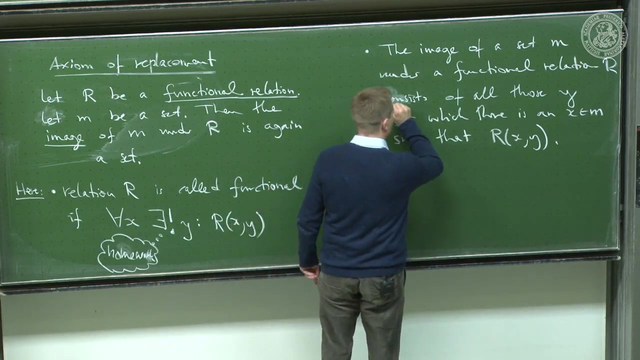 has as its elements or consists. I write consists, and you ask, in a second I'll answer. the thing consists of all those Y for which there is an X in M, such that R X comma Y, and if you're careful, your alarm bell should ring, because I put 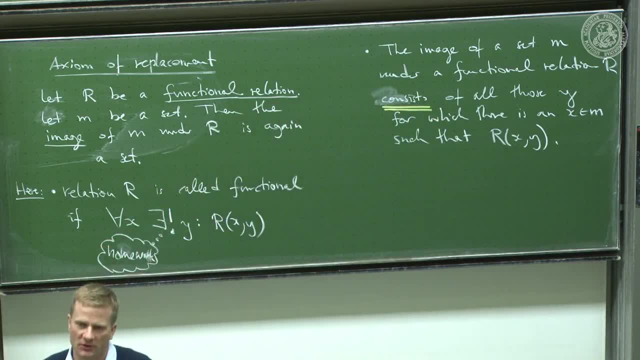 here the word consists, very harmless word, but of course wherever I wrote consists- before I meant consists- of all those Y. I mean has all those Y as elements. the image has all those Y as elements which I read from some X by R, X, Y, right, they say. 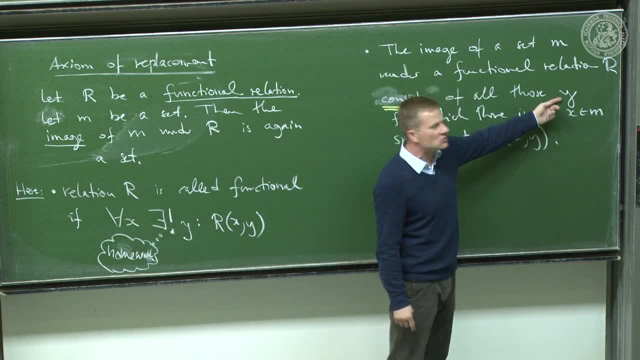 hang on a second. how do you know that all those Y are the elements of something, are the elements of a set? who tells you that all those Y Y's I arrive at constitute a set? again, how would I know? how can I write this down? well, the. 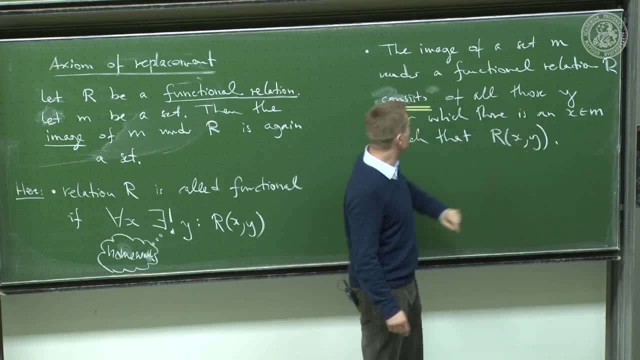 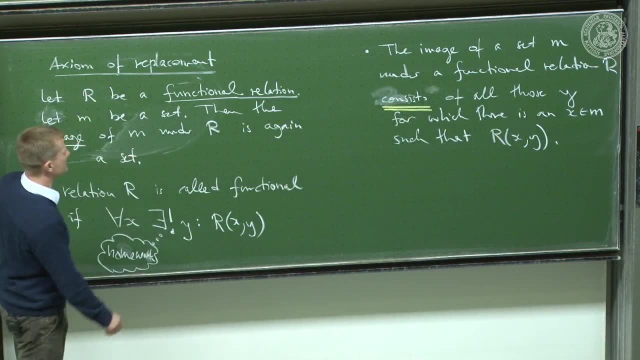 answer is: I write this down. I make no such assumption, but it's in fact the axiom of replacement that guarantees this. the axiom of replacement says then the image is a set is again a set. okay, so that's the logic here. it is guaranteed by postulate. 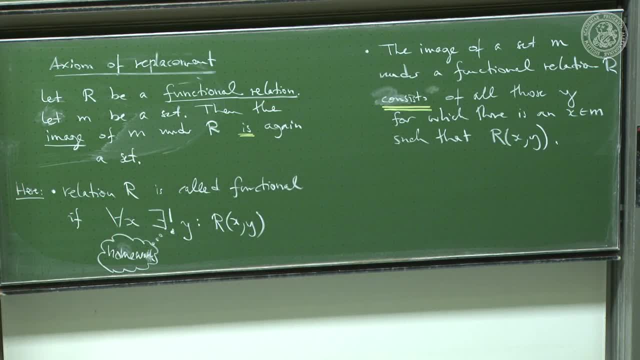 by the axiom of replacement. now, you very likely haven't seen this before, and that's surprising because I said it's one of the most powerful axioms. how come we haven't come across it? well, you have come across this axiom, I think, even in school, in high. 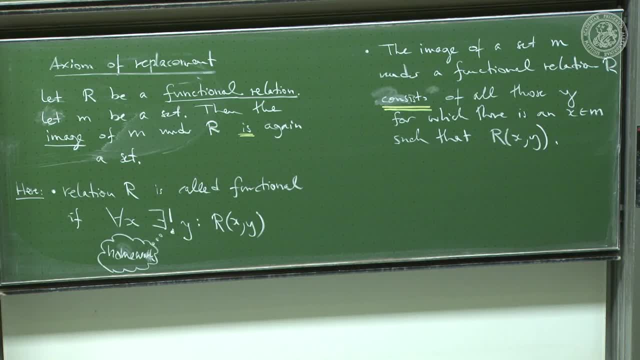 school, but it came in a weaker form and the weaker form is called restricted comprehension, which follows from the axiom of replacement, which I'm going to write down in a second. but the axiom of replacement is slightly stronger and, in order to have all of modern mathematics covered, 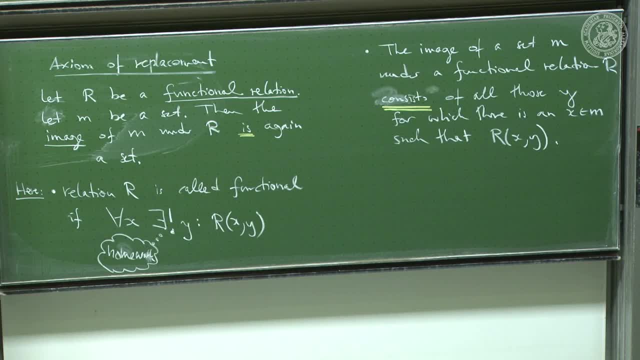 by our set of axioms. we need a slightly stronger axiom of replacement, but in this course we'll actually never again- I think we'll never again- really need to invoke the axiom of replacement, but only its weaker conclusion, namely the principle. let's not call it an. 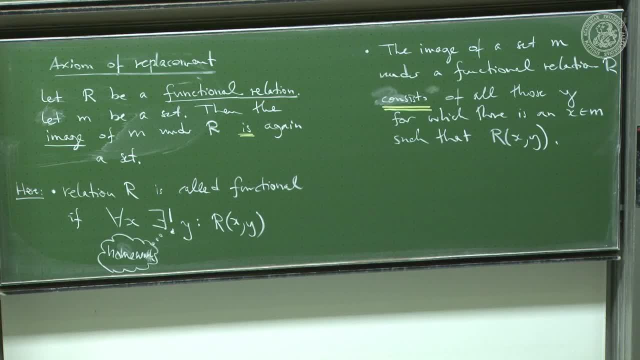 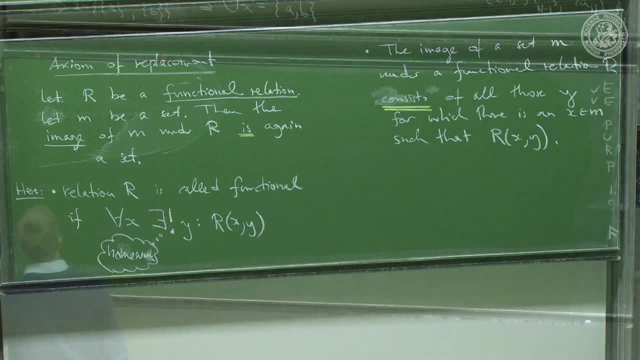 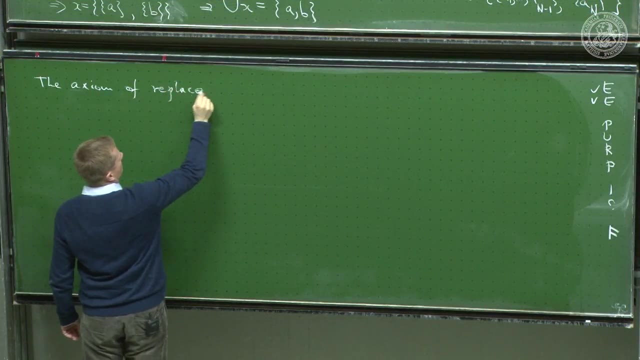 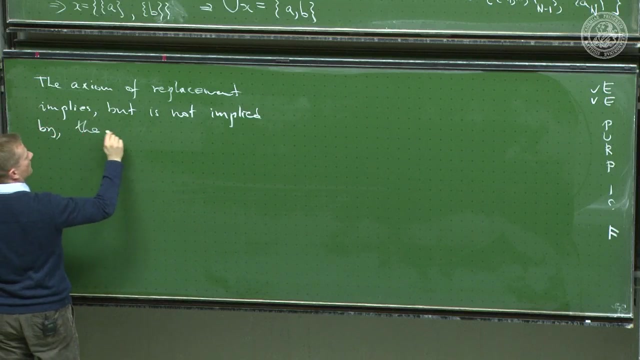 axiom. let's call it a principle, because it's just a derivation from an axiom: the principle of restricted comprehension. I'm going to write this down now and you will recognize it: the axiom of replacement implies, but is not implied by the principle of restricted comprehension, which is: 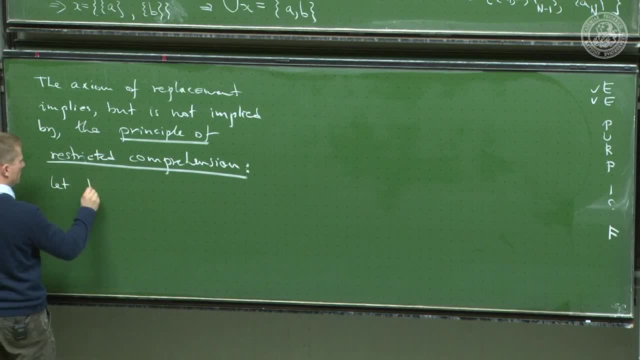 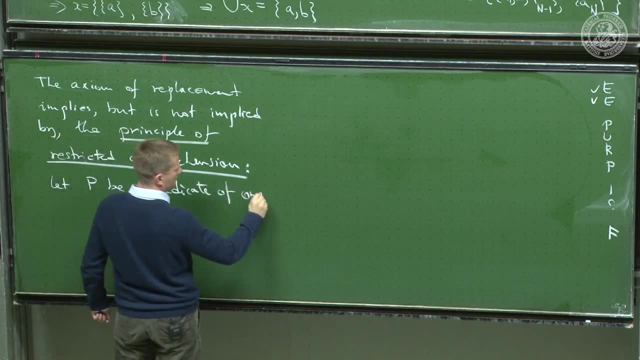 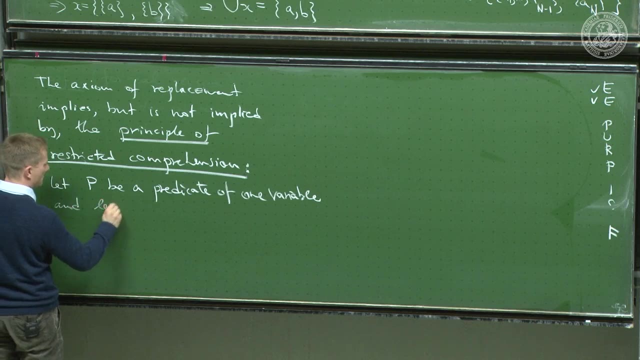 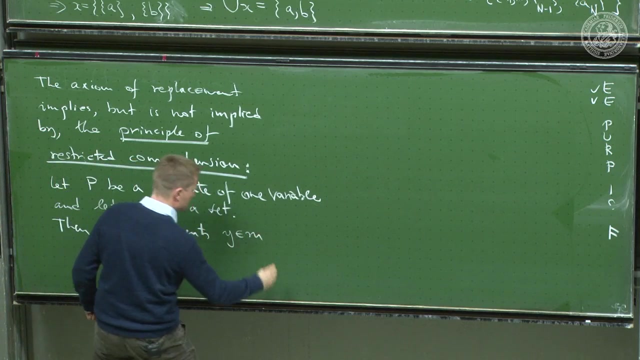 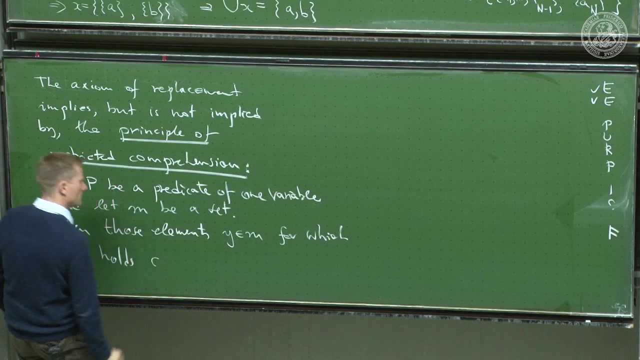 the following: let p be a predicate of one variable and let m be a set. then those elements- y in this previously given set, m, for which p of y is true, holds p of of x, for y, for x p, and then those elements constitute, constitute a set. 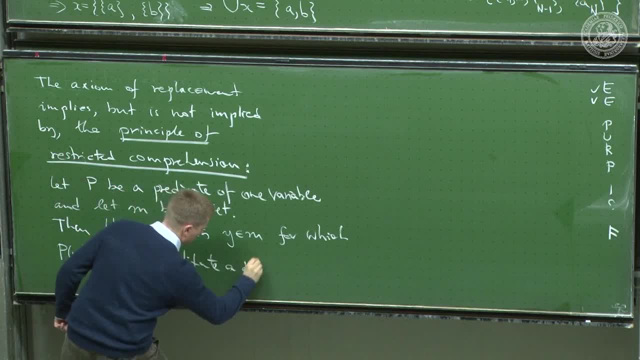 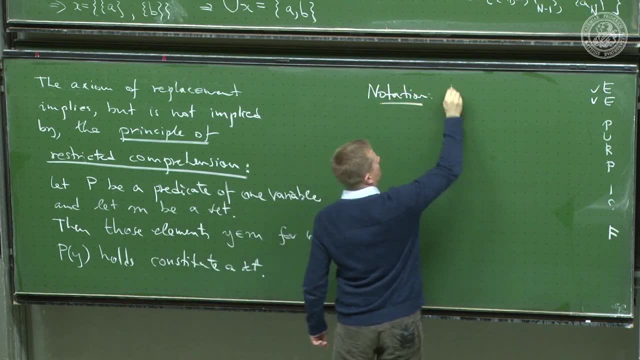 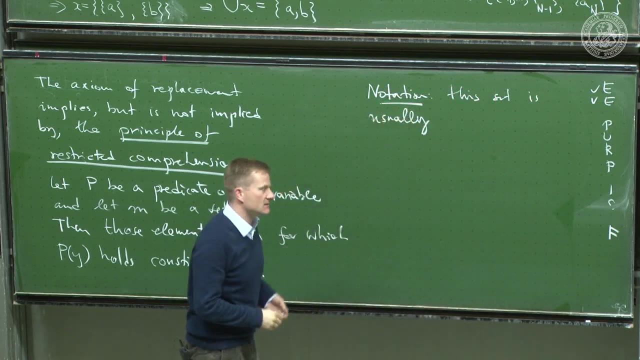 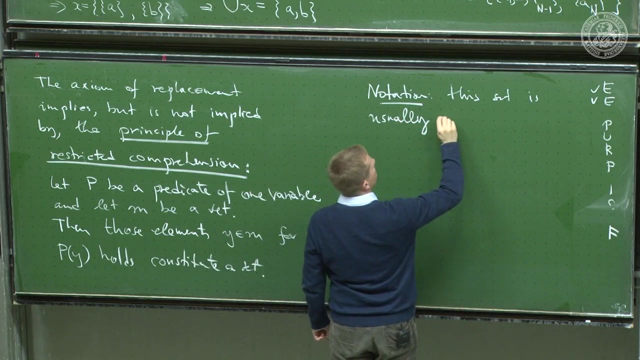 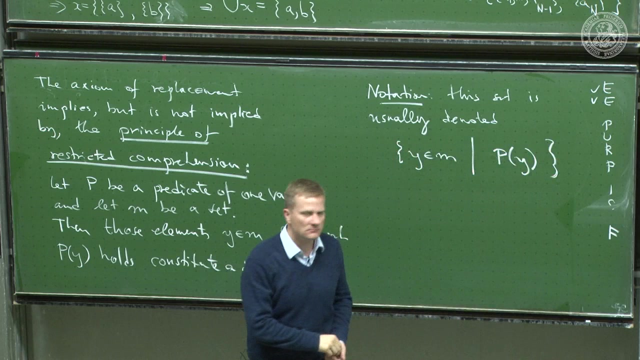 notation: this set is usually denoted, but its existence is guaranteed by the principle of restricted comprehension which follows from the axiom of replacement. usually is usually denoted the set that contains those y in m for which p of y holds- and you saw this before. you do this all the time. 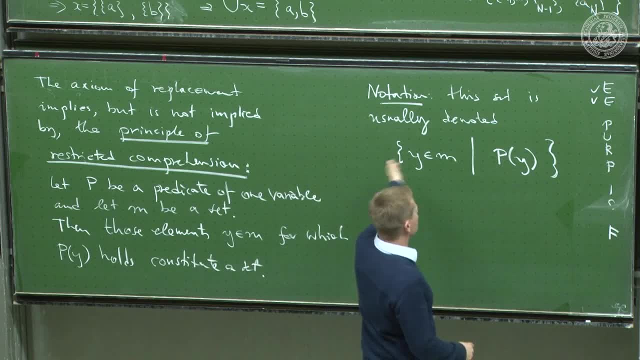 you say: select those elements for which a certain condition applies- standard stuff, and but didn't I tell you just a few minutes ago that this is not consistent? I think we had this on the blackboard, so not to be confused. so the principle of restricted comprehension is not to be confused. 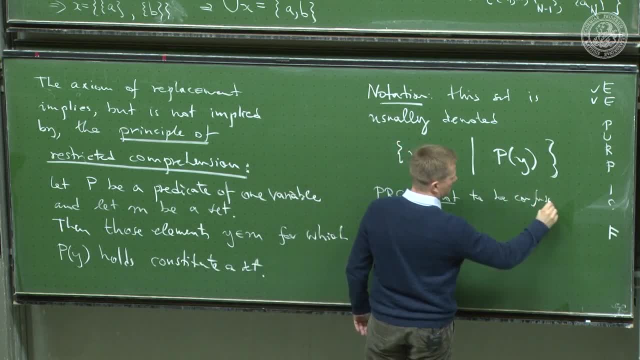 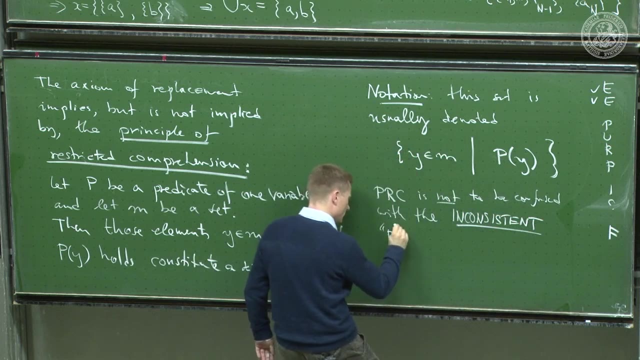 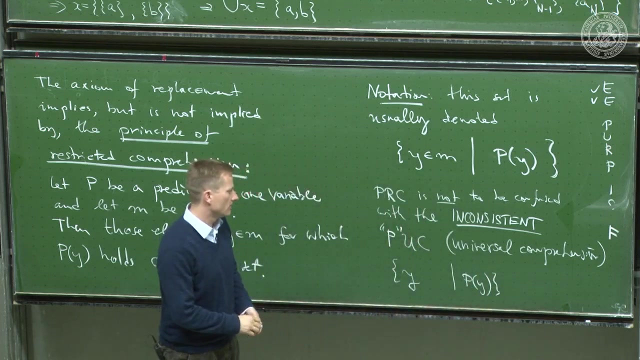 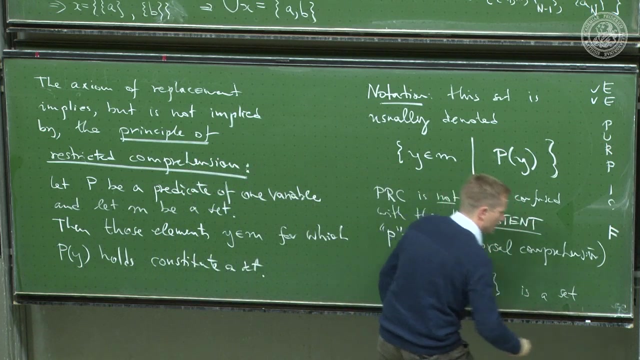 not to be confused with the inconsistent principle of universal comprehension which Mr Russell had his problems with. and this principle of universal comprehension stands and I can say: collect all the y for which p of y applies is a set. well, sick right, it's not a set. this is not true. 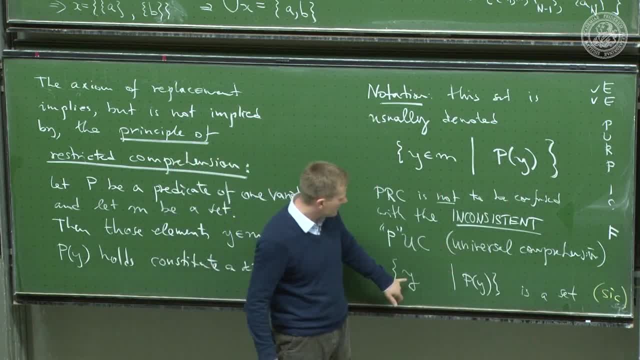 so the principle of universal comprehension says you can collect all the y for which a certain property holds, but this is too much. this could be all the y for which a certain property holds for which y not an element of y. this is the problem. what's the difference? 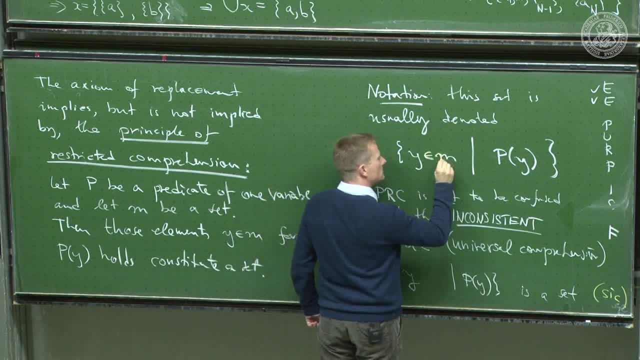 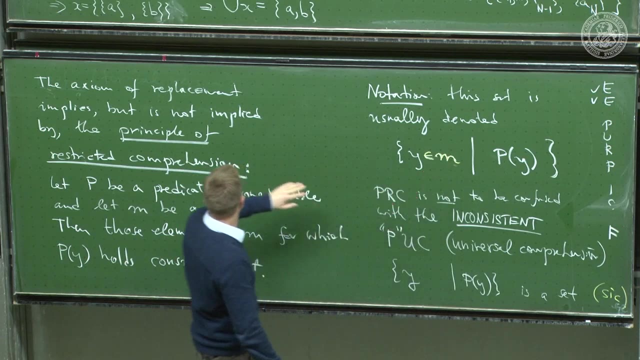 well, the difference is that up here I need to tell from start a set, m, from which I select these elements. so, intuitively speaking, intuitively, if m is already a set, which is what is assumed, and then this thing here can't make it bigger. so I can't make it bigger. 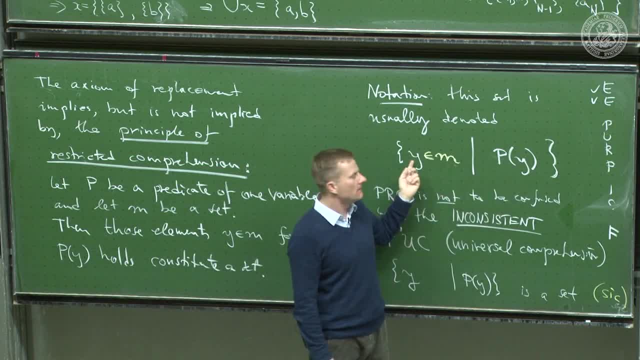 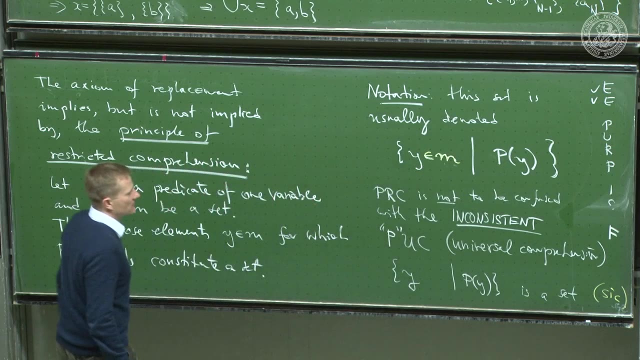 you at most kick out some of the y's that don't make this condition, but the whole thing cannot become bigger and bigger and bigger than m. but because m is already a set, this is not unbounded, this is not unrestricted, it's restricted comprehension. so the restricted in restricted comprehension. 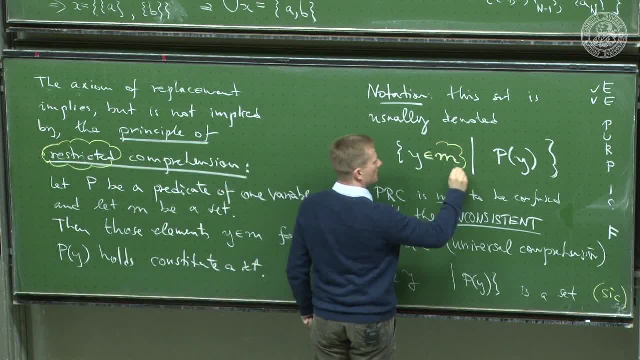 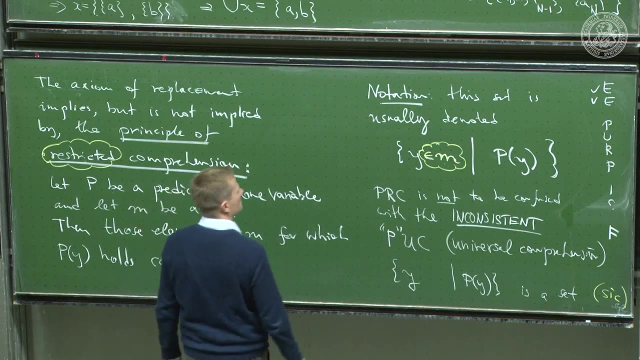 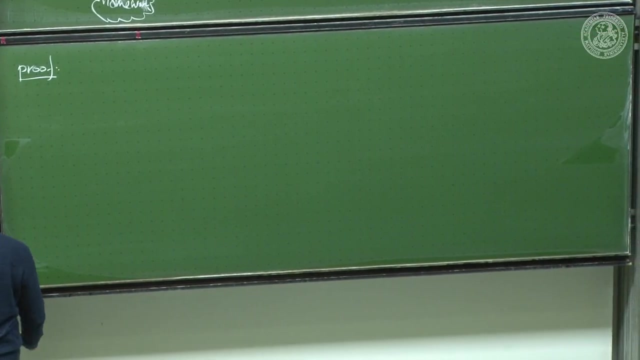 the restricted is this bit. it's restricted to come, the elements are restricted to come from an object that previously has been known to be a set. ok, so this is the principle of restricted comprehension. well, we need to prove it. proof from the axiom of replacement. well, that proceeds. 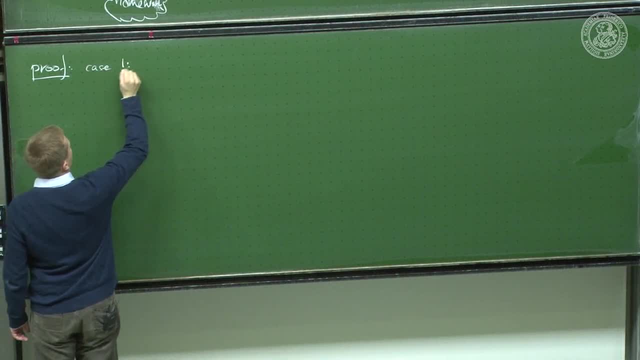 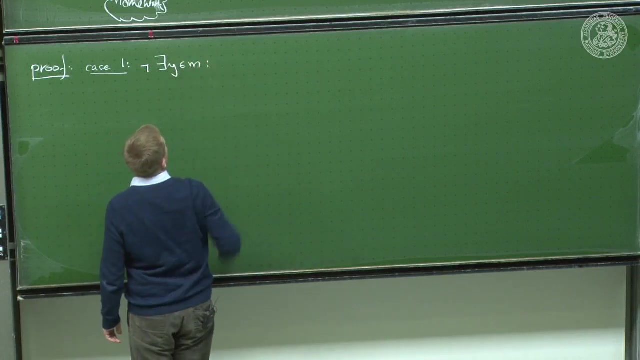 as follows. case one: it could be that there exists. no, there exists no single y in m for which p of y is true. it could be that there is no such. did I define what it means there exists y in m, or only wrote exists y, so anyway. 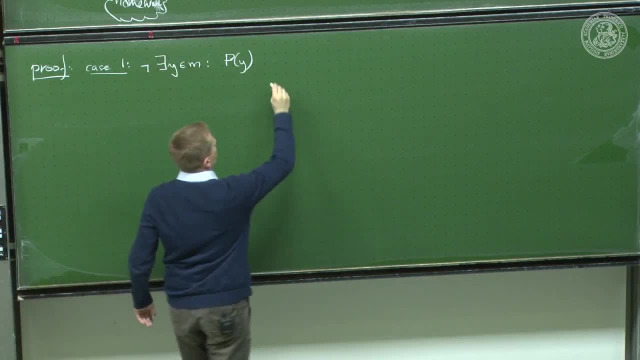 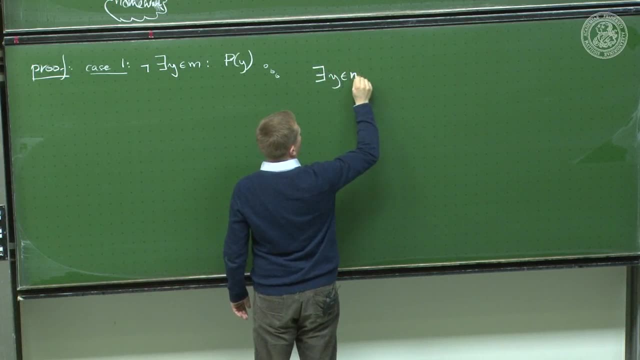 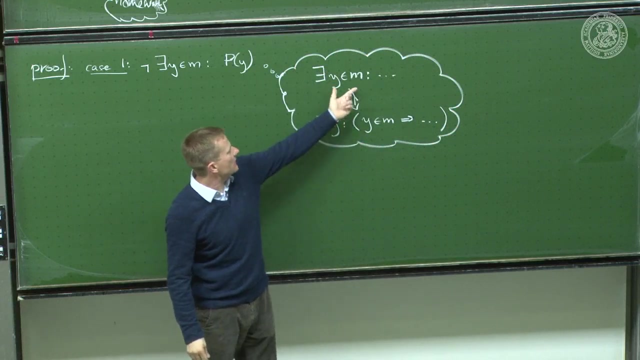 so the idea is: there exists a y in m, such that something this is defined as there exists a y, such that y in m implies the very same something. now I mean first order predicate logic only has this. if I restrict here like this, it's just a short form. 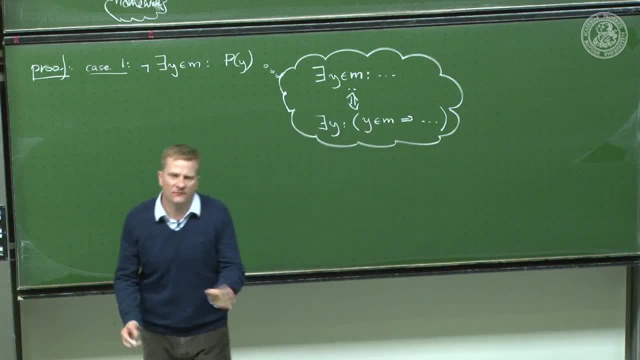 of saying: I condition it on y being in m. very simple, I don't remember what I said. ok, so case one is there is no y such in m, such that this would ever be satisfied. in this case we define. well, I mean, this is just a symbol. 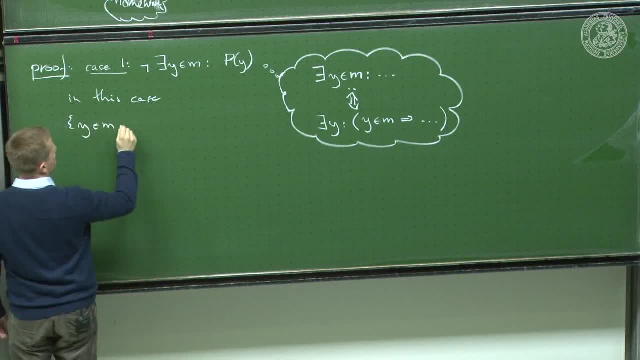 I need to define what the symbol means. and the symbol is a symbol and the symbol is a symbol, and the symbol is a symbol is then defined as the empty set. that's pretty clear. so we don't need the axiom of replacement. it's just our clear statement. 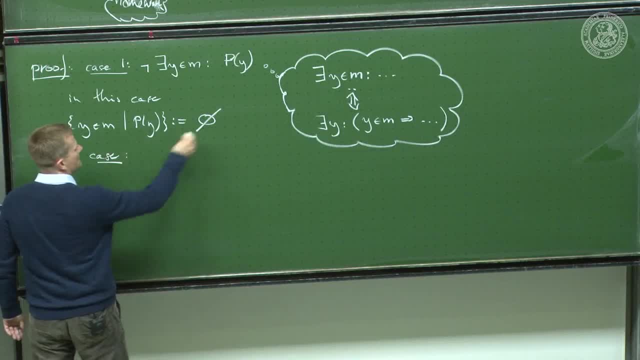 of what this set we are constructing, how it is, and this, the empty set, is a set. so this thing is a set. this is what the principle of restricted comprehension says. but then, in case two, that's obviously the complement of this, there exists a y in m. 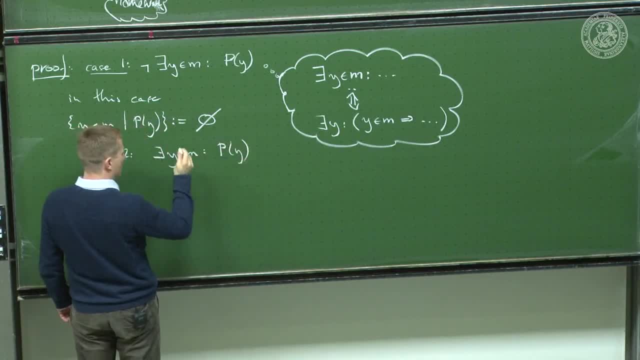 such that p of y and let's call it, let's call this y, let's give it a special name. it's a y hat. there is a particular y hat for which it's true. so there's at least one y for which it's true. take one such. 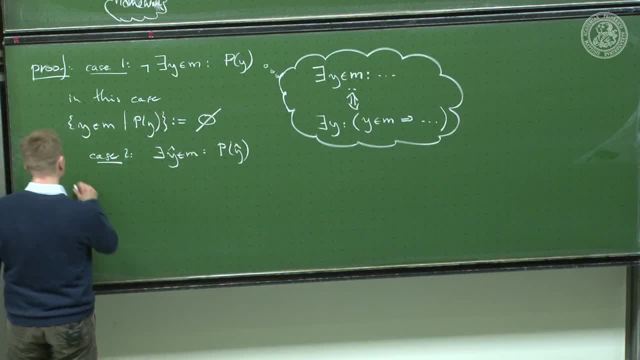 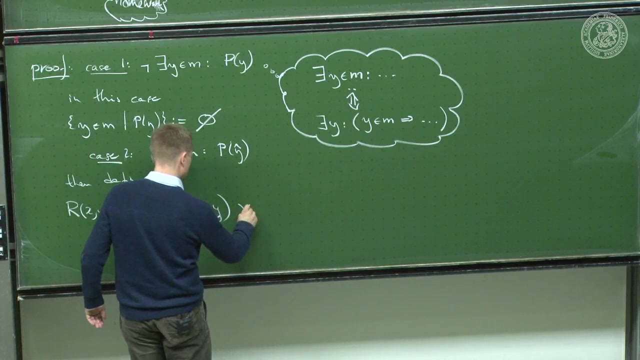 y hat, take it ok and then define. well, if we want to relate to the axiom of replacement, we better construct a functional relation and we define the functional relation x, y, r of x, y as p of x, y, p of x and x equals y or not. 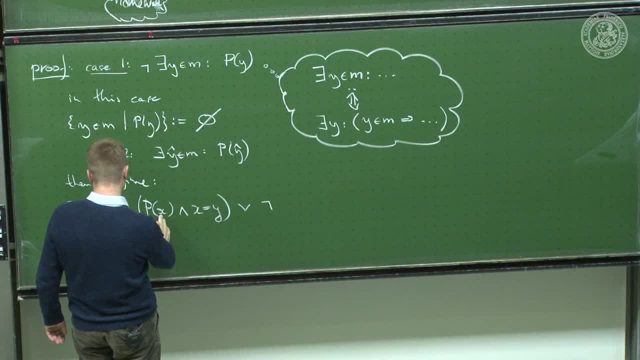 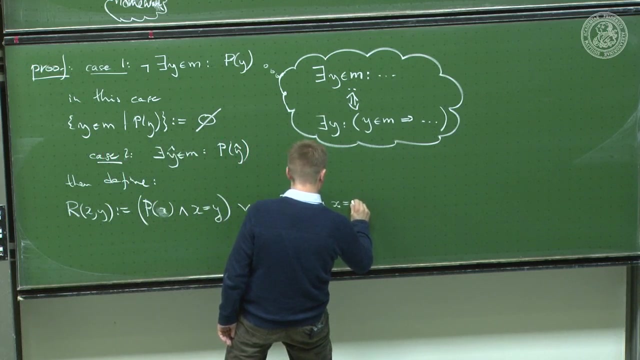 p of x or p of y p hold on, p of hold on. what did I? which way around do I do I do this? um. so no p of x, correct or non p of x, and then um x equals no and then y equals y hat. am I happy? 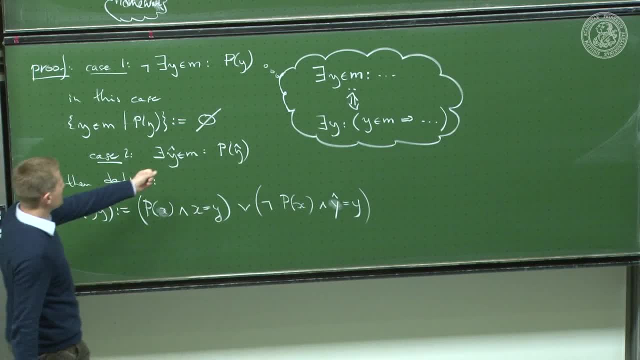 with this. yes, I'm happy with this. so you see, I picked a y hat, a particular y hat, which happens to satisfy the conditions condition. take one of those, a specific one, one of those, and then you find a relation of two variables: x, y, the x and y. 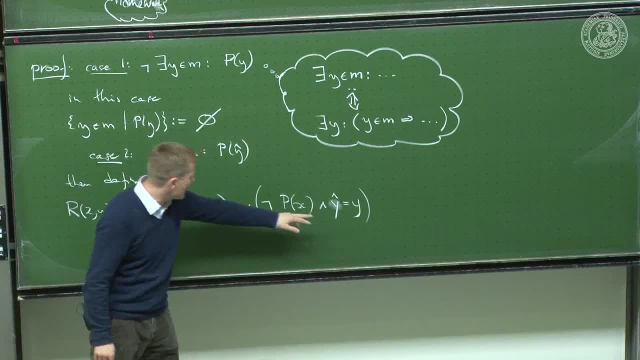 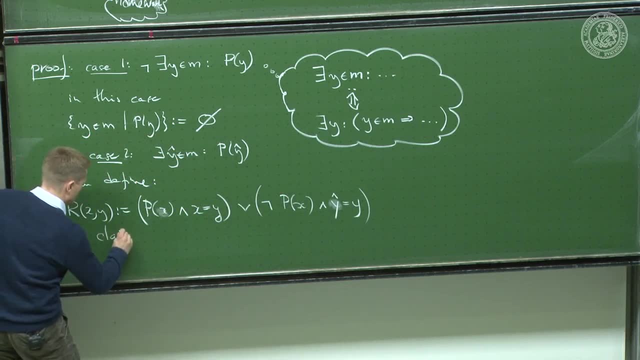 appear on the right hand side, the relation of two variables. there also appears a y hat, but that's a fixed y hat. okay, we, we pick this. and the claim is that this relation is functional. r is actually functional. what's the idea of this function? the idea: 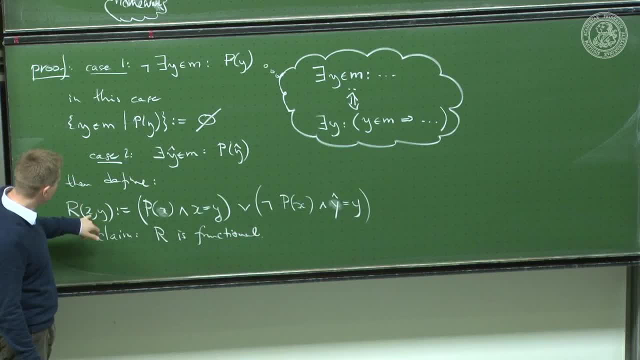 is we want, after all, we want to take all the x in m for which the condition applies. well, if the condition applies, then take just this x as the image y, but if the condition doesn't imply a functional relation requires, it maps to something you every time 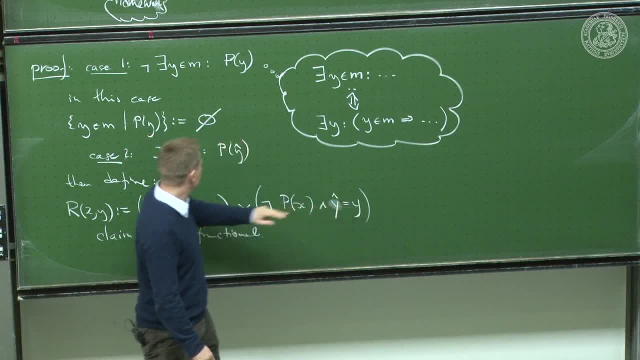 map all those x's where it doesn't apply. you map them to the one y hat where it applies. that's the idea. you need to stare at this at home for five minutes and then you say, ah, so okay, fine, so this is functional. this is the case. 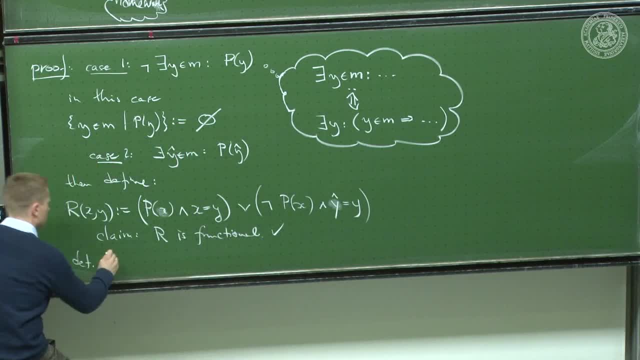 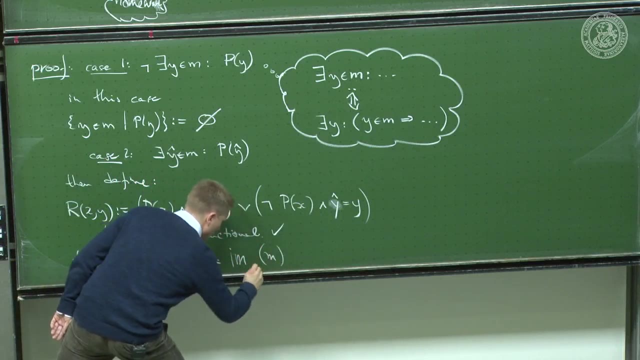 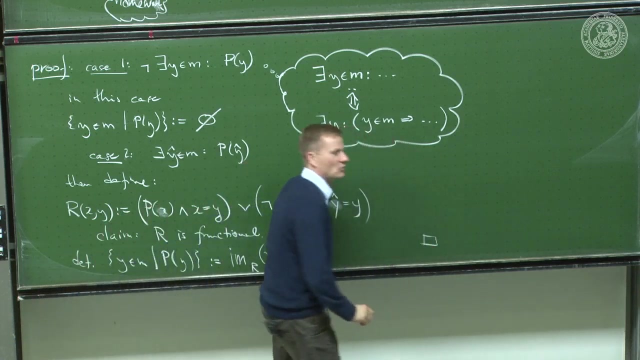 and then we define the set y and m, for which p of y applies. you define it as the image of the set m and under the functional relation r. that's just my notation. I could write out what's written up there. don't worry if you don't. 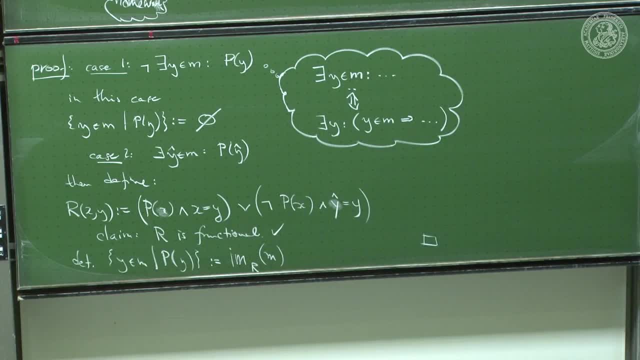 see it immediately. you've got to stare at the definition for a while and then you understand this is absolutely correct, right? so, as I promised, we will rarely invoke the axiom of replacement in full. we only invoke this restricted comprehension and we're very familiar with this. so there's. 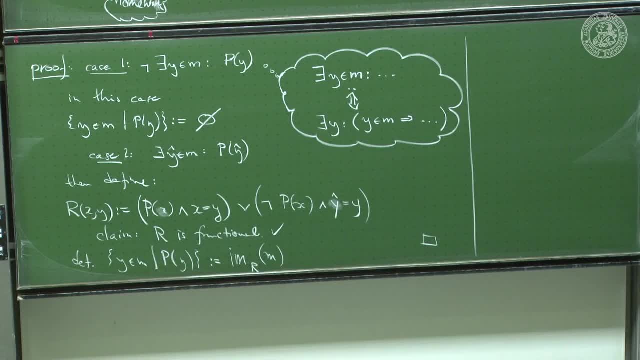 no problem, you just now know where it comes from and obviously there are a number of conclusions you can make. for instance, you can define the complement: let u be a subset of m. they're both sets. yeah then, m without u, what is this? m without u is the. 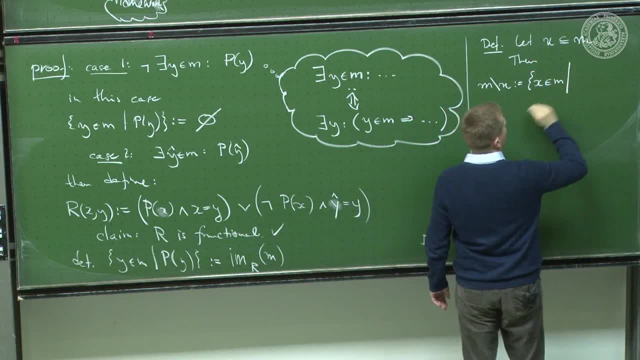 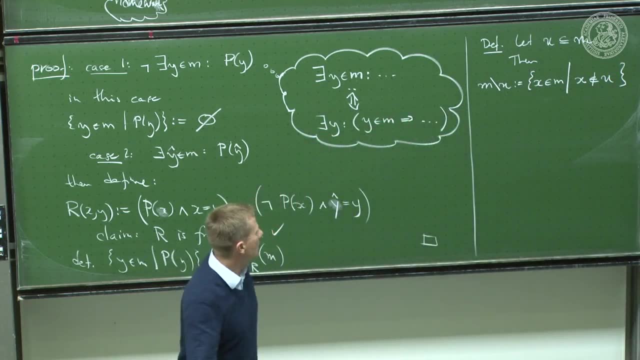 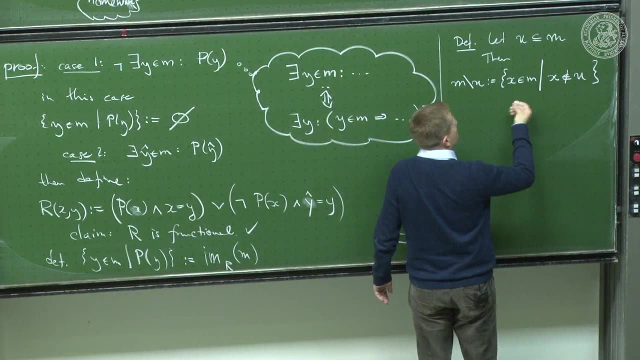 collection of all those elements of m for which x does not lie in u. obviously that's the complement and everything is fine: x in m. this is restricted comprehension. so because of restricted comprehension, we can conclude: is a set. so therefore this is a set due to principle. 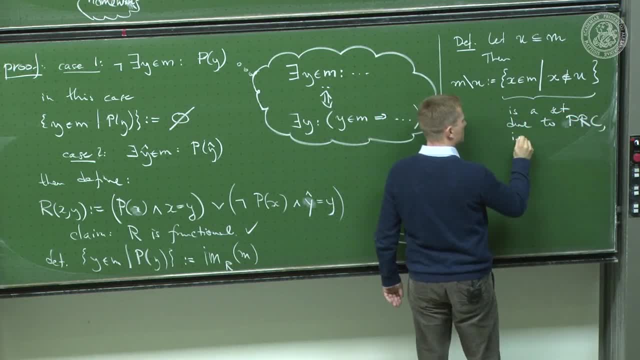 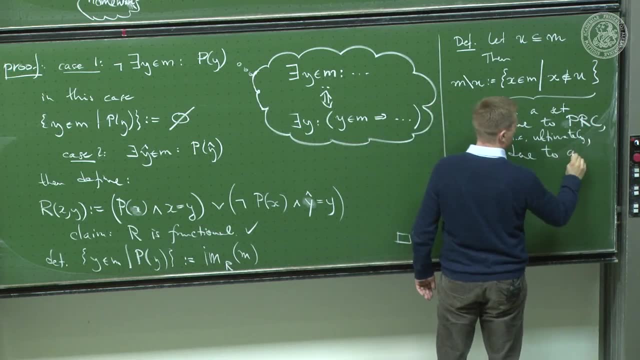 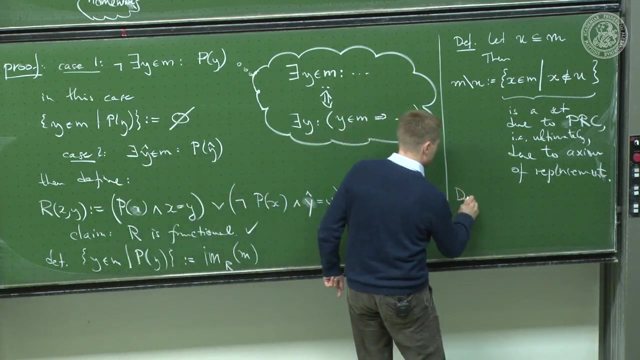 of restricted comprehension that is ultimately ultimately due to axiom of replacement. but you see, this is a little bit more cumbersome to use. this goes more easily. but and then again, as a homework, i leave you with definition of the intersection of sets. so let x be a set. 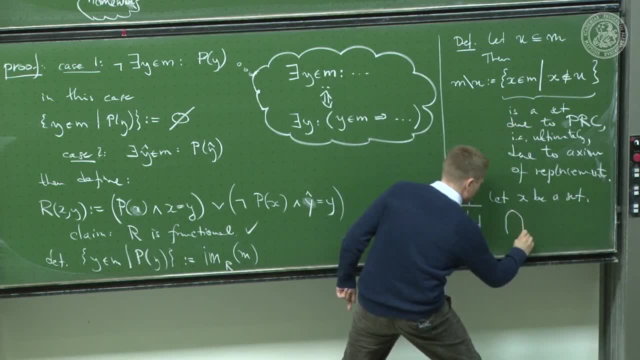 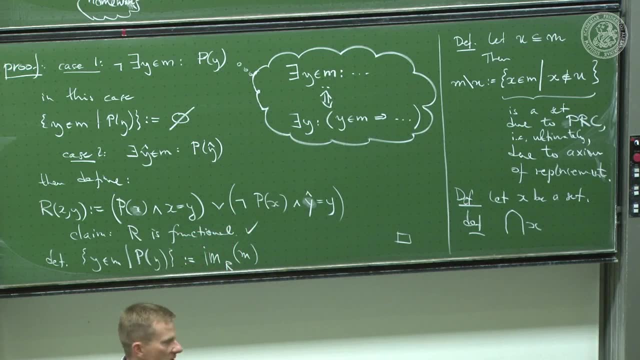 define the intersection of all the x. and i leave it to your imagination of how you do this and i just tell you, use restricted comprehension, okay, so we can do more and more and more. and you see, unions, you got to define them, intersect, you got to postulate. 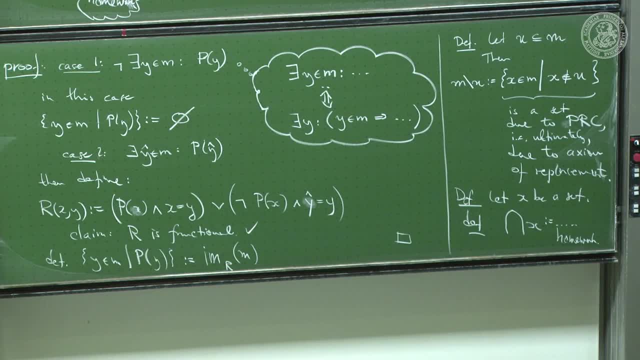 the existence, that this is a set, the intersections you concluded from the axiom of replacement. okay, already made the historical note that the principle of universal comprehension is far too powerful. but you can now see. well, you'll see in the next for the next axiom, why people thought. 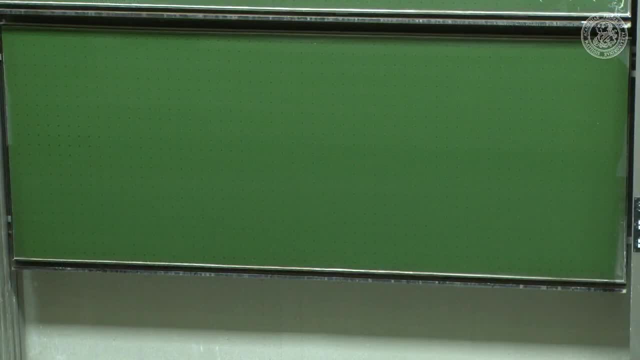 that you need this, but are there any questions so far? yes, where you define the exists y element m in the bottom line. sorry, where. where you define what the involved? yes, where you say exists in the bottom line. yeah, can i not just simply choose any y which is: 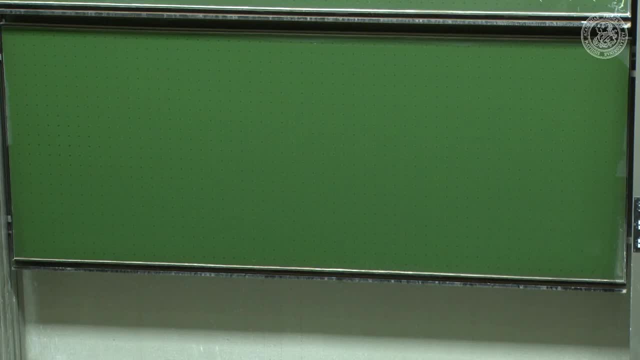 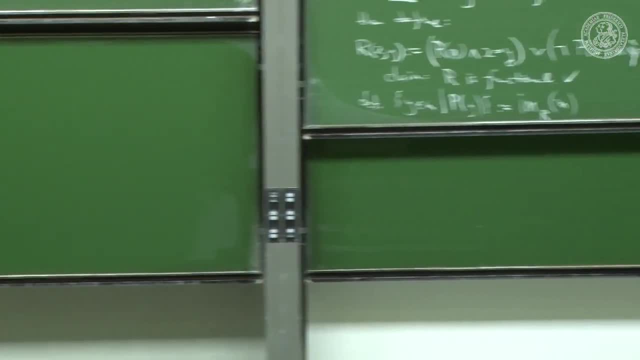 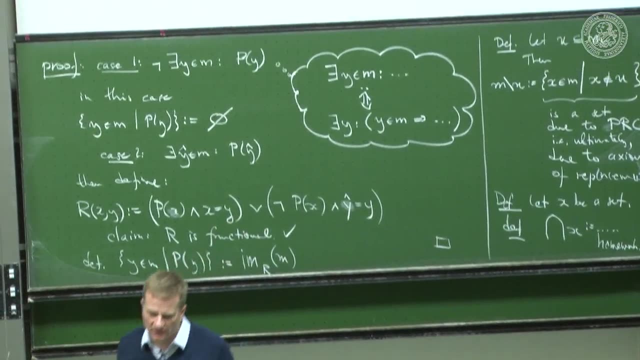 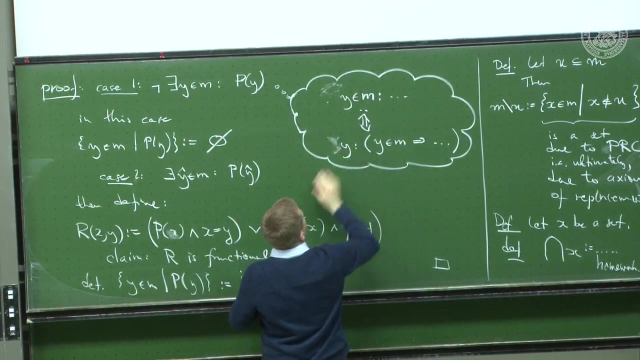 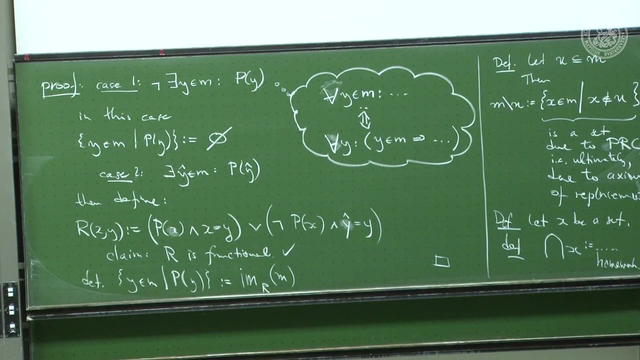 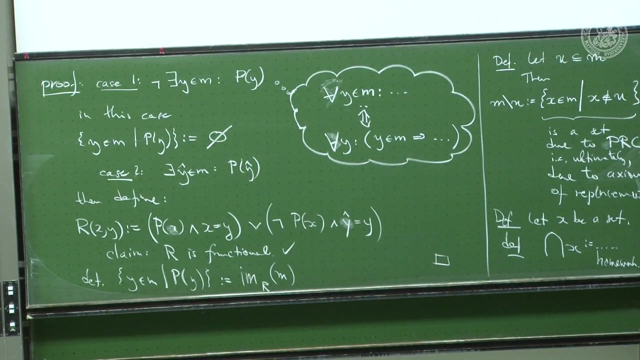 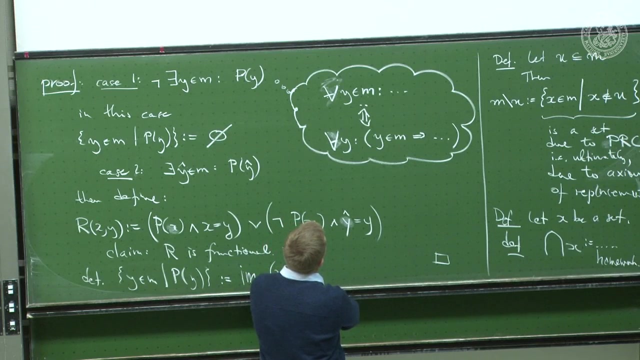 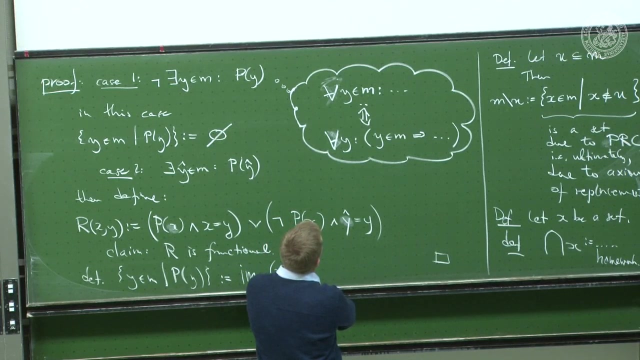 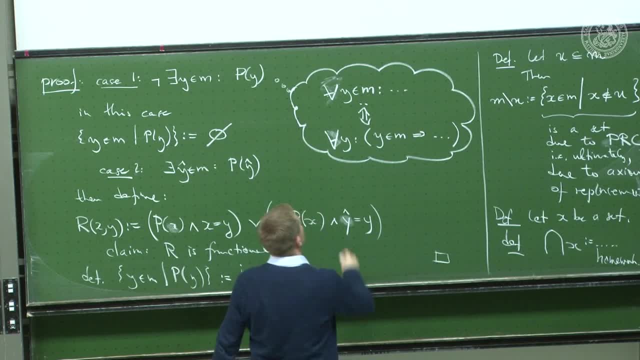 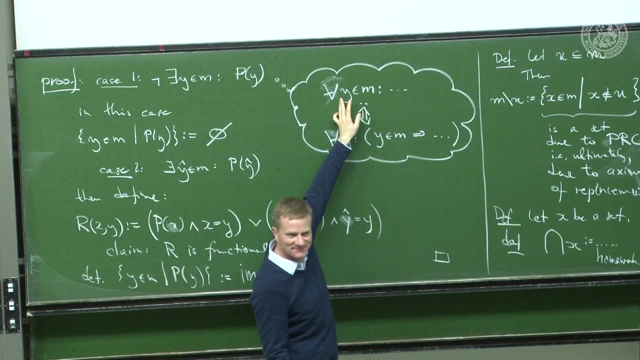 yes, we want it like this, because if i say for all y and m, the following should be true: you could certainly always choose a y that's not in m right, and then anything i write here would always be false. we want, if the y doesn't come. 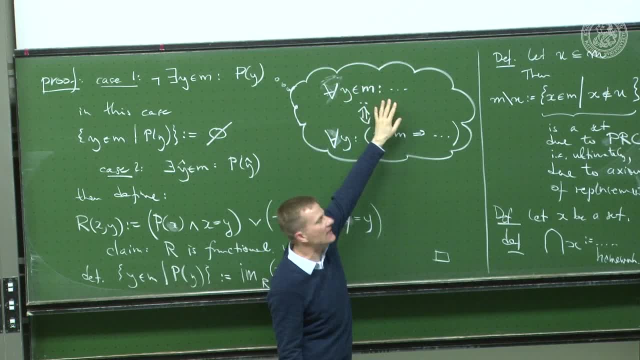 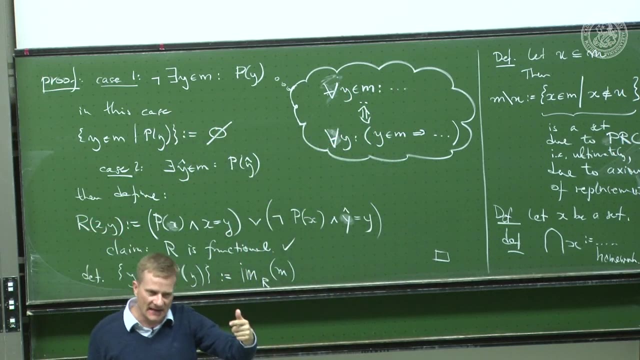 from m, not to affect the validity of this statement, which then only hinges on the condition being true for the y and m being true. okay, i'm confident that for the all quantor it's correct, and then this existence quantor is defined as before it's. 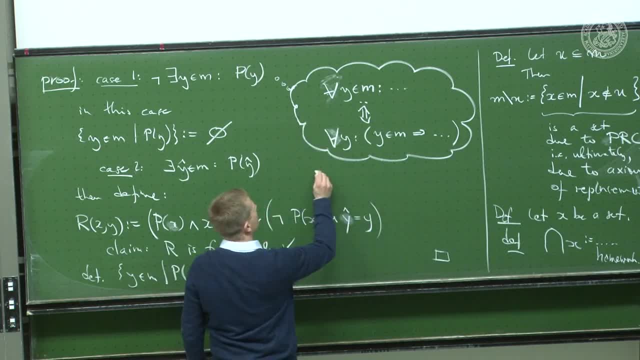 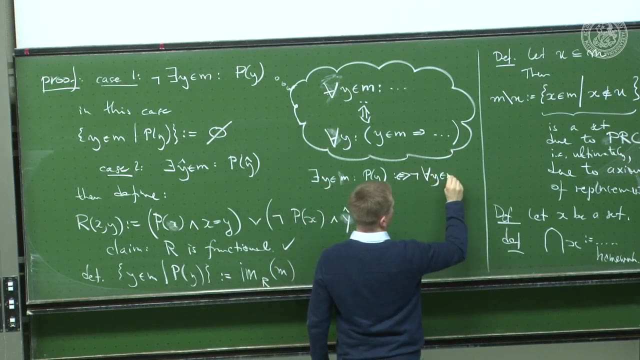 derived from this definition of the all quantor, then the existence quantor there exists a y in m, such that a certain condition p y holds, will then be defined as not for all y in m. is it true that this does not hold? yes, yes, and this: 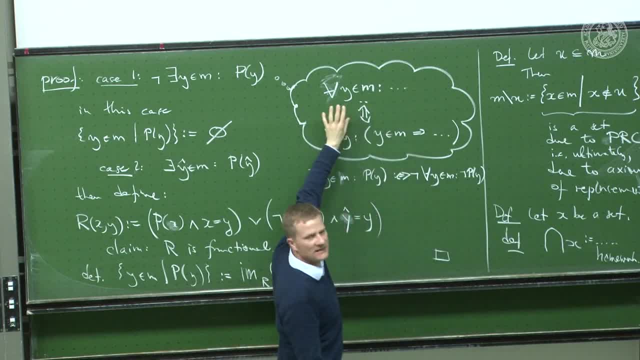 double, double, not doesn't pull into here the way i suggested. very good observation. thank you very much. that's very important. you define for the all quantor like this. that's exactly what we want, if you think about it, and then this is related to this in: 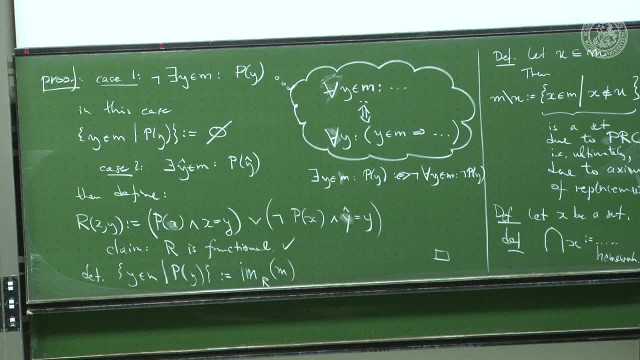 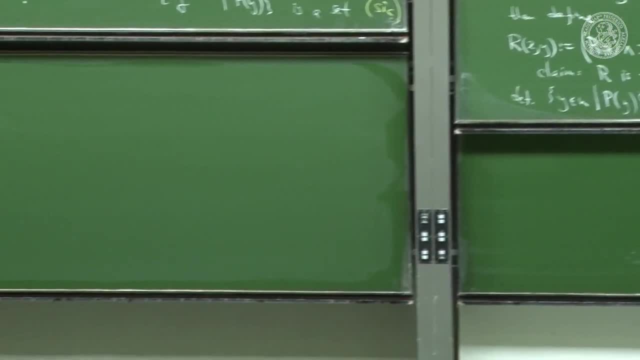 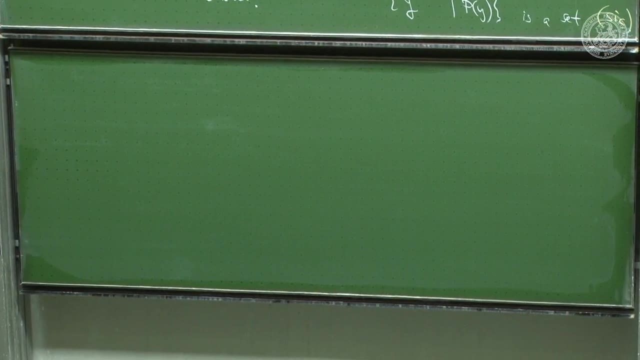 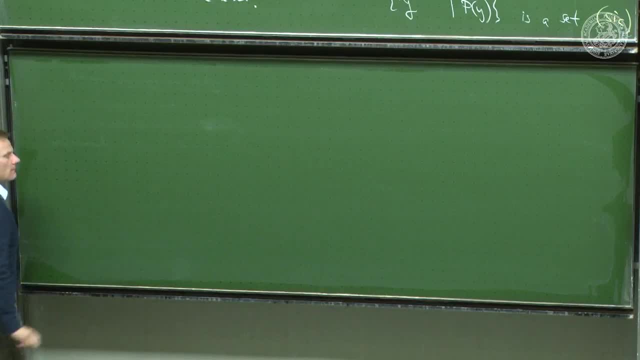 axiom on power sets, and we all know what a power set is. the power set is the collection of all subsets of a set right. so traditionally- no, historically, I should say historically- in naive set theory, the principle of universal comprehension was thought to be needed in order to 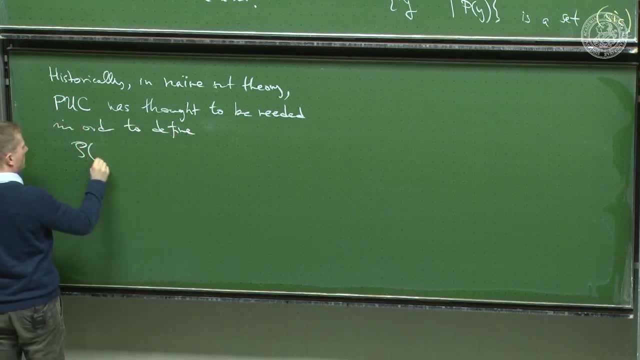 define for any set m, for any set m, this object, curly p of m, called the power set and traditionally and, I remark, inconsistently well, by using the principle of universal comprehension, which is not a good principle, it's a bad principle, it's inconsistent to say those are. 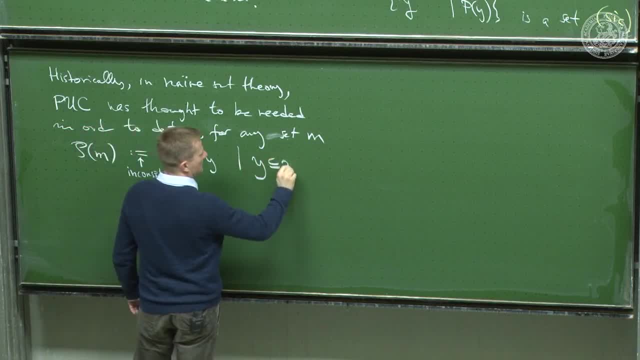 all the y's that are subsets of m. we collect all the subsets of m but we cannot tell which bigger set these subsets come from if we're only given the set m. so to an extent, what you want to do in set theory it's a very deep 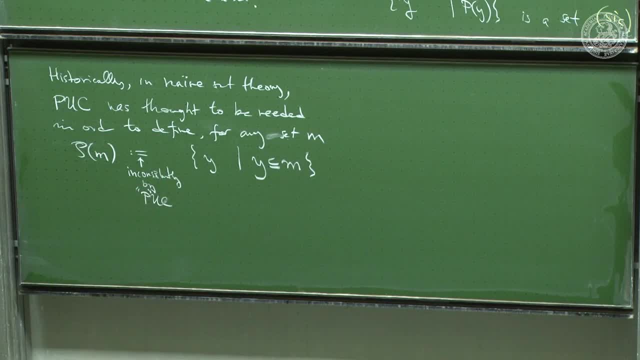 thing in set theory is you want to repeatedly apply power sets. you take the power set of the power set, of the power set, some other sets- we'll come back to this- and this way you go through the entire universe of sets. if you wish, you can generate. 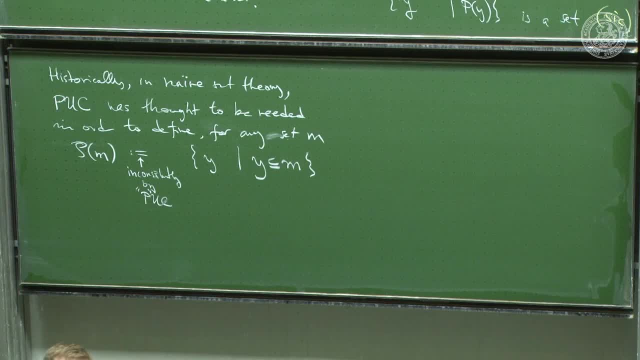 every set in set theory, roughly speaking, by repeated application of taking the power set, of the power set and so on. so but if you want to generate sets, it cannot be that you know before where they come from which big set. so people thought you need this principle. 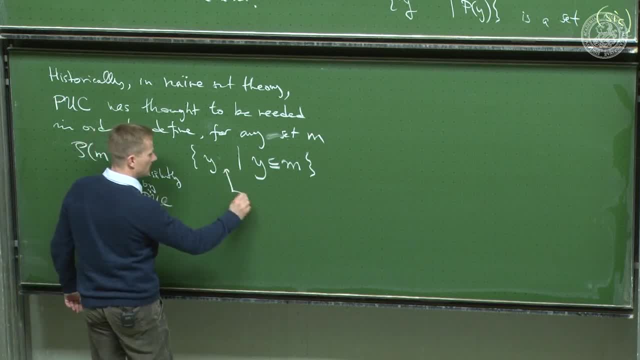 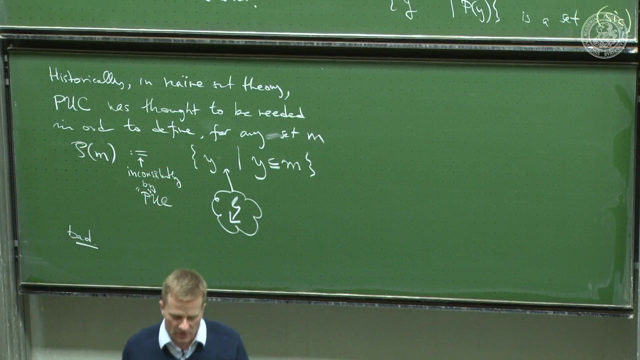 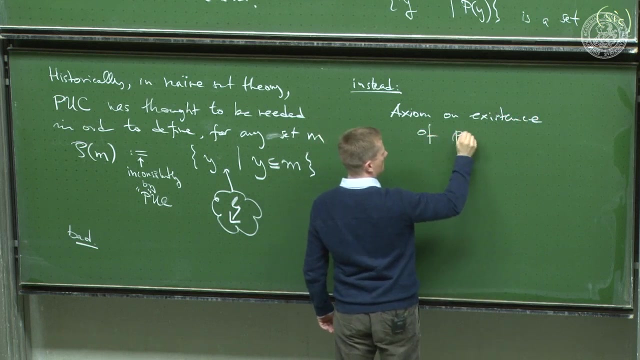 of universal comprehension. but we of course here we lack the restriction, so we know we're not going to do it this way. bad, and in fact there is no other choice but to postulate that the power set exists instead. axiom on existence of power sets. let m 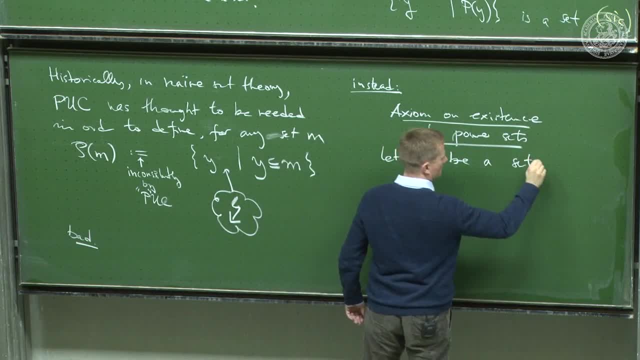 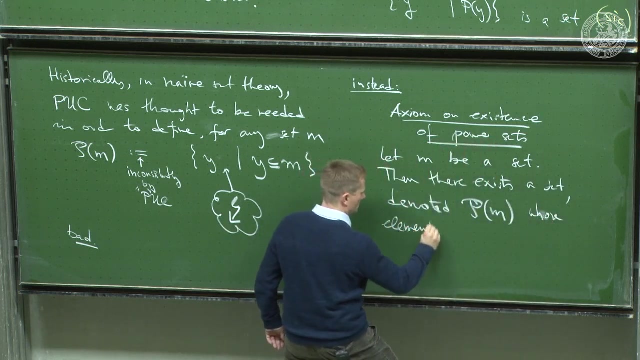 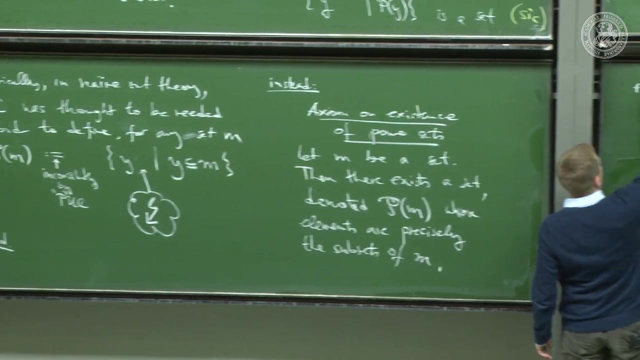 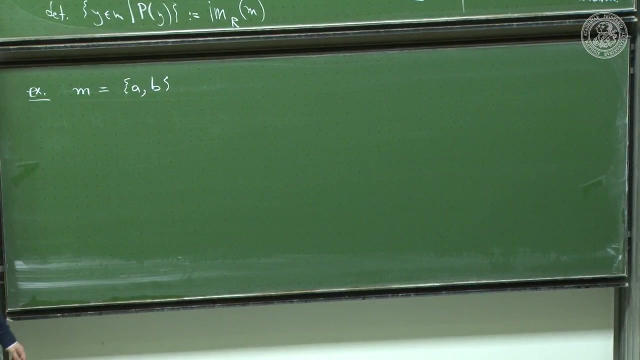 be a set. then there exists a set, denoted curly p of m, whose elements are precisely the subsets of m and the T of m, which is the collection of all subsets. well, the empty set is a subset of any set. then there come the one element subsets. 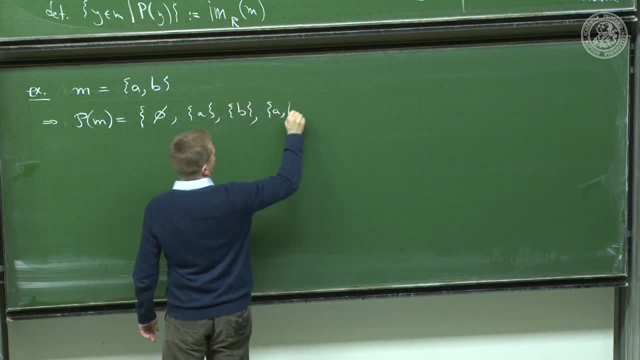 of m and then here it's already the entire set. so these are all the subsets of m and they're all collected, if you wish, in the power set of m, and that's, of course, the standard issue power set. that you know, and it's so easy. 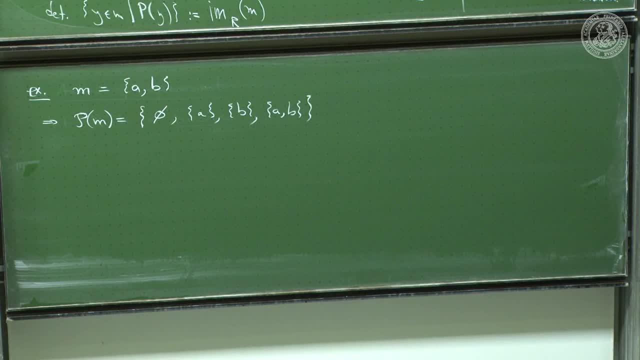 to explain how to build it. you take all those things and collect them into a set, but is the result a set? we cannot argue so by the non-existent principle of universal comprehension, because that's not a principle. we don't want that. we cannot argue so by the 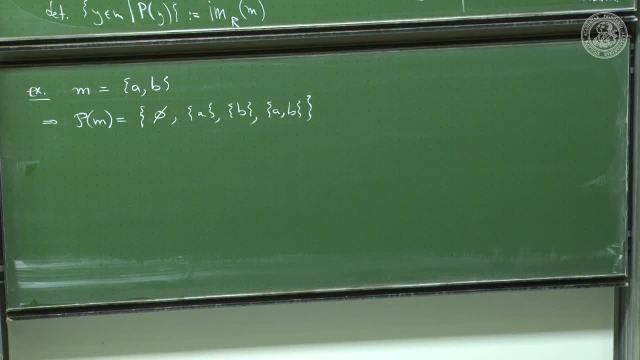 principle of restricted comprehension, because we wouldn't know a priori from which set the subsets come from which bigger set, because that's just a set we want to define. this way, there's no other choice but to have to dedicate an extra axiom to the existence of power. 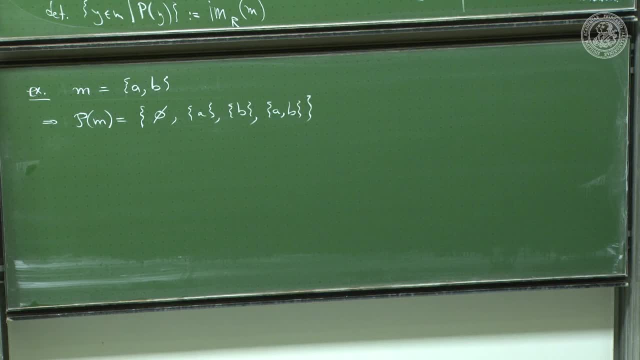 sets. that seems not very economical. I mean, what on earth else we will come up with that we want and put down an axiom, right well, the power sets we want. so we have ee, perp, icf. let me go to the i and then I'll. we'll continue. 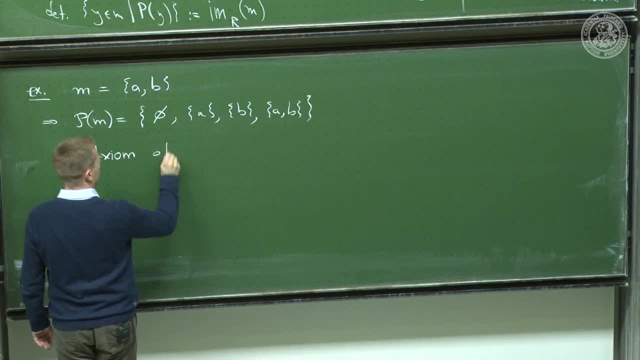 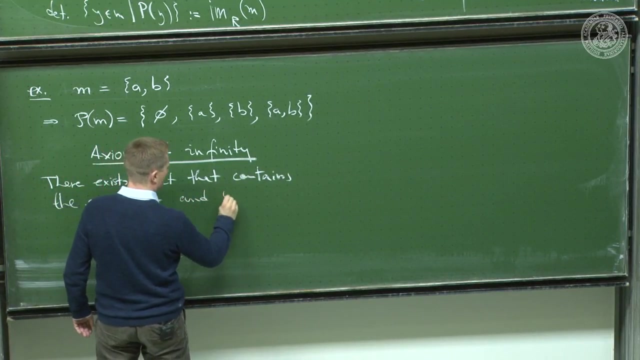 with the rest. next time it's the axiom of infinity. the axiom of infinity is something we also want, because otherwise we don't get standard mathematics. the axiom of infinity says there exists a set that contains the empty set. okay, that's simple enough. and with every of its 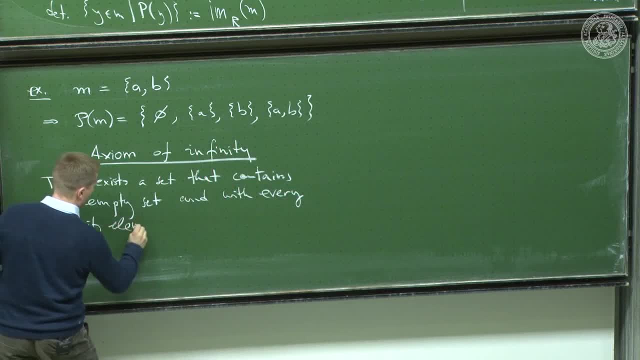 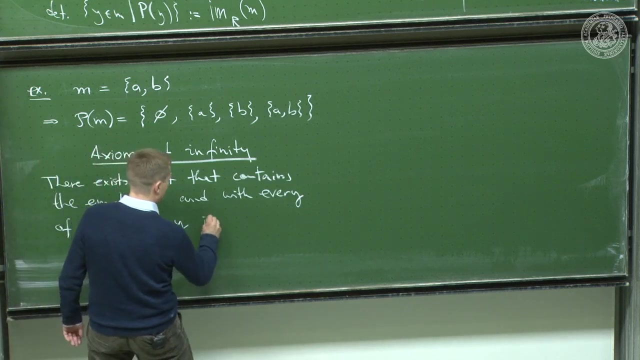 elements. y. well, this, of course, does not refer to the elements of the empty set, because there are none. these exist, to the elements of the set whose existence is postulated with every of its elements. y it also contains. contains always means contains, as an element contains the. 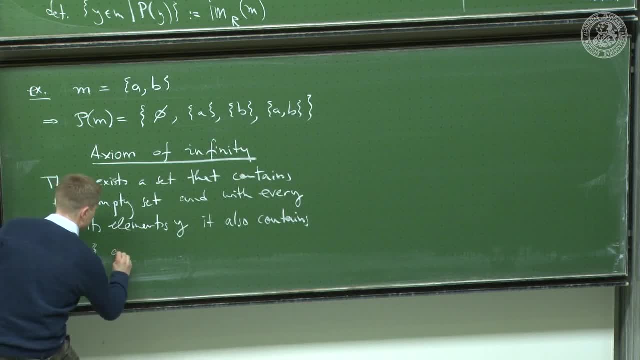 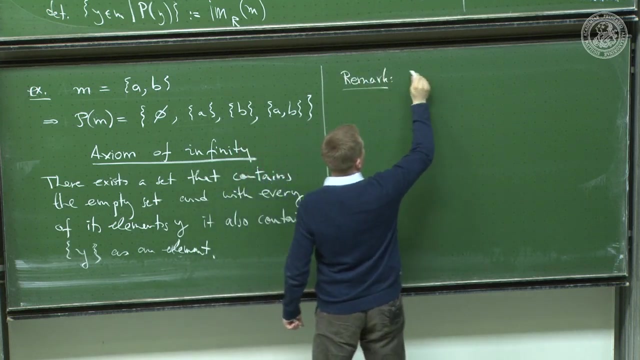 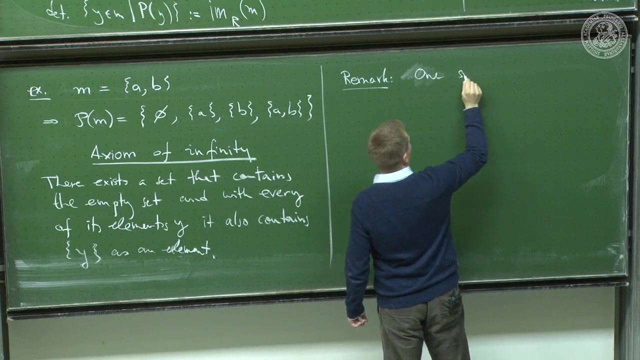 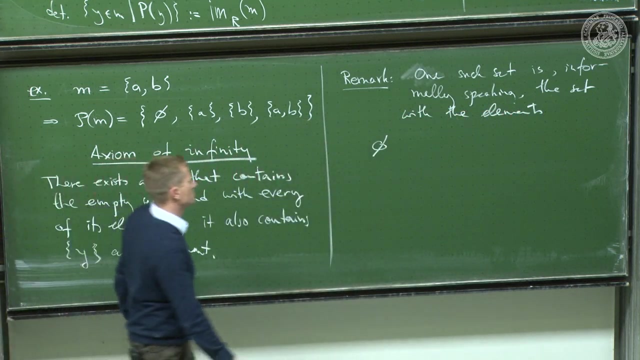 set with the element y as an element. so the smallest, the simplest, one such set. one such set is, informally speaking, a set. the set with the elements empty set. okay, yeah, sure, the empty set got to be in there, but if there's the empty set in it, 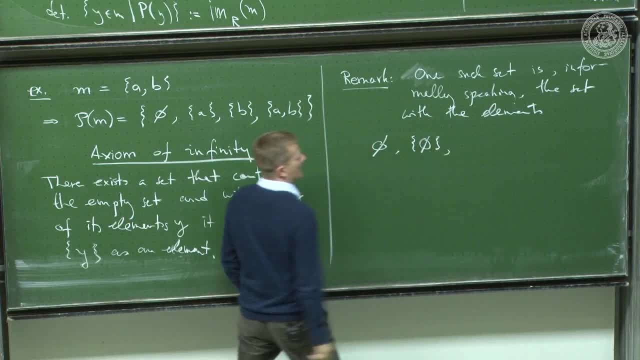 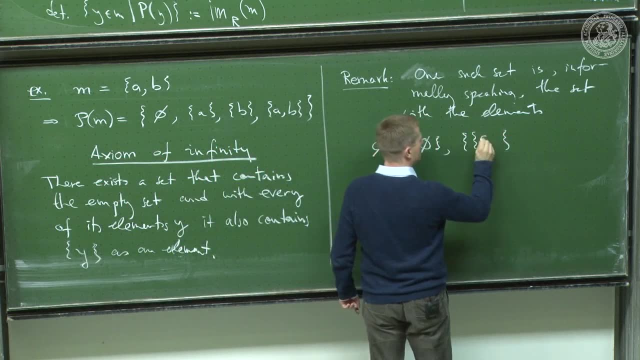 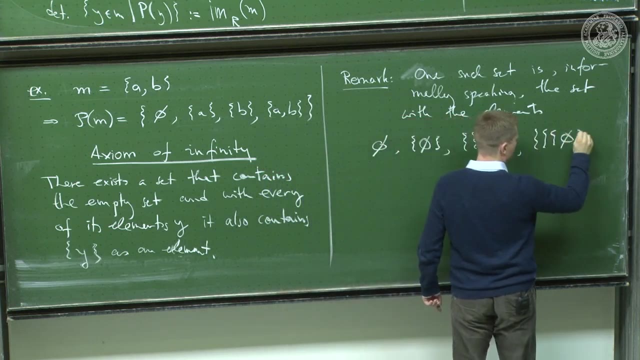 it should also have the set with the element empty set. all right, but if we have that, it should also have the set that contains as an element the set with the element empty set, and then it should have set set, set, empty set, set set, and so on. 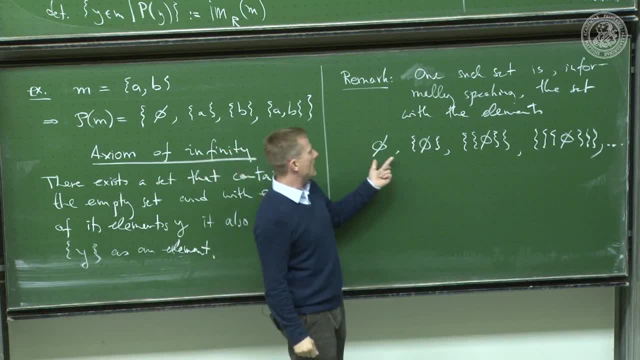 because this can serve as the y for the element y and so on. now in elementary school these are too many brackets. so in elementary school people introduce trivial notation for this and they simply forget the slash here and they say this thing: we make a funny symbol like that: 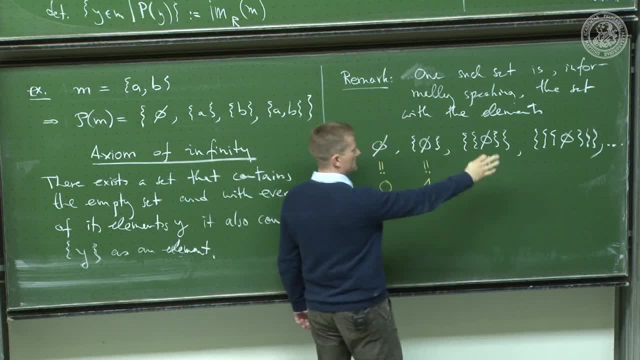 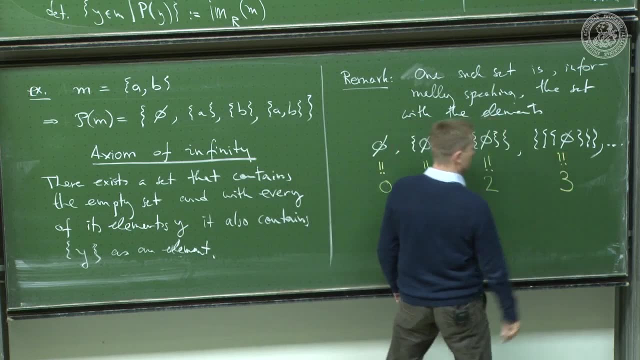 and for this set. these are all sets right. for this set we have a funny symbol that looks like that. for the next set we write yet another one like that, and I think you know what the next funny symbol is. so we invent trivial names for these sets. 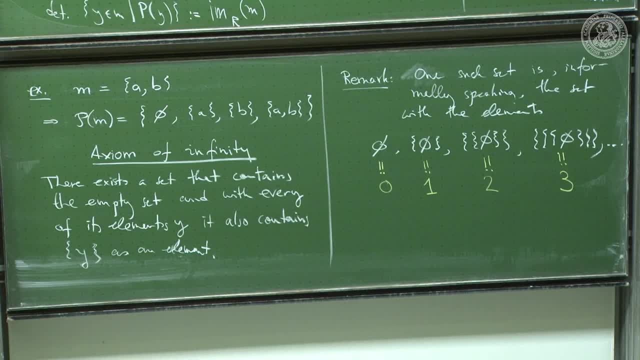 there are other sets that you, whose existence is guaranteed by the axiom of infinity, but this is one particular of those sets. so, corollary, the set of non-negative integers is a set, and it's a set according to axiomatic set theory. if we didn't 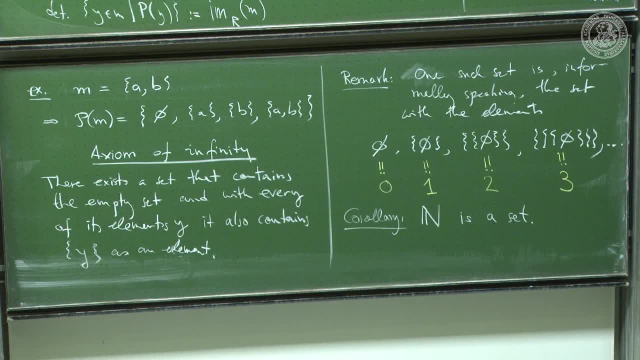 have the axiom of infinity? you still could. you simply could not prove that the natural numbers or the non-negative integers constitute a set, so you need this axiom to get this thing running. now you say again one of these maybe aesthetically not so appealing axioms. 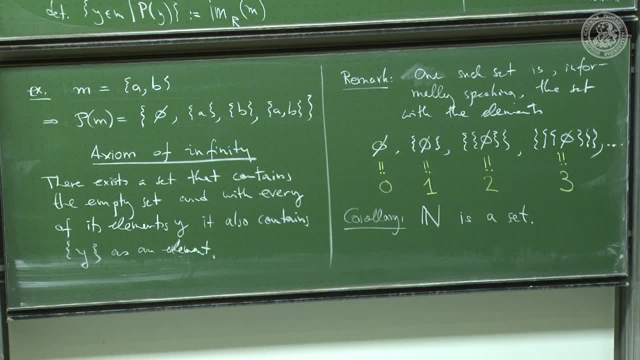 but you can say: ok, what's next? you require that the real numbers always exist. well, remark as a set, not anything further. as a set, the real numbers can be understood as the power set or defined as the power set of the integers, and then you can again. 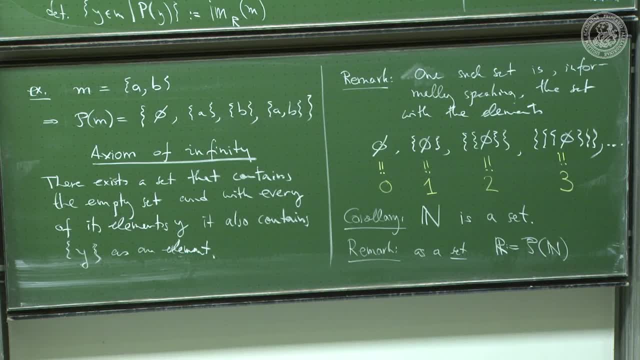 take the power set of the real and you get an even bigger set. and then you can take the power set of the power set of the power set of the integers, and you get a bigger set. and this way you go through the entire universe, the universe of sets. 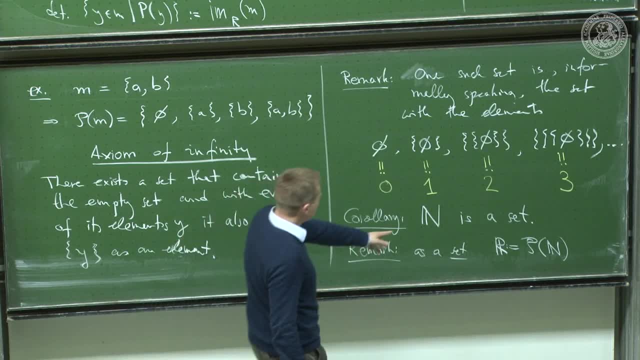 if you wish. but what is this n? this n has just been built from the empty set, and So, up to this point, the only set whose existence we explicitly demanded was the empty set, and we already arrived at the reals. So you see, these are sometimes maybe ad hoc seeming postulates. 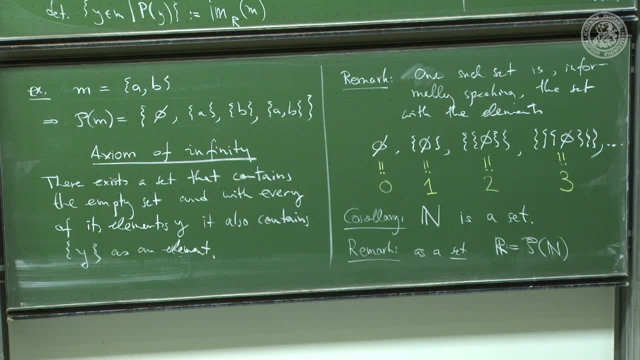 and we haven't gotten all of them. We still need the C and the F, and the C is a special one. You could put it there. You can leave it out. It's the axiom of choice. You can have Zermelo-Fraenkel set theory with or without the axiom of choice. 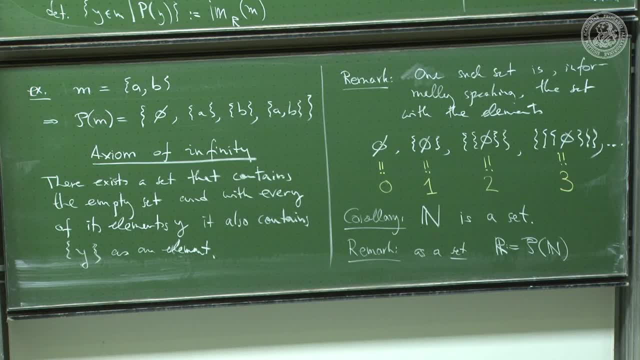 And the F, the axiom of foundation, says you could also have the idea that instead of building sets from the empty set, you could have a bootstrap that you set. Say, you take a set that contains itself or contains the set, and so on and so on. 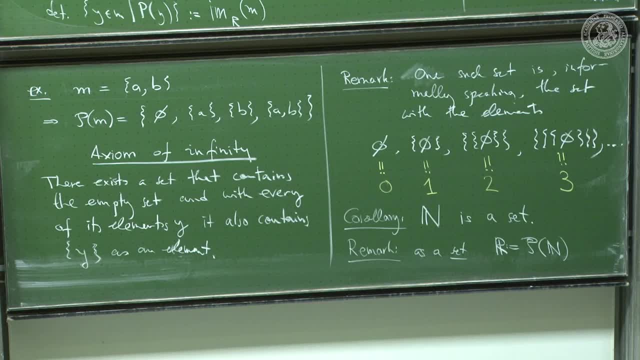 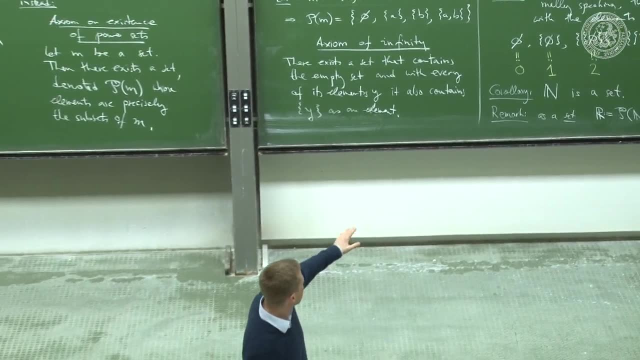 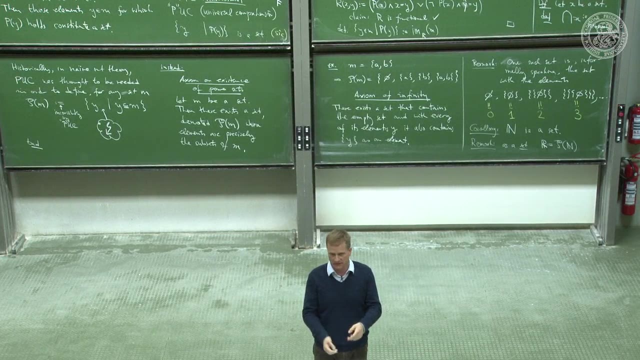 and the axiom of foundation we're going to introduce together with the axiom of choice next time tells you no such thing can be done And in total it will turn out, once all the axioms are there, that essentially every set we will ever consider in standard mathematics. 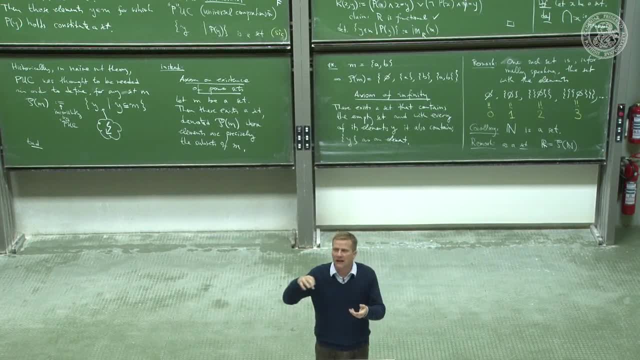 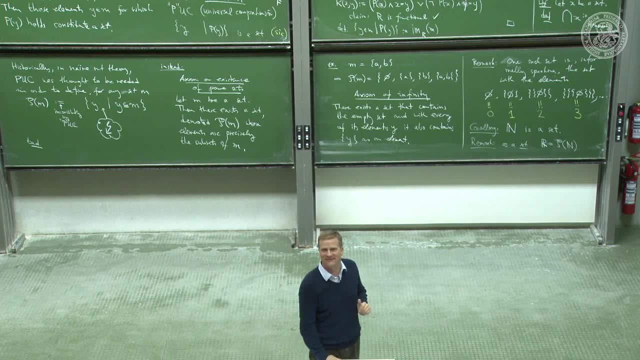 at least in the mathematics built on these axioms will be ultimately basically constructed only from the empty set by these construction axioms we wrote down. So set theory is very simple, It's just the empty set. We continue next time, Thank you. 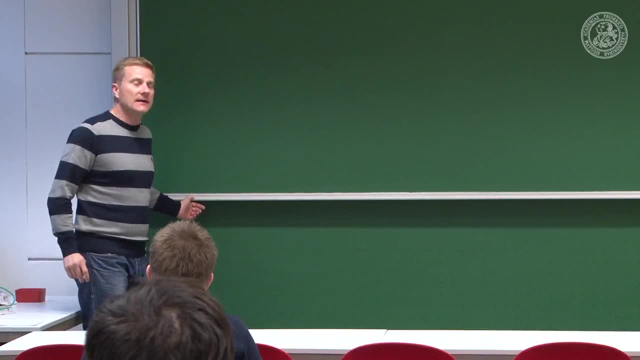 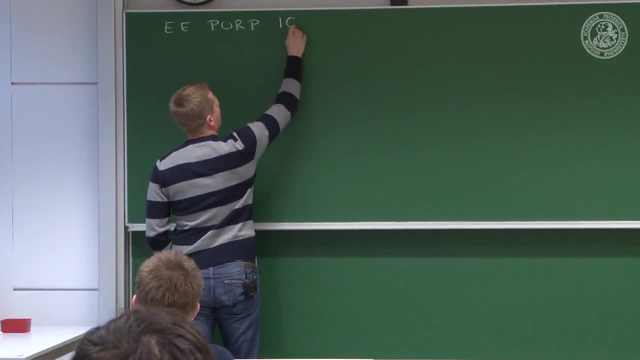 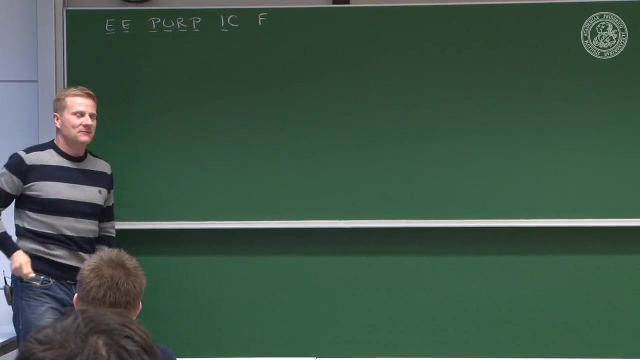 So welcome back to the lectures. In our discussion of the nine axioms of set theory, which were E, E, perp, IC and F, we already discussed the first seven, so that means two to go, And the next one is the axiom of choice. 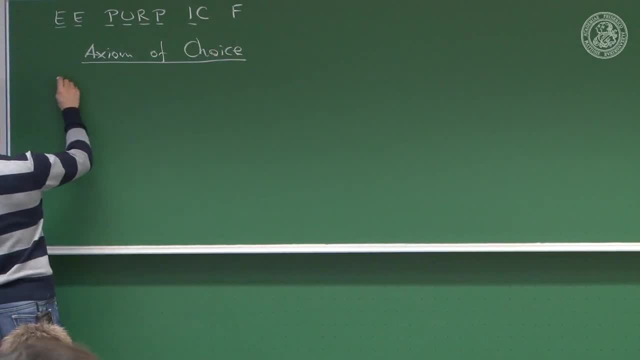 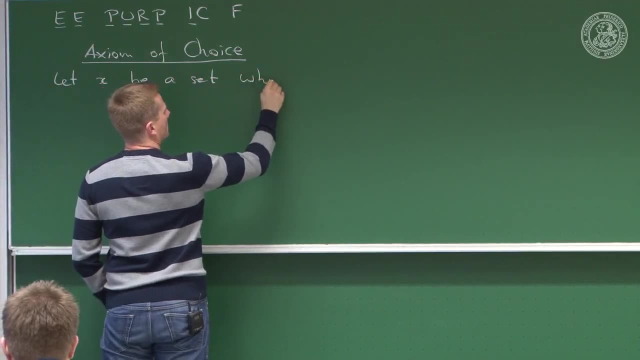 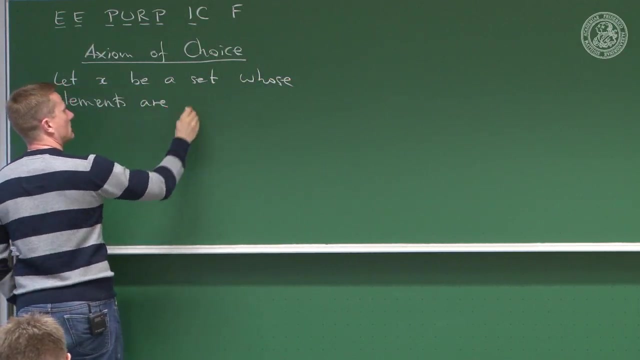 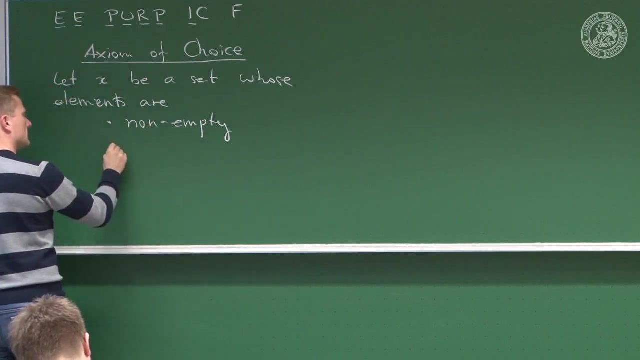 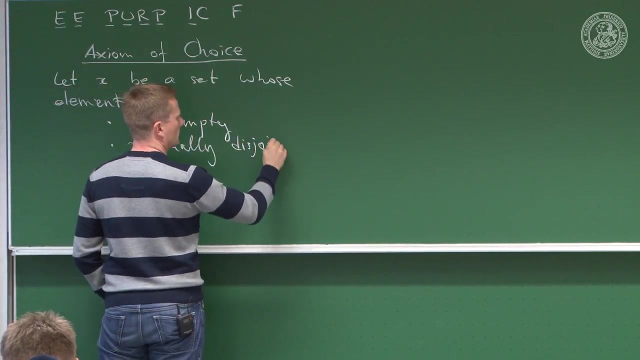 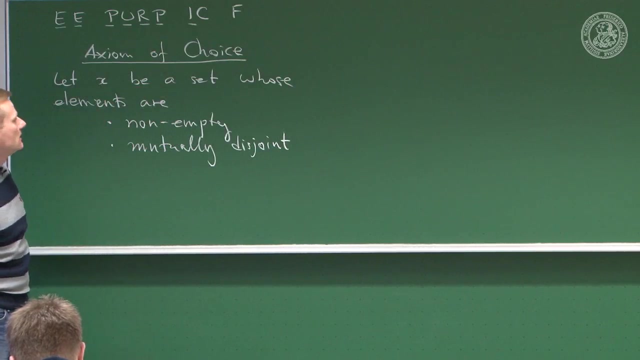 So the axiom of choice talks about a set. Let X, X be a set whose elements are. now there are two conditions: non-empty and mutually disjoint. And that means if you take the intersection of any two elements of the set X, then this intersection will be the empty set. 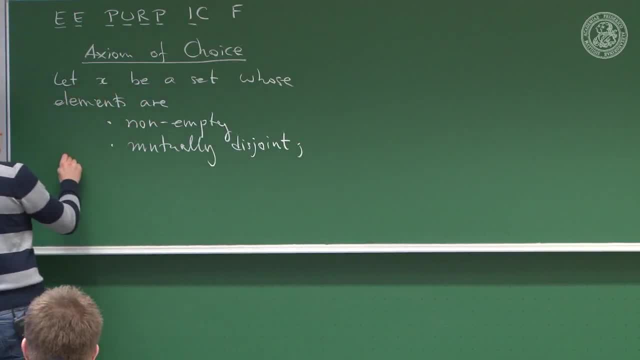 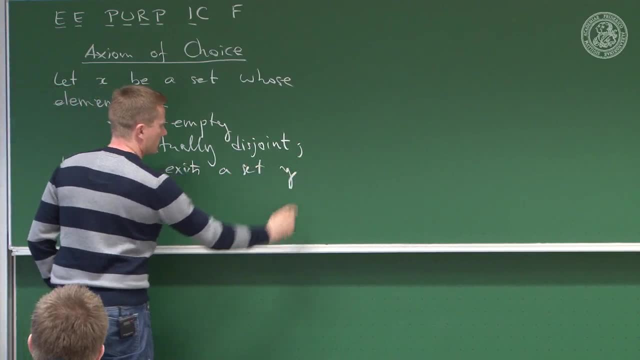 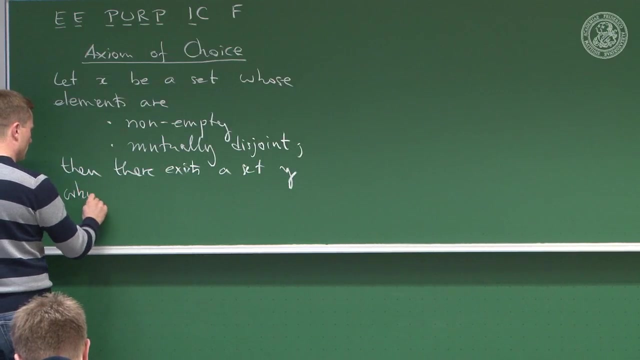 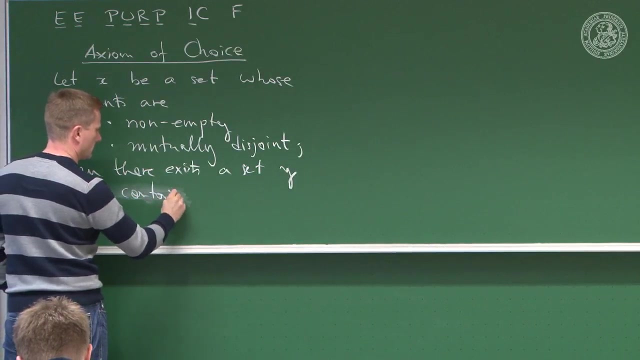 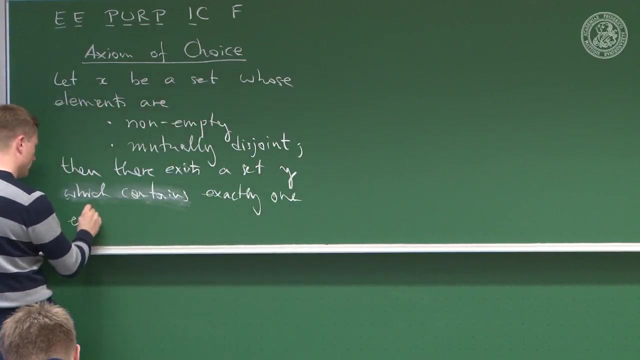 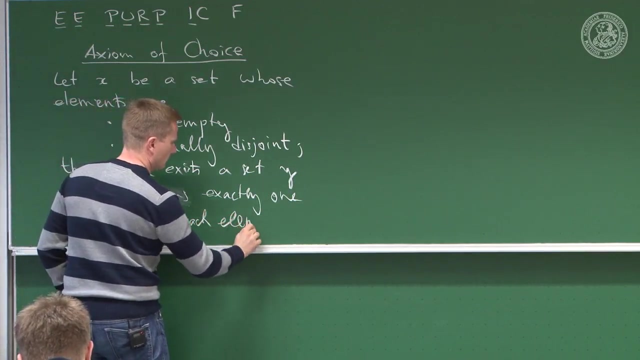 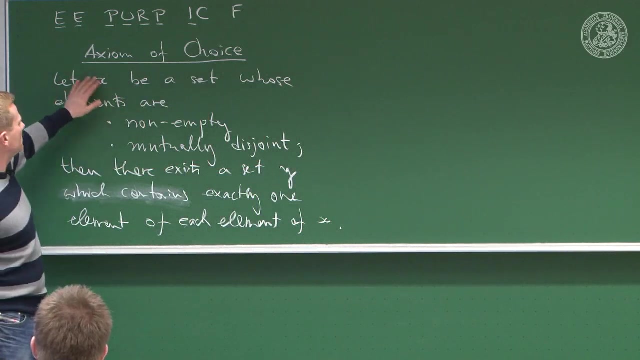 A mutually disjoint. then there exists a set- let's call it Y, whose elements, which contains exactly one element of each element of X. So, intuitively speaking, you look at the elements of X, which are all sets. what else? 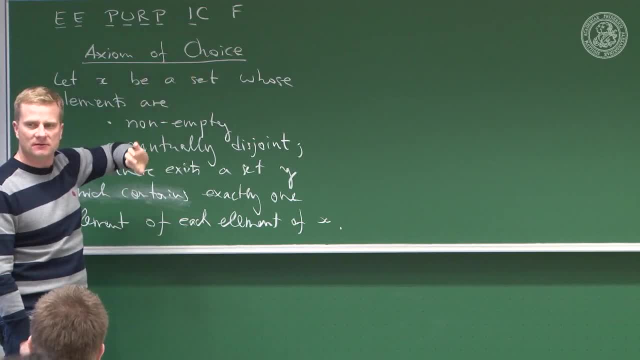 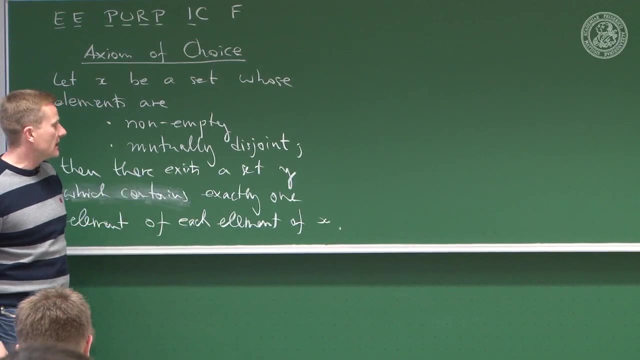 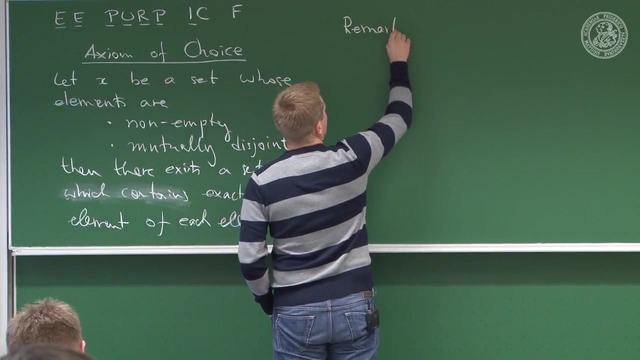 And from each of these sets you pick one element And you collect them all into the set Y, And all the axiom of choice guarantees you that there exists such a set that contains exactly one element of each element of X. Now, an important, well at least maybe somewhat clarifying remark is: 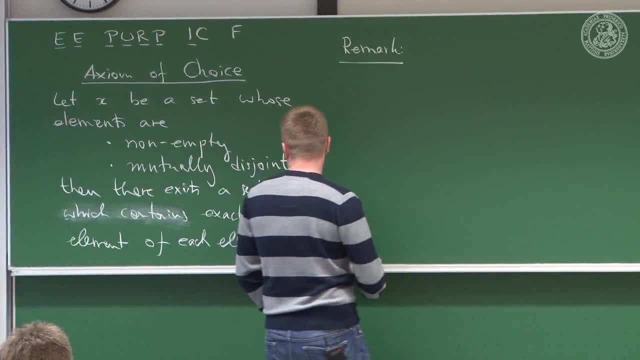 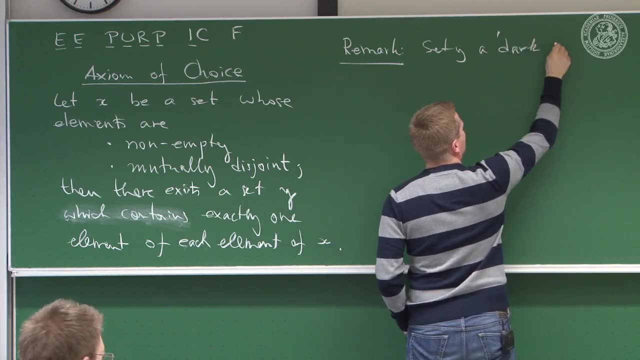 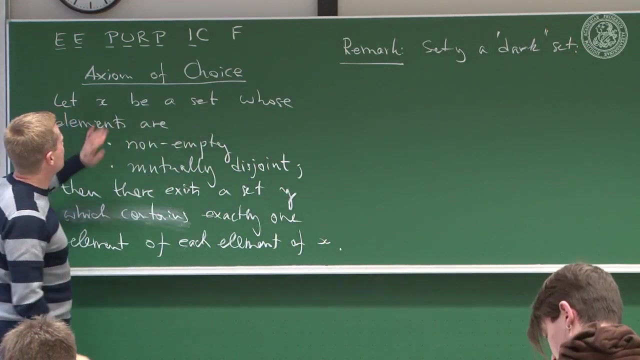 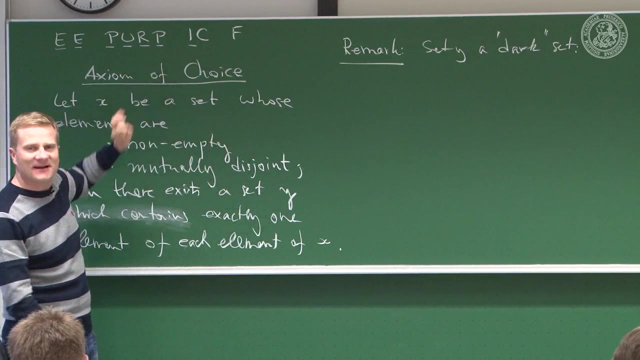 that sometimes people call this set Y a dark set. So what's so dark about it? Well, given any set X, it's not so clear. there's no clear prescription of how you pick an element Of each of the elements of X, right? 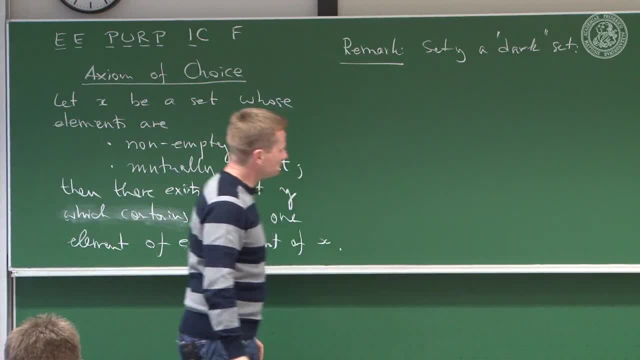 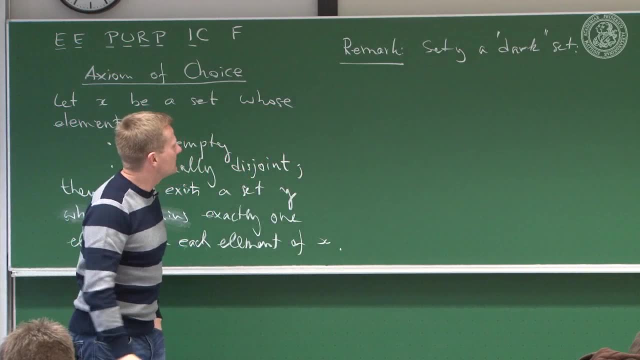 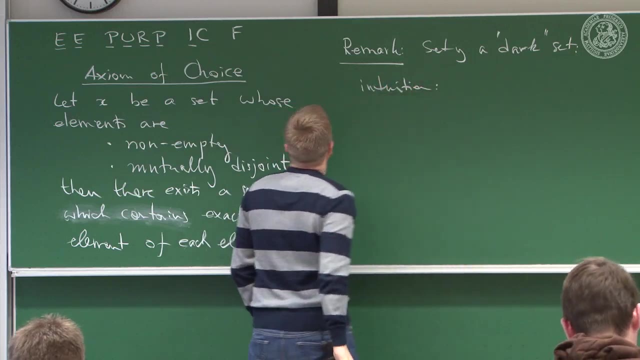 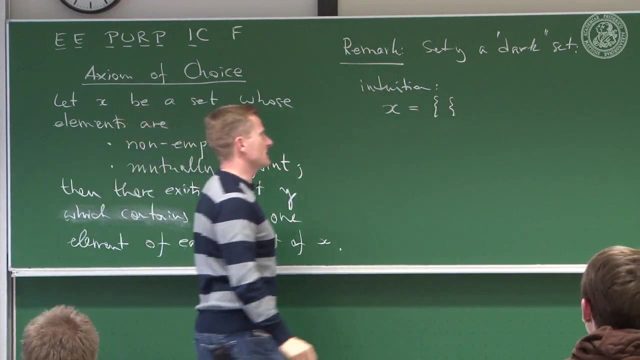 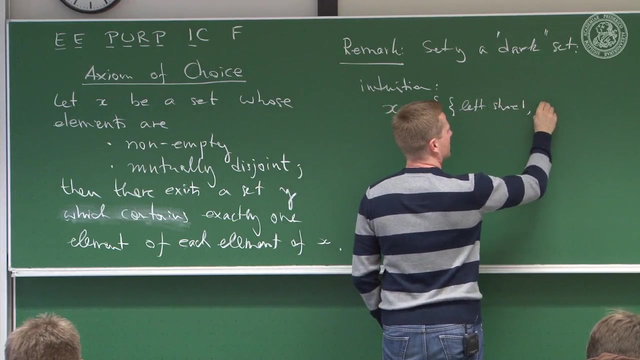 So that's the dark side of it. And so there's this nice- I think it's by Russell- this intuition about it: If your set X consists of sets that consist of pairs, pairs of shoes, okay, So left shoe one, right shoe one. 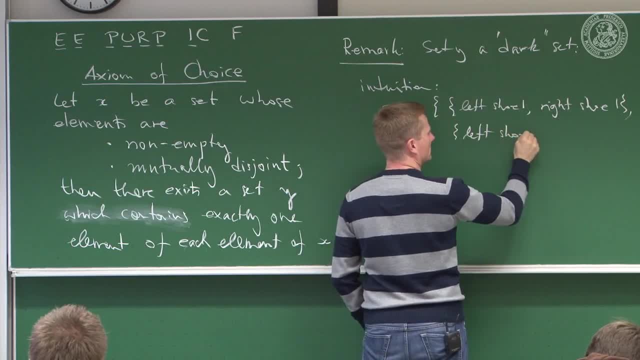 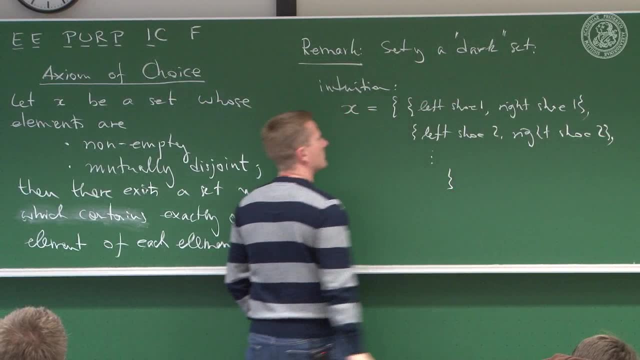 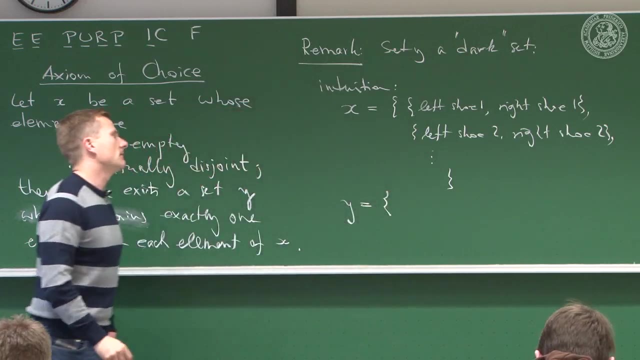 comma, left shoe two, right shoe two and so on, Then in principle you can of course apply the axiom of choice. but you don't need to. If you look at the individual elements here, you can have an algorithm. 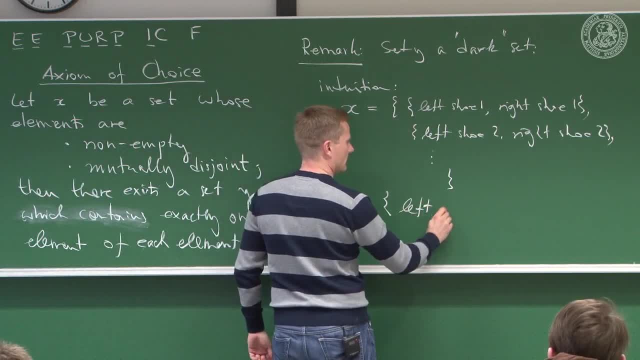 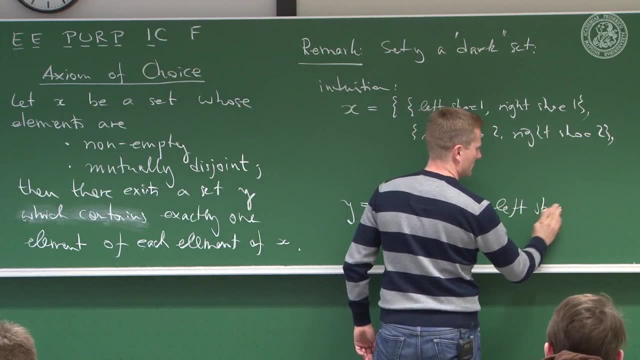 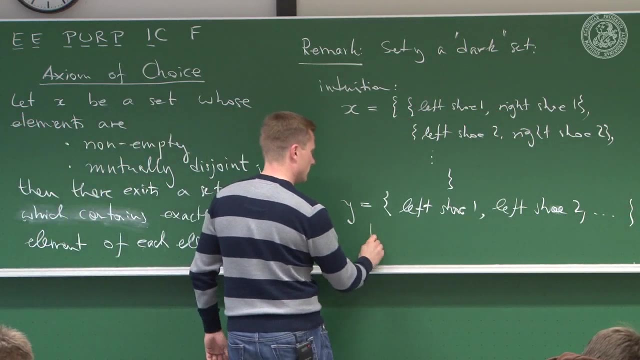 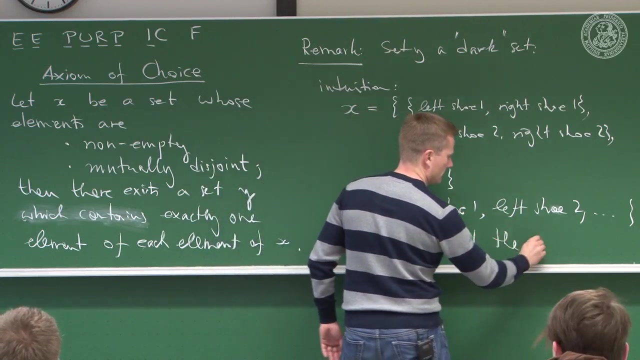 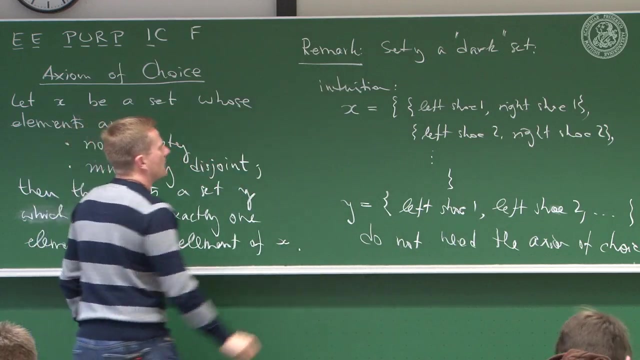 You say: always pick the left shoe So you can build the set- left shoe one, left shoe two, and so on. And to do this you do not need the axiom of choice. But if, instead, you were to consider a set of socks? 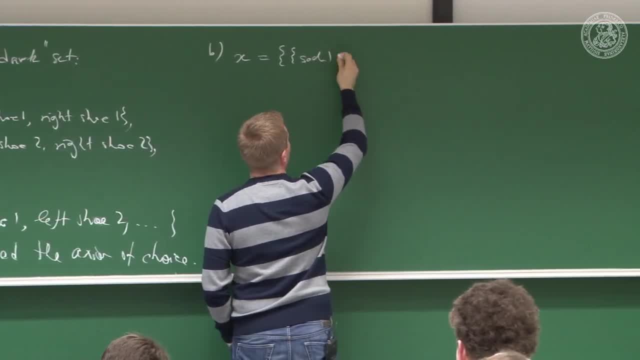 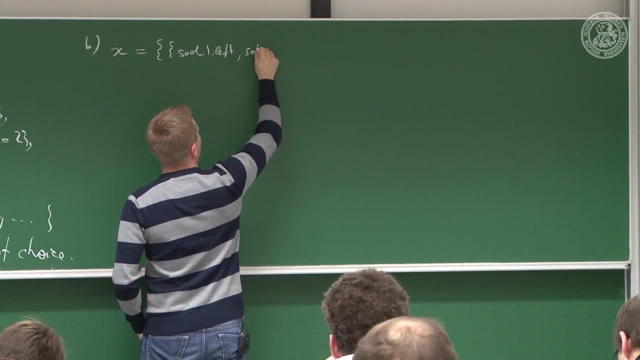 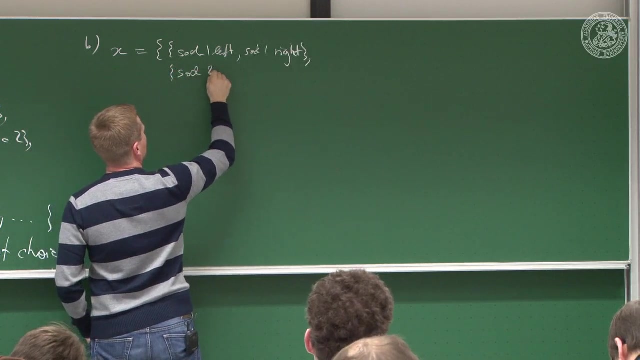 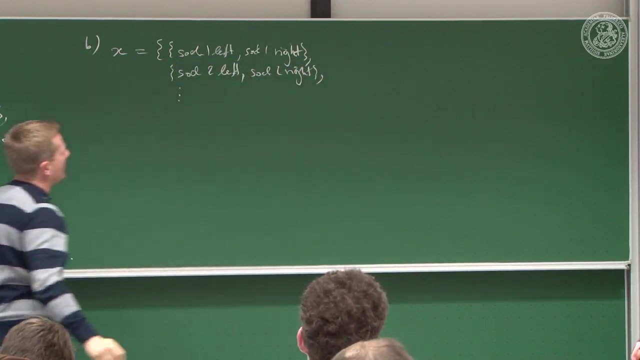 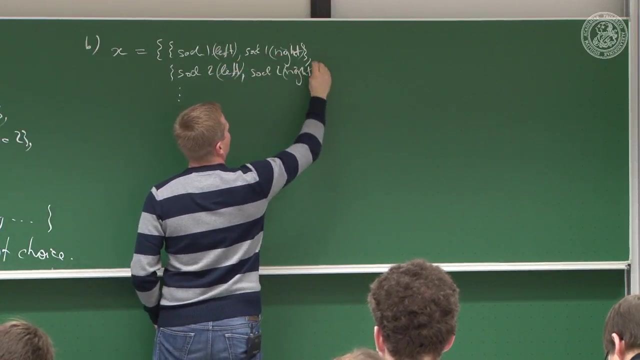 sock one. well, sock one left sock, one right sock, two left sock, two left sock, two left sock, two right, and so on. I introduced this left and right only to say these are two different socks. okay, Different individual socks. 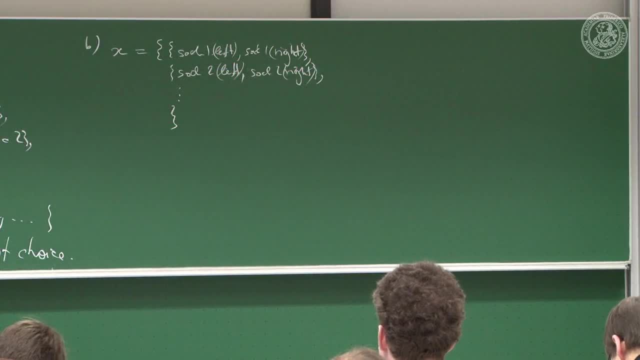 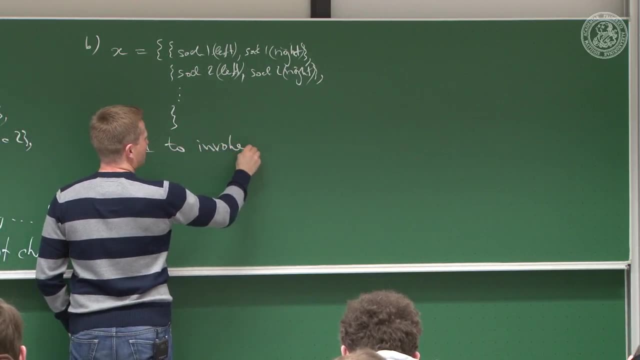 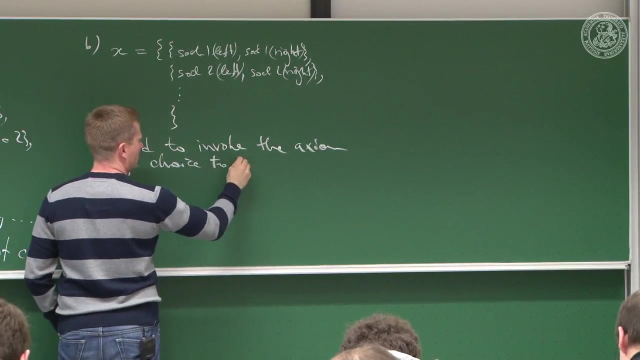 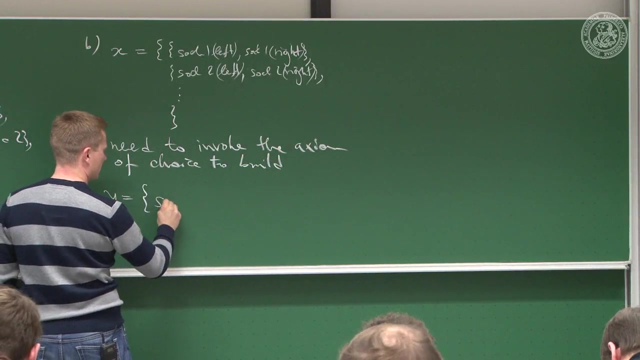 but you cannot distinguish them. So you have two socks. they look the same and in this case you need to invoke the axiom of choice To build the set Y that contains, say, sock one, sock two, and so on. 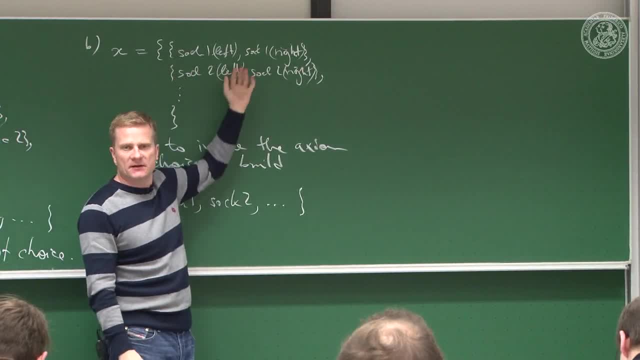 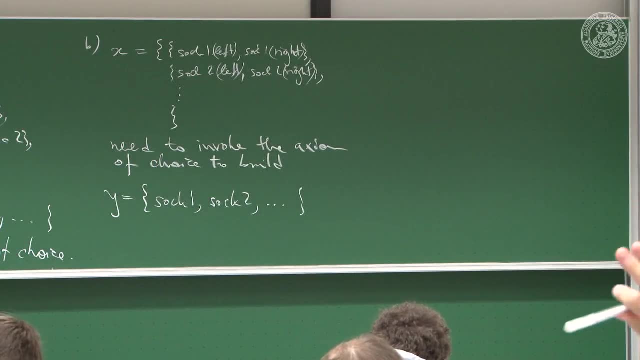 Because you don't really see which one you pick. You have no further means of distinguishing them. Well, it's just an intuition, It's just an analogy. Yes, On the left-hand side, in the last sentence, should it not mean exactly one element? 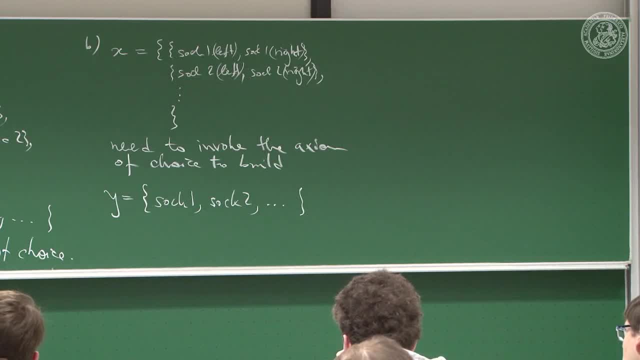 of each set of X. Well, the point is, everything that appears is a set. So, if there's an element of a set, what is an element? Well, we never talk actually about elements, It's just if you want to emphasize. 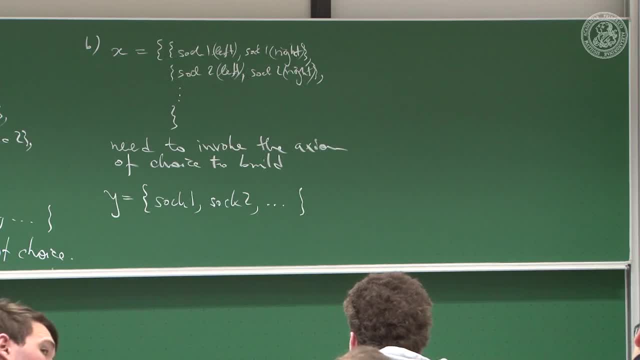 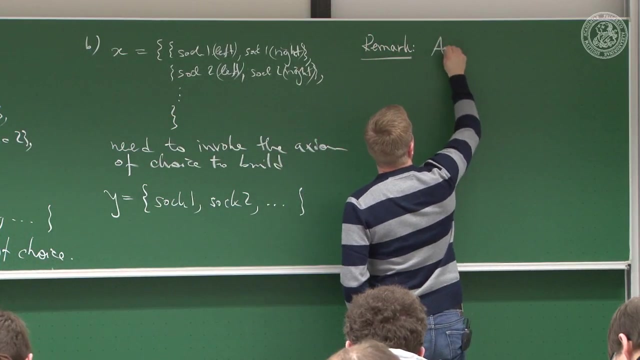 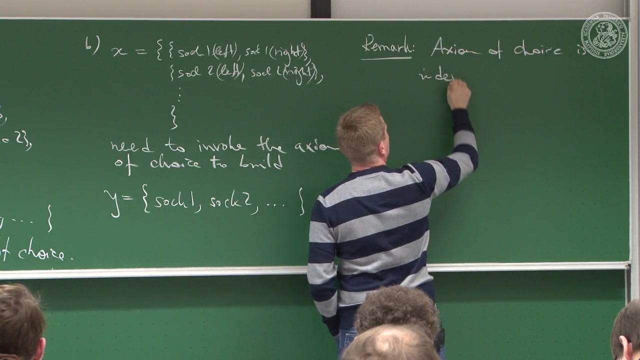 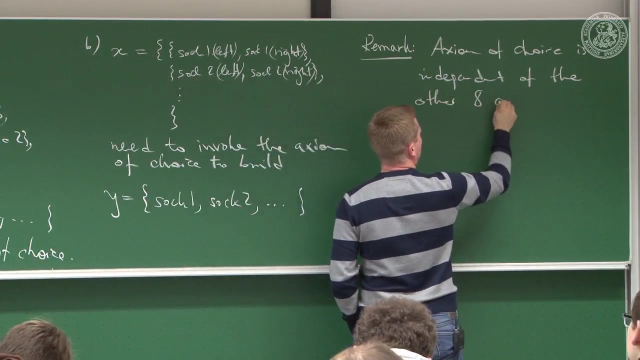 this lies as an element. somewhere we use the word element, But actually elements are also sets. That's the point. Okay, So that's the axiom of choice. Further remark is that the axiom of choice is independent, Independent, Independent of the other eight axioms. 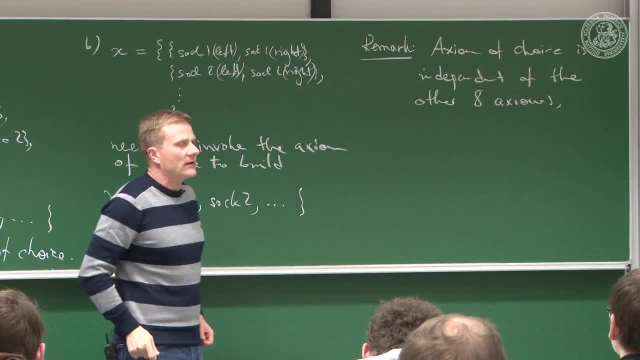 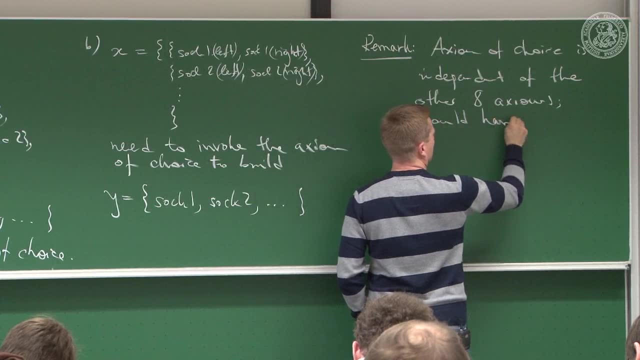 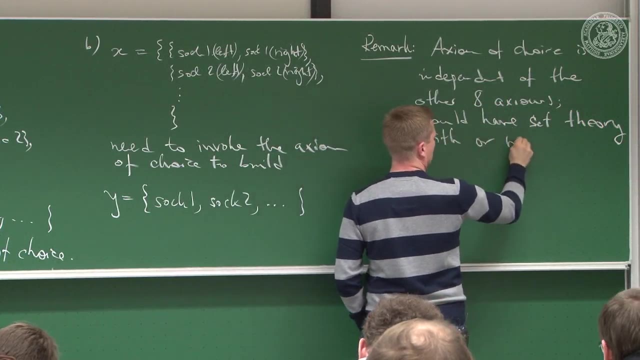 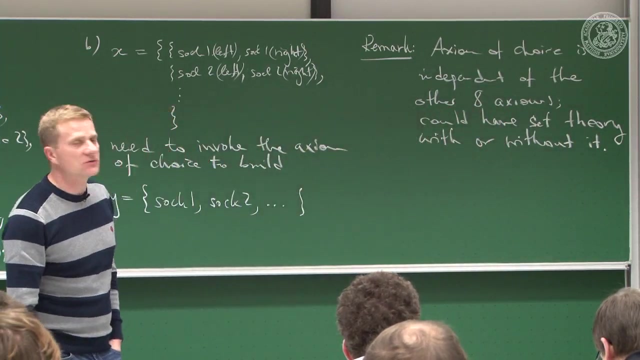 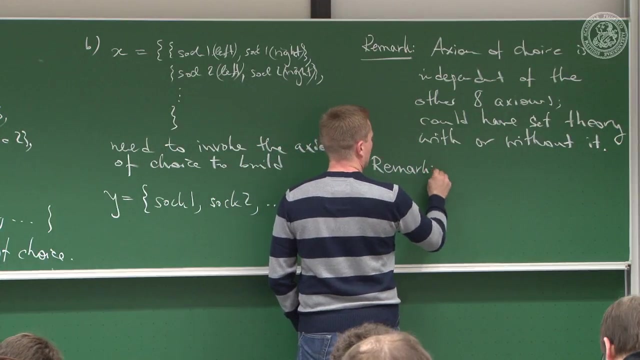 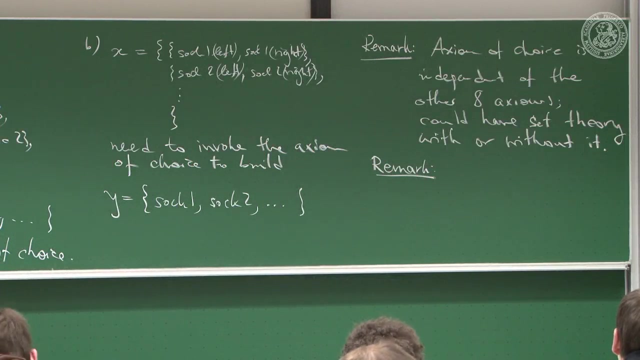 And that means we could have set theory with or without the axiom of choice, But standard mathematics uses the axiom of choice, and so will we. And one last remark is what we actually need it for, And there's a number of uses and a number of theorems. 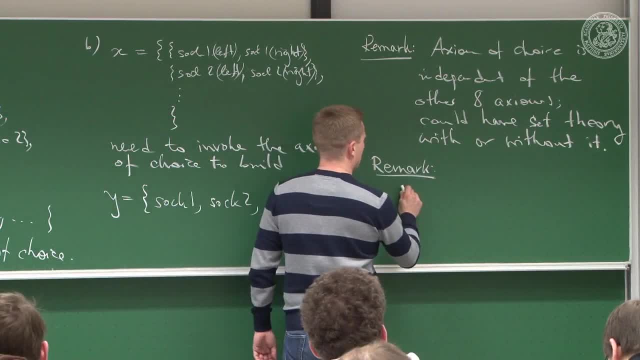 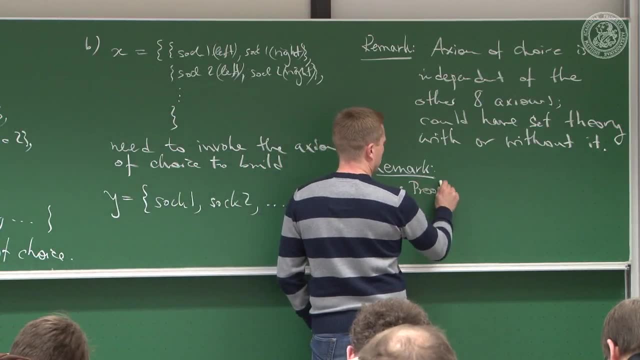 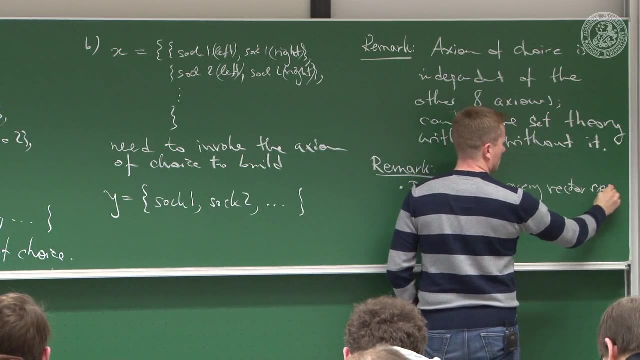 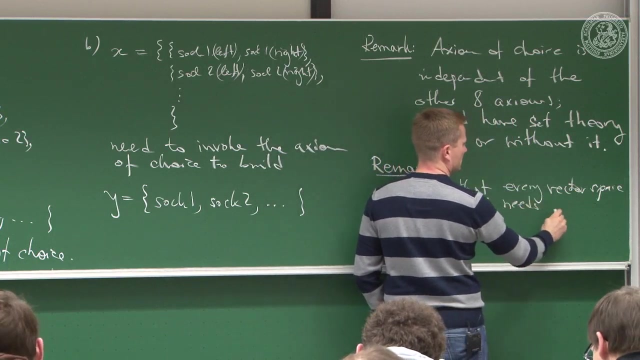 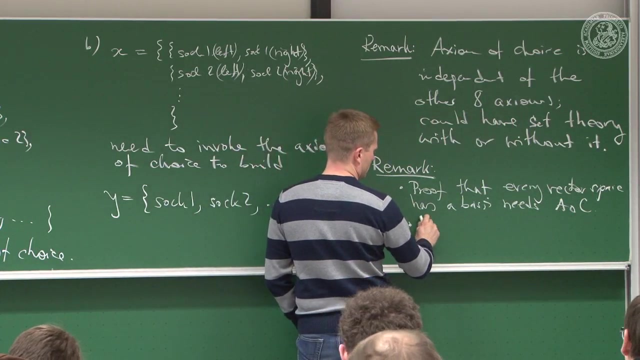 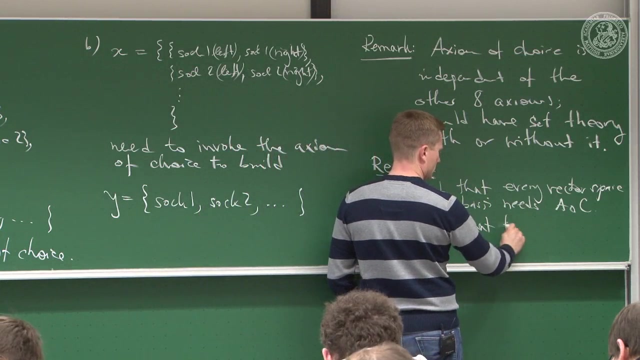 that can only be proven with the axiom of choice. Two that will appear in this course are the proof that every vector space has a basis that needs the axiom of choice, And also the proof that there exists a complete system of representatives built in the axiom of choice. 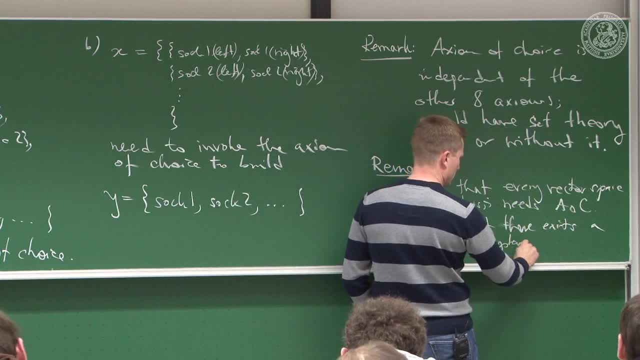 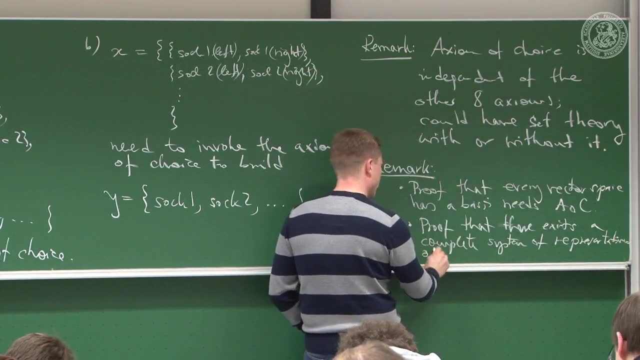 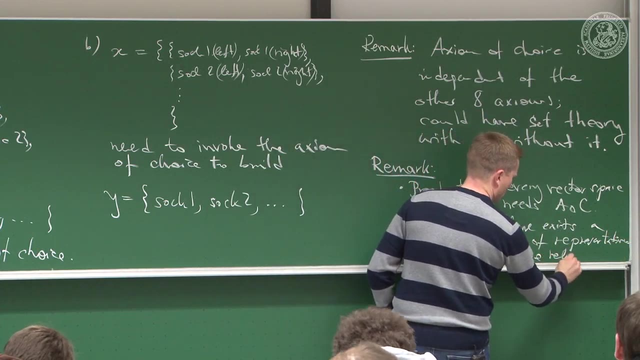 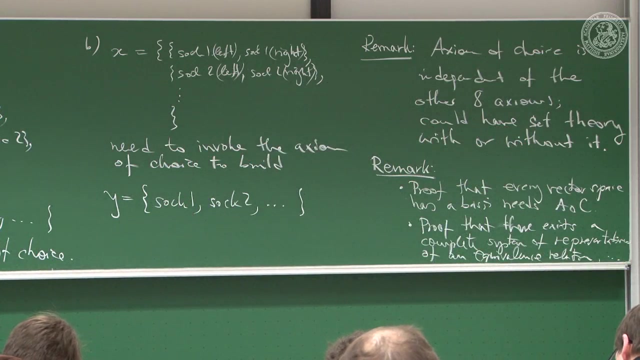 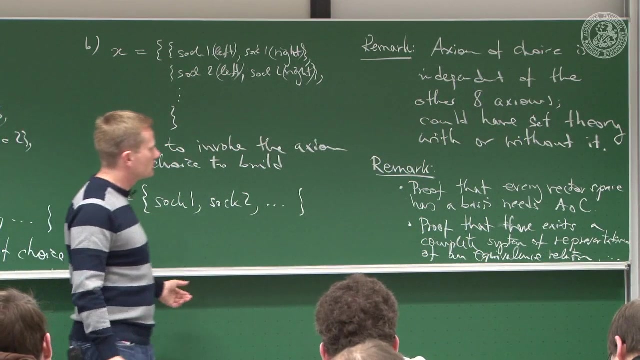 So that's the axiom of choice, And another proof that there exists is the axiom of choice. representatives of an equivalence relation also requires the axiom of choice, And today we'll talk about equivalence relations a little later. Originally, the axiom of choice was, I think, introduced by Zermelo. 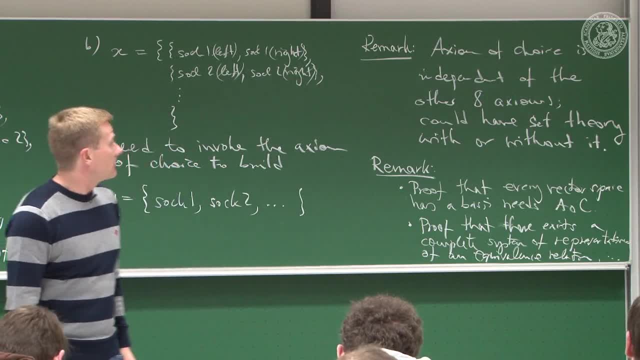 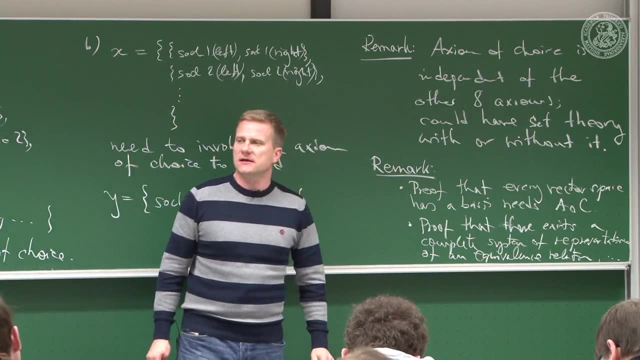 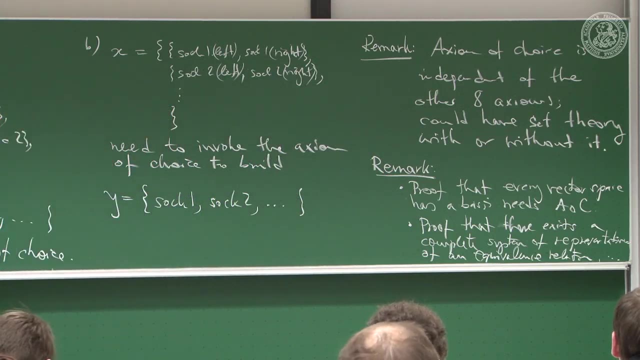 I'm not entirely sure- in proving a theorem that had been unproven for quite a while, And he proved it by introducing this additional assumption. So initially there was some suspicion that this was a meaningful or a very valuable axiom. because there was a suspicion that this was a very valuable axiom. 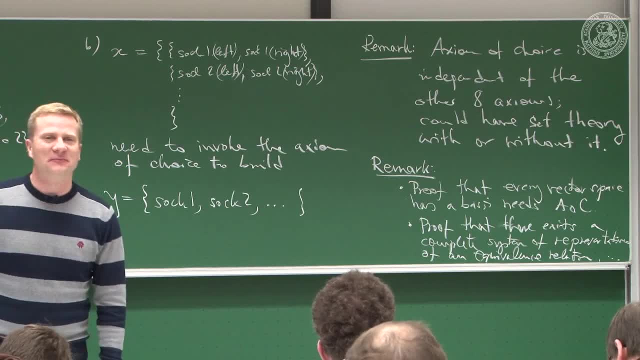 And there was a suspicion that this was a very valuable axiom, And there was a suspicion that it's only been used in order to prove that theorem. So that didn't sound so good, But actually today we like to use this throughout. 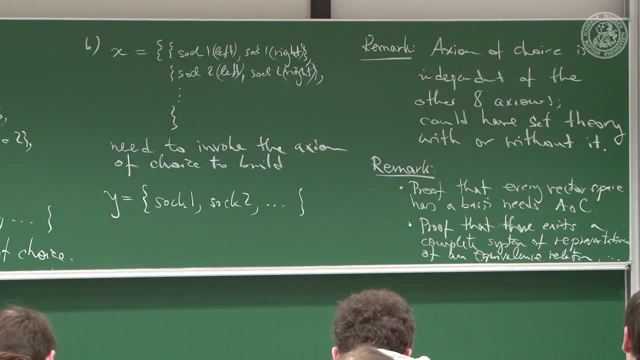 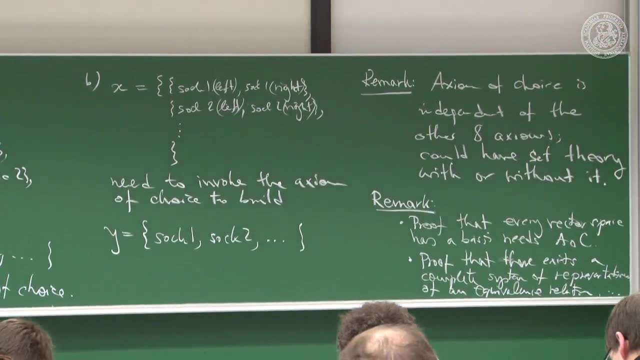 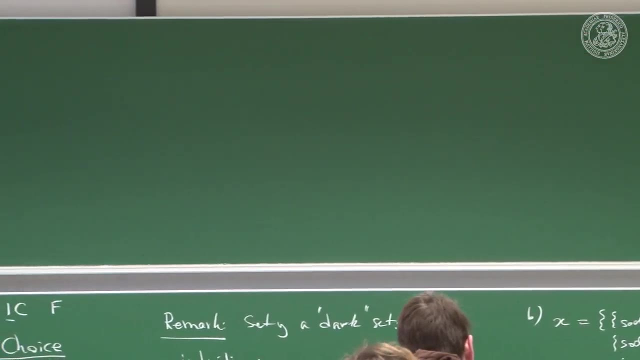 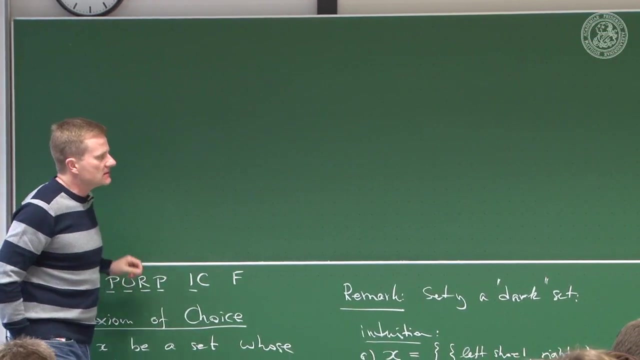 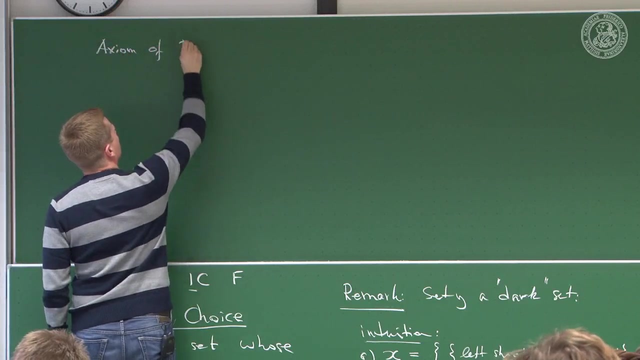 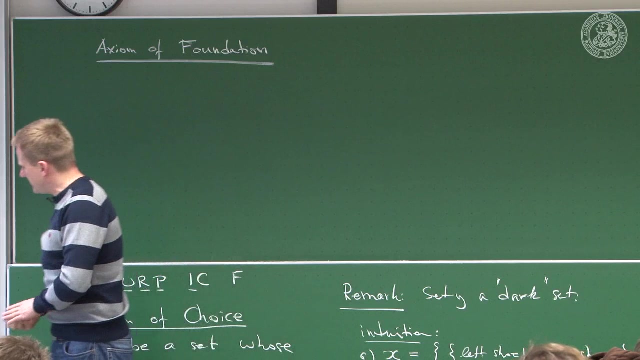 So there is nothing really about the axiom of choice. that's suspicious. So the final axiom is not an existence axiom like some of the others or a construction axiom. It's more like a non-existent existence axiom. That's the axiom of foundation And notwithstanding its name, 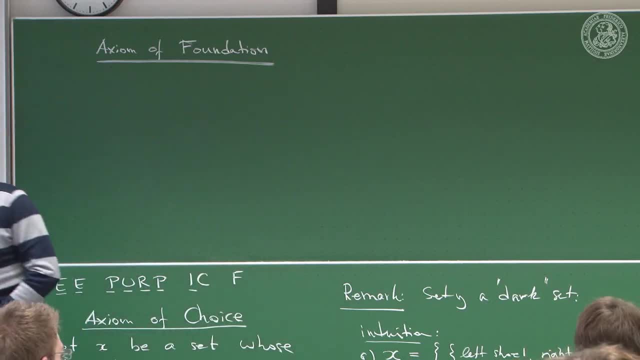 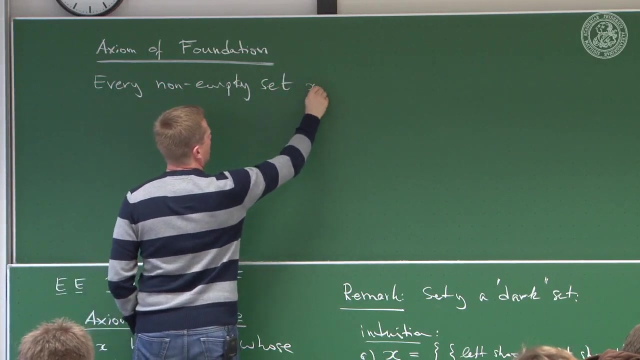 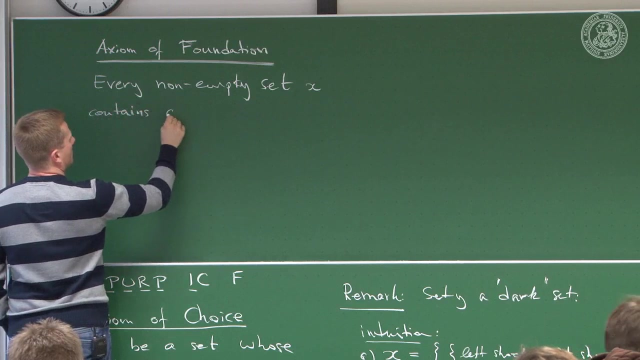 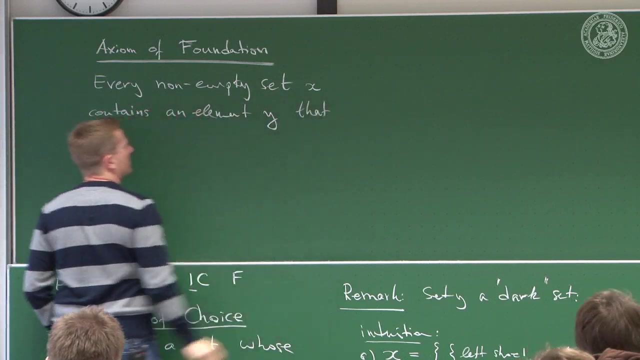 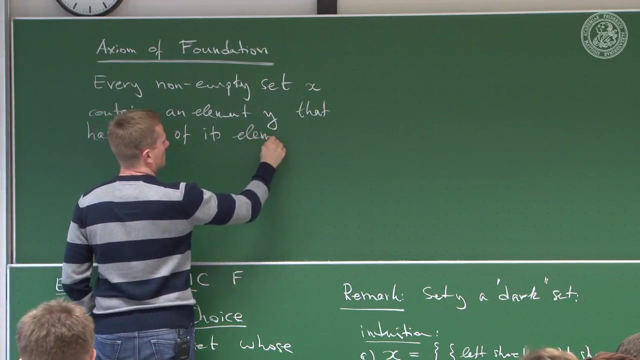 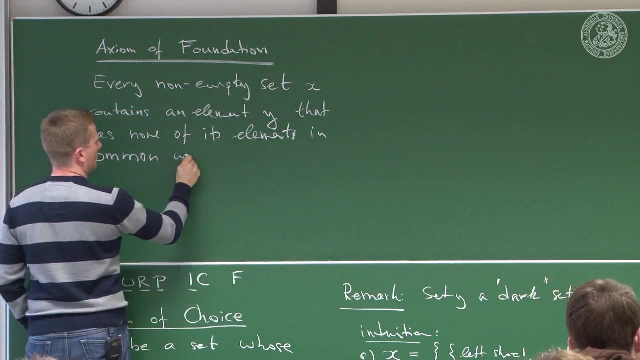 it was one of the axioms that that were introduced last into set theory, And it says that every non-empty set, non-empty set X contains an element Y that has none of its elements in common. that has none of its elements in common with X. 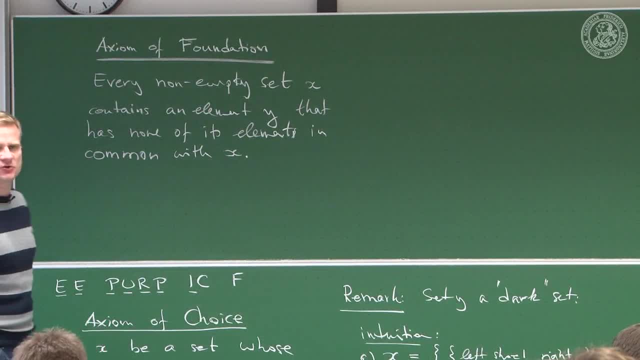 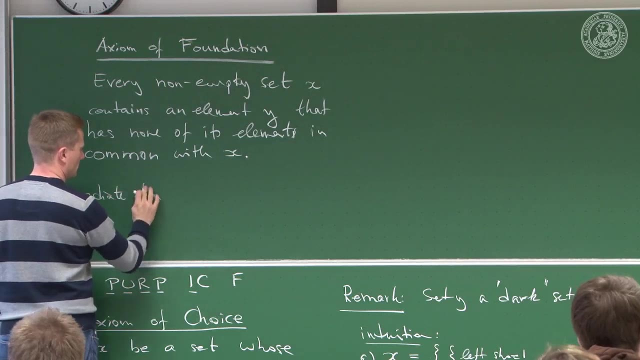 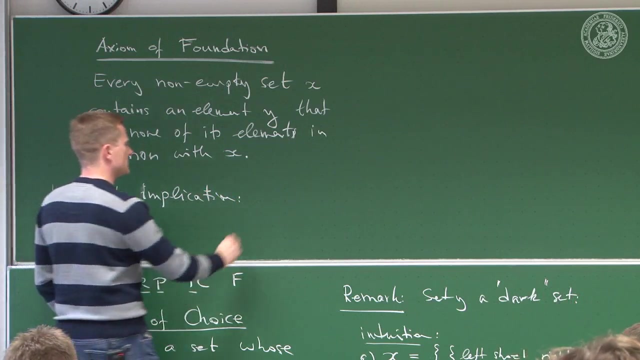 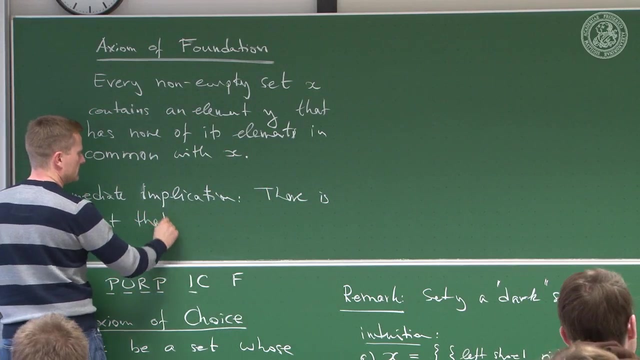 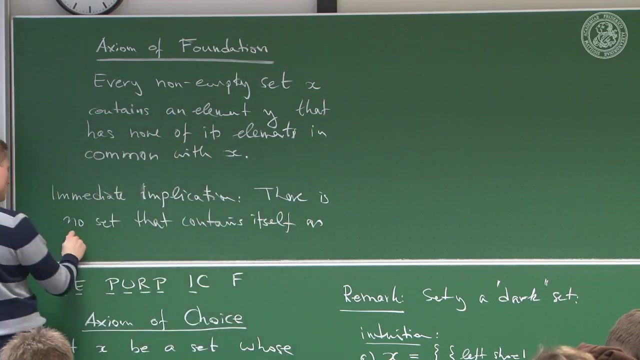 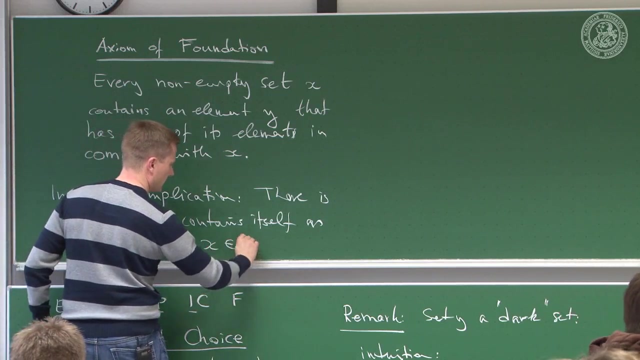 So it's a non-existence axiom, if you wish. It excludes certain situations, So it's an immediate implication that there is no set. There is no set that contains itself as an element, So it's a non-existent X element X. 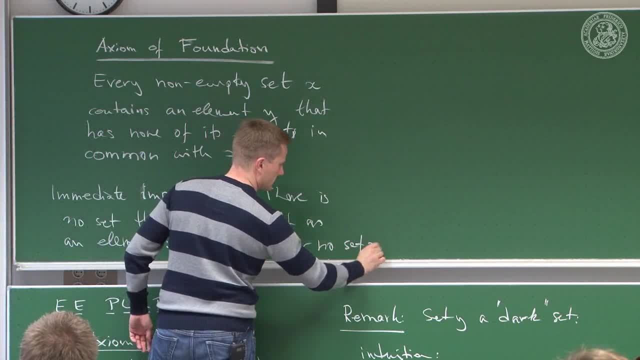 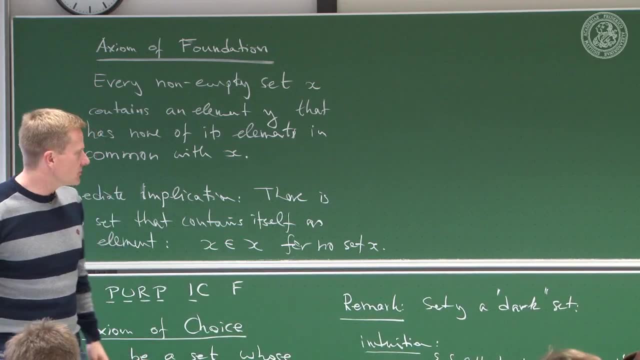 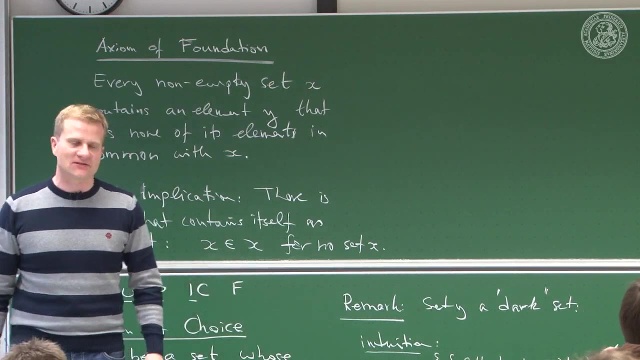 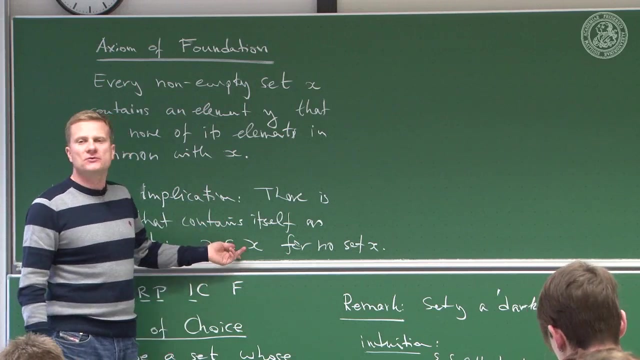 for no set X. OK, So you may remember that when I introduced the element relation, we tried to construct the set of all sets that do not contain themselves. So there was an early attempt to exclude this, but we also showed that trying to build such a set 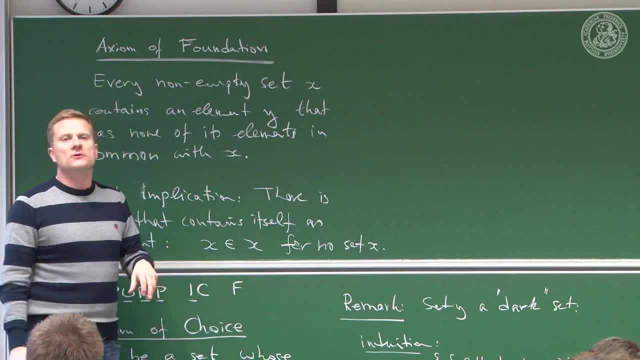 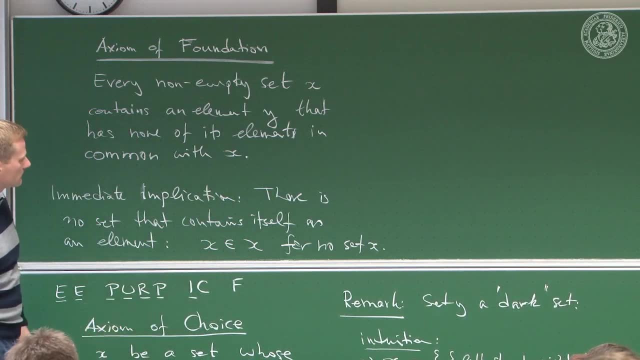 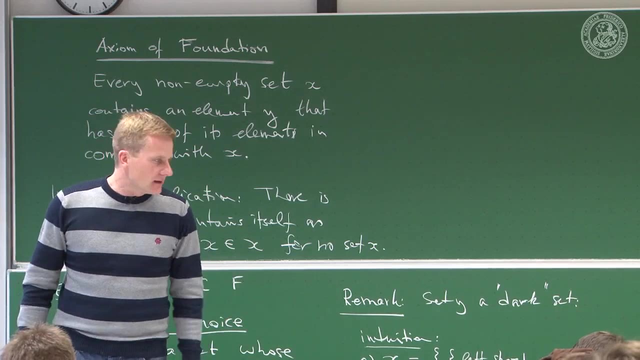 of sets that don't contain themselves, we get something that is a non-set, because it no longer satisfies the first axiom of our system of axioms. well, that we had to give up. we also couldn't include it by a principle, a universal principle of restriction, a universal 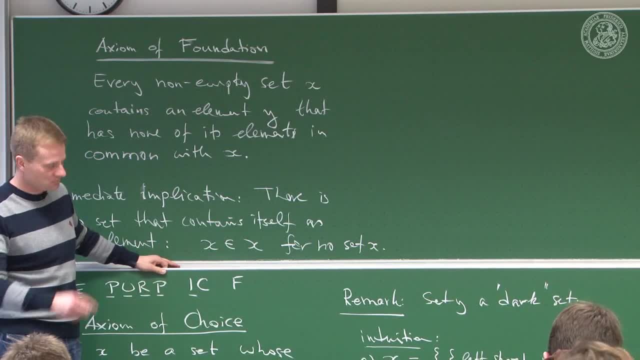 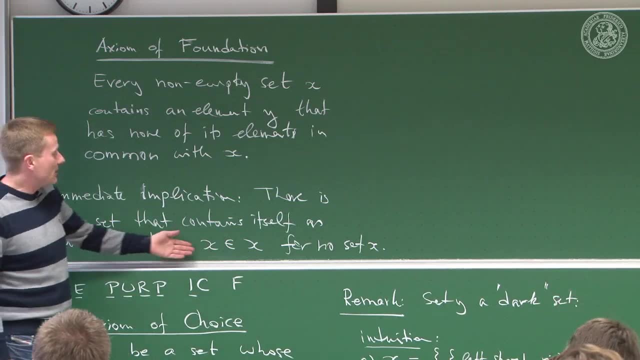 sorry, universal principle of what was it called comprehension. thank you very much, because there is no universal principle of comprehension, there is only a restricted principle of comprehension. so, after all, the axiom of foundation has to take care of that. ok, and so ultimately, I discussed this before the axiom of foundation. 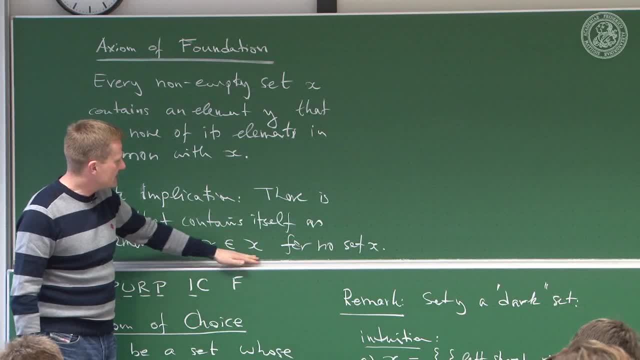 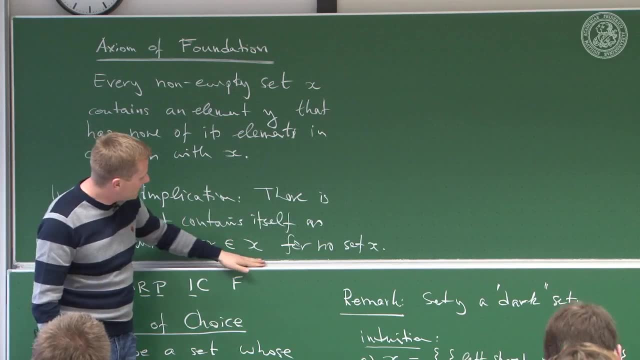 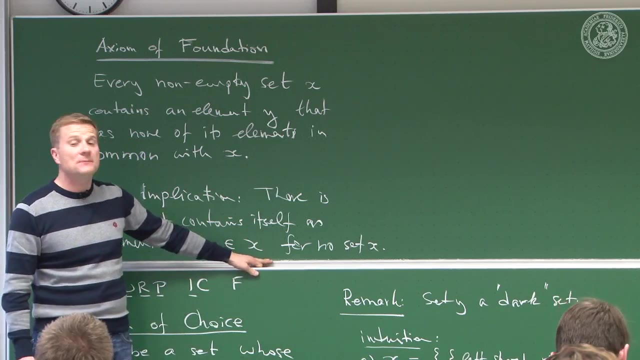 also excludes that you start defining sets in this way. you could say, well, let's take a set that contains itself as an element, as self-referential, and so on. if you don't have this, then ultimately, every set needs to be built of the empty set.